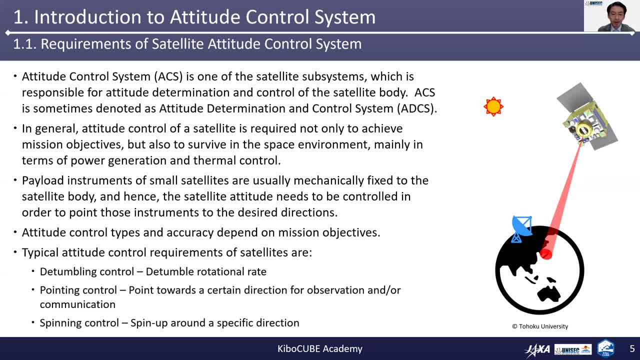 entire satellite. Tailored instruments of small satellites are usually mechanically fixed to the satellite body and hence the satellite attitude itself needs to be controlled in order to point those instruments towards the desired directions. Archer control modes and accuracy depend on each satellite's mission objectives. There are three typical actual control requirements. 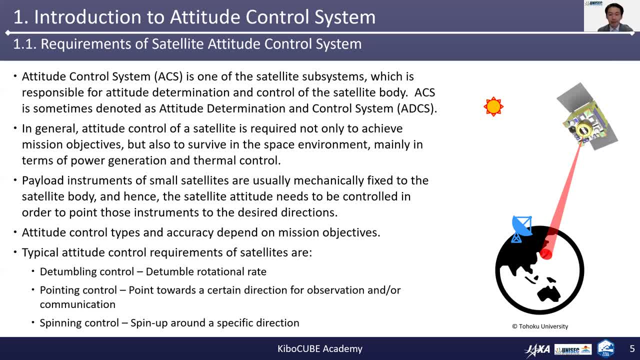 of satellites. The first is the tumbling control, which is to retumble the rotational rate of the satellite body, especially after the separation from the launch vehicle or release from the International Space Station. The second is pointing control, which is to point the spacecraft. 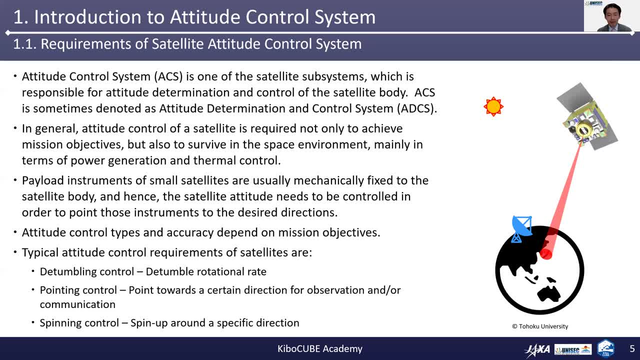 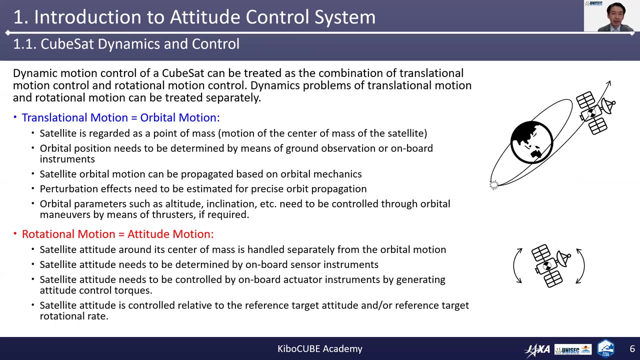 attitude towards a certain direction for observation and or communication purposes with the ground station. And the last is spinning control, where the spin-up is required to achieve a spin stabilization of the satellite. To understand ACS better, let's study the dynamics of CubeSat in space. 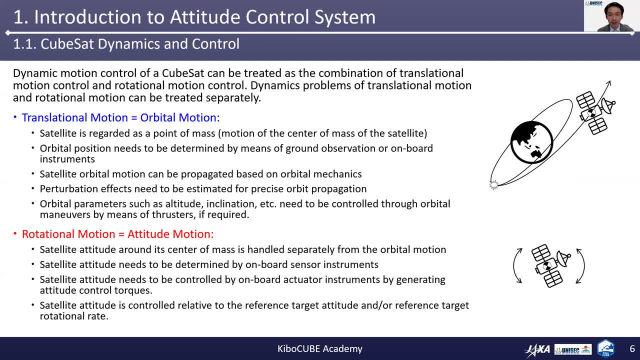 The dynamic motion control of a CubeSat can be treated as the combination of translational motion control and rotational motion control. Dynamics problems of translational motion and rotational motion can be treated as different from the dynamic motion control of the CubeSat in space, treated separately from the mathematical point of view. 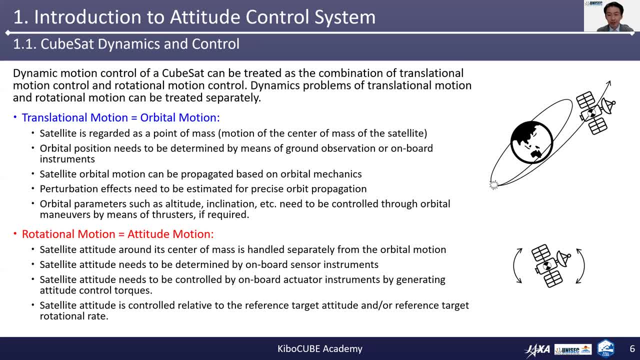 The orbital motion is referred to as a translational motion. as it has these characteristics, Satellite is regarded as a point of mass, which means that the motion of the center of mass of the spacecraft is discussed in the translational motion analysis. The orbital motion needs to be determined. 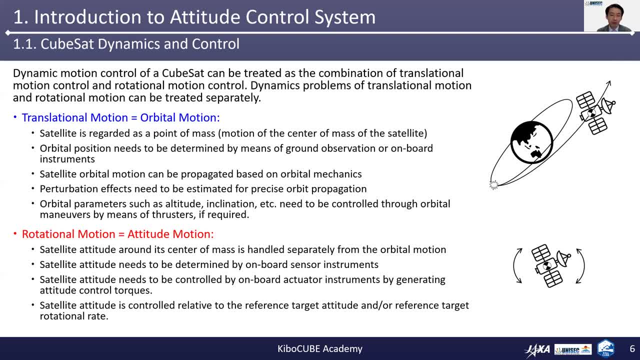 by means of ground observations or onboard instruments, A satellite's orbital motion can be propagated based on orbital mechanics. Perturbation effects acting on satellites need to be estimated for precise orbit propagation And orbital parameters such as altitude, inclination et cetera. 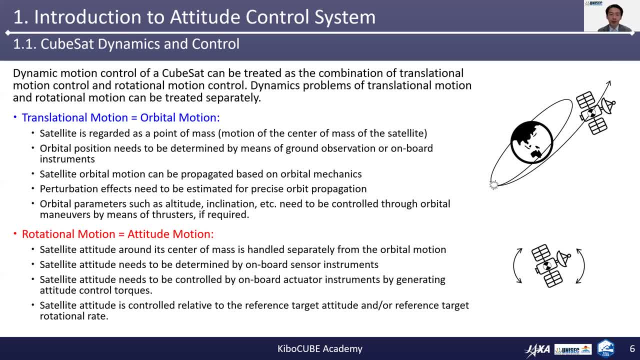 Need to be controlled through orbital maneuvers by means of stresses if required For the rotational motion or the attitude motion analysis. the spacecraft attitude around its center of mass is handled separately from the orbital motion. Satellite attitude need to be determined by onboard sensor instruments. 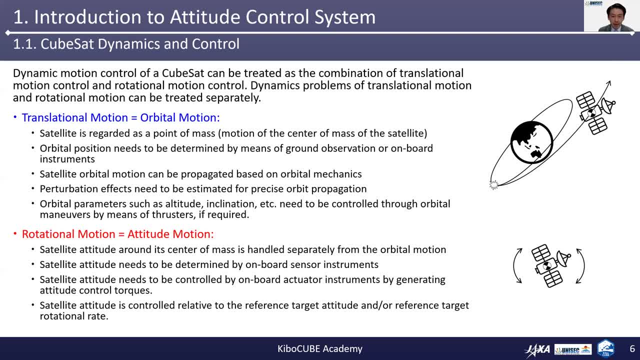 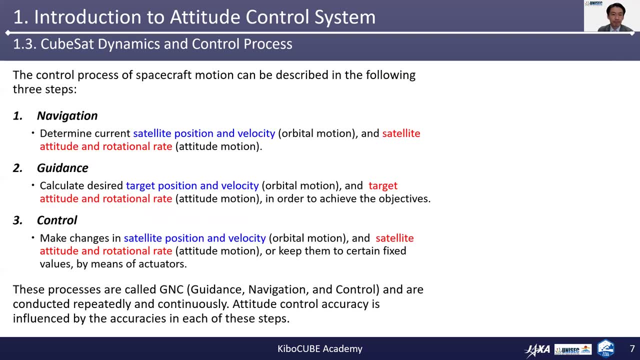 And controlled by onboard actuator instruments by generating actual control torques. Furthermore, the satellite attitude is controlled relative to the target attitude and rotational rate. The control process for motion of a spacecraft can be described in the following three steps: Navigation, guidance and control. 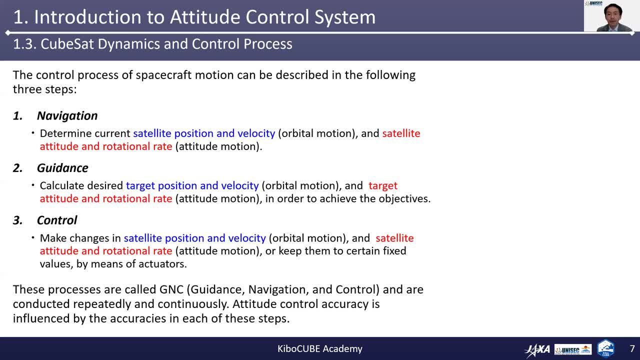 The figure on the right illustrates the analogous situation on Earth. To reach the target place on Earth, you will need navigation in order to know where you are currently located, Then guidance in order to know where to go, And then control, And then control. 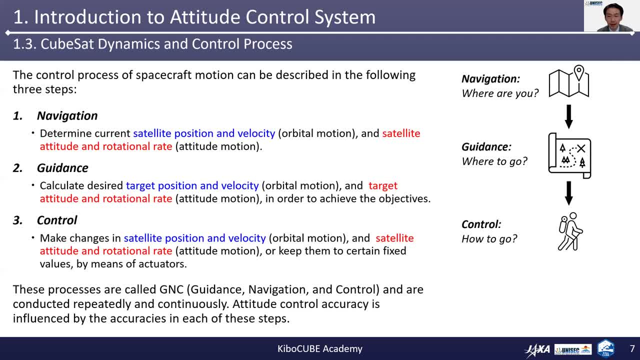 And then you will need navigation in order to know how you proceed along the way to the goal, And you will repeat these steps until you finally arrive at the goal. Satellite control can be understood in a similar way. The first step is navigation. This step is to determine the current position. 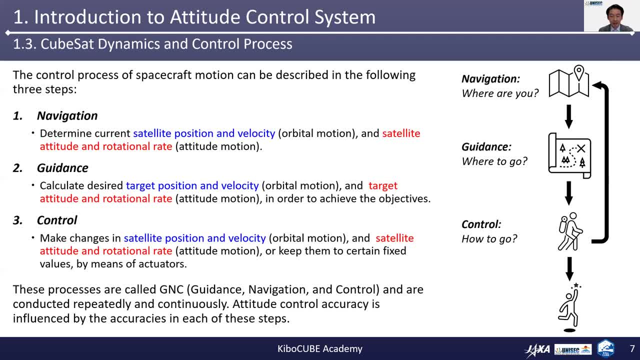 and the velocity of the satellite for the orbital motion analysis analysis, as well as the satellite attitude and rotational rate for the attitude motion analysis. This is also illustrated in the right figure. The second step is the guidance, which is to calculate the desired target position and 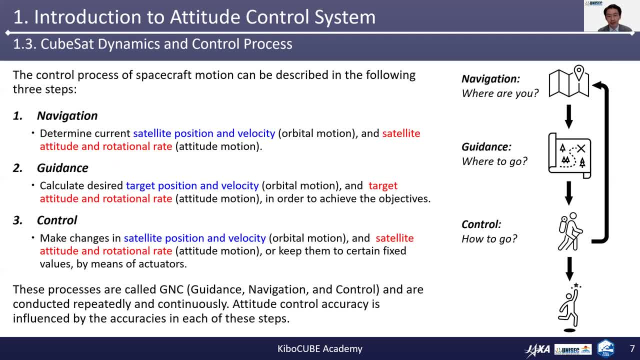 velocity for the orbital motion and the desired target attitude and rotational rate for attitude motion in order to achieve the mission objectives. And the third and last step is control. In the control step, changes are made in the position and velocity of the spacecraft for the orbital motion, as well as the attitude and rotational rate of the spacecraft for 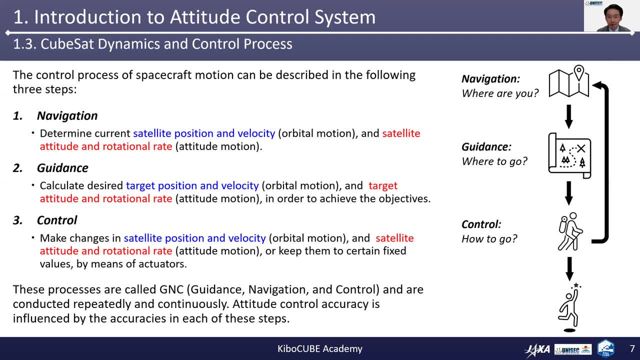 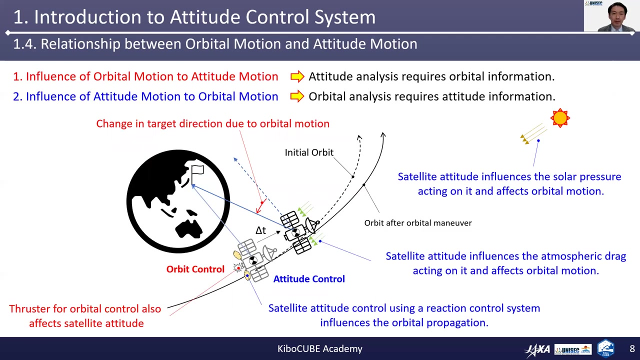 attitude, motion, or even to keep them to certain fixed values by means of actuators. These three important steps are processes which need to be conducted repeatedly and continuously. The resulting control accuracy is influenced by the accuracy in each of these steps. In this next slide, I would like to introduce 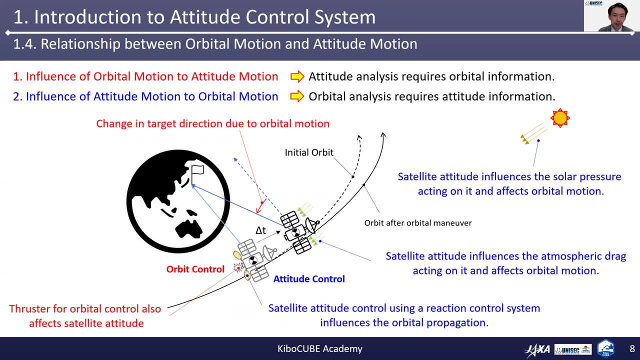 the relationship between orbital motion and actual motion. In the figure below, the inference of orbital motion to actual motion is described by the red characters and the inference of actual motion to orbital motion is in blue. So let's take a look at them one by one. 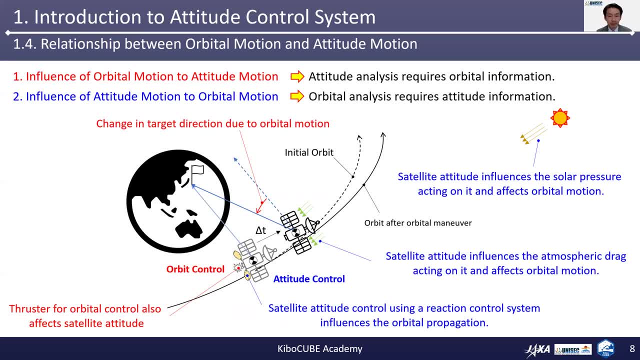 In the case where the satellite is rotating around the Earth, the orbital motion of the spacecraft result in the change of target direction, as illustrated here, And when you conduct an orbital maneuver using thrusters, as illustrated in this figure, it also affects the spacecraft attitude at the same time. 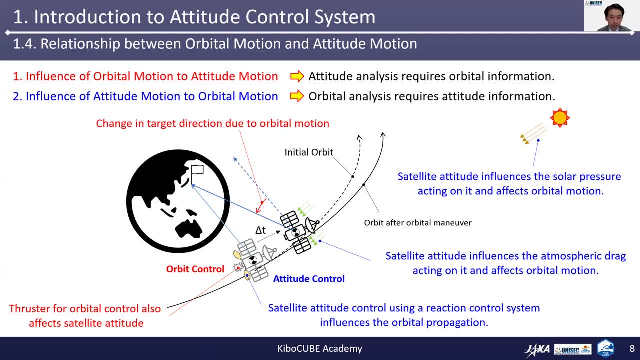 So you need to take into account this perturbation inference to the spacecraft attitude as well while you conduct any orbital maneuver. Then, on the contrary, satellite attitude control using a reaction control system based on thrusters also influences the orbital propagation of the satellite as well. 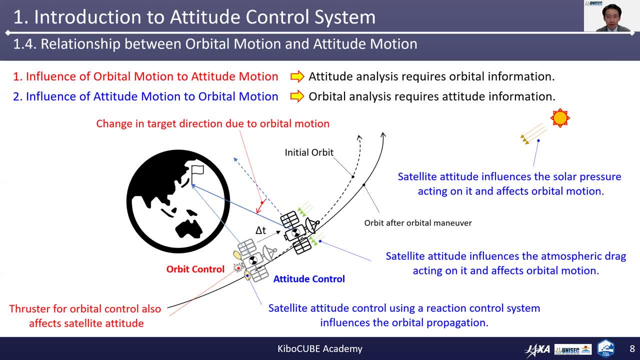 Additionally, the magnitude of solar pressure, of the Earth's atmospheric drag acting on the surface of the satellite, are influenced by the satellite attitude and consequently affects the orbital motion. In this way, the orbital motion and actual motion influence each other And therefore orbital information is required. 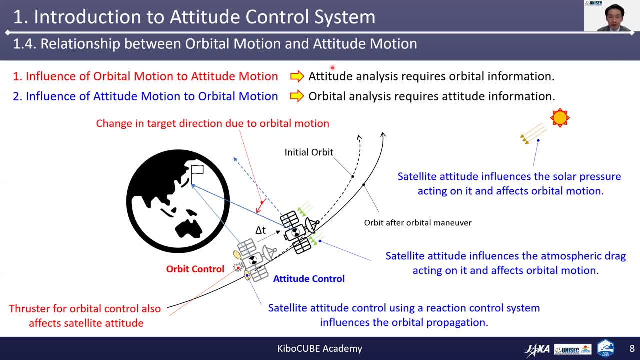 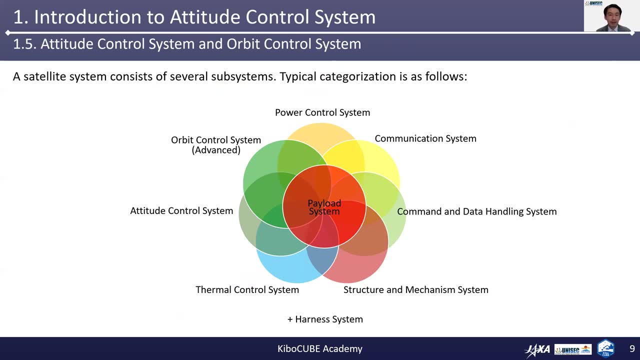 for the actual analysis And the attitude. information is required for the orbital analysis as well. So the main topic of this lecture is the actual control system. You can understand now that it is closely related with the orbit control system. This slide illustrates the relationship. 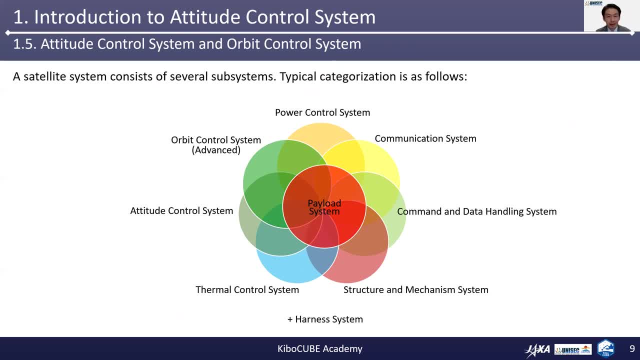 of satellite subsystems. As indicated in the figure, the actual control system and orbital control system are sometimes treated as separate subsystems or they are treated as a single subsystem, referred to as the attitude and orbit control system, or just a-o-C-S For system integration and the systems engineering. 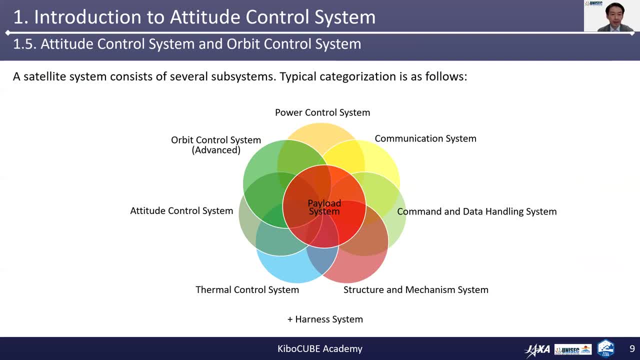 of satellite. it is very important to identify, identify the boundaries between the subsystems and the interfaces between them, as well as their components. The combination of all subsystems except the payload system are denoted as the satellite bus system, And it is also very important to understand 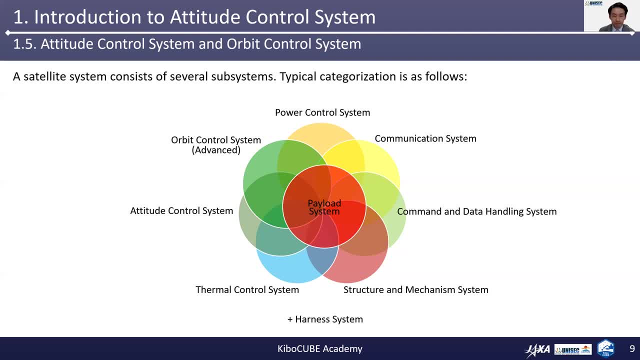 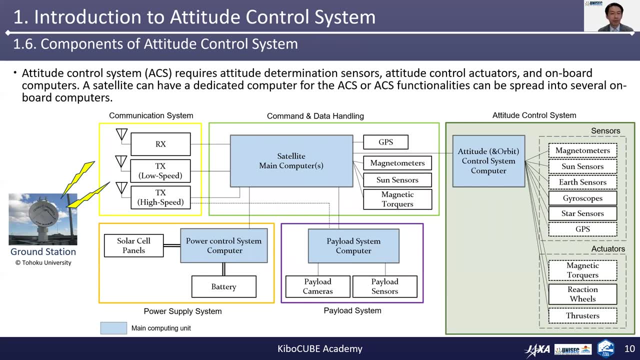 the relationship between the payload and the bus system. This next slide illustrates an exemplary satellite system block diagram, which includes the actual control system and orbit control system. In this way, the satellite system architecture can be described using a system block diagram. Also, satellite components can be categorized into subsystems. 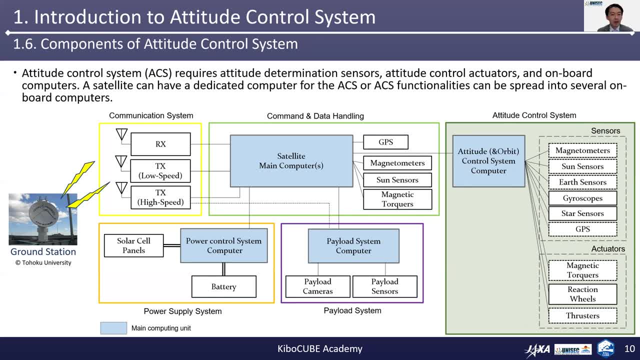 according to their functionalities. Okay, From the diagram you can understand that there are many onboard satellite components which belong to the actual control system and orbit control system. Each of these interfaces need to be specified, controlled, integrated and tested for the satellite system integration. 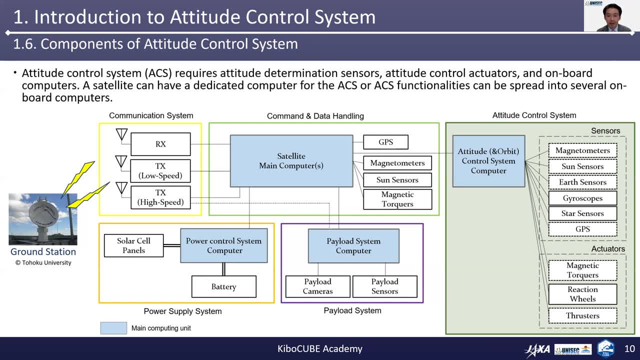 From the left top to bottom right side. the other subsystem illustrated in this figure are the communication system, power supply system, command and data handling system, payload system. In some cases the main computer might be connected to primitive actual determination sensors and actuators. 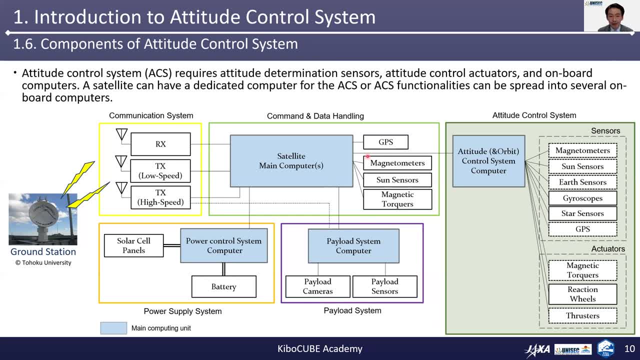 such as magnetometers, san sensors, magnetic torquers and GPS receivers, etc. as indicated in this diagram, In this caseuss. 所以, As indicated in this diagram, In this case the attitude control computer can be turned off, while precise attitude determination. 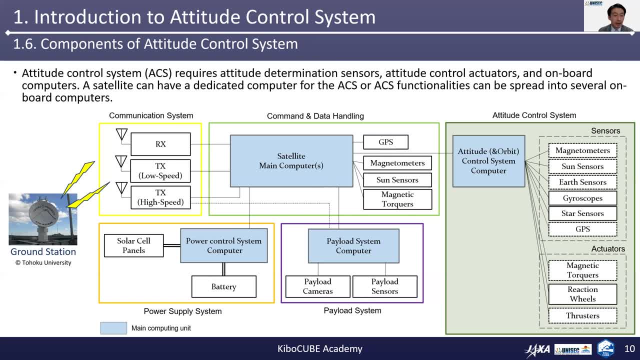 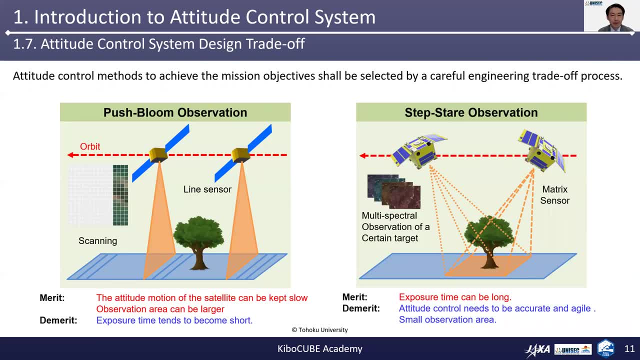 and control is not required so that the satellite can minimize the power consumption. In this slide I have shown you two examples of attitude control methods for Earth observation. The left-hand side figure is illustrating a so-called push-broom observation, which is often used for Earth observations by relatively larger spacecraft in a scanning observation. 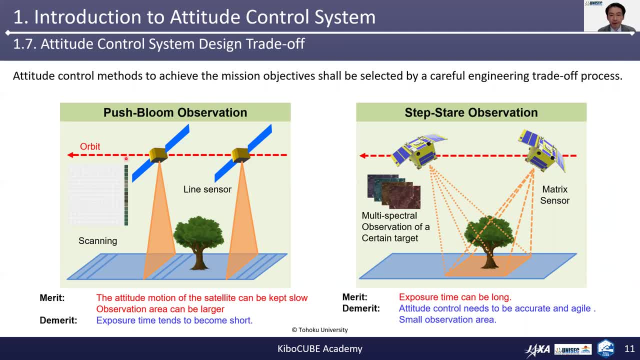 mode, as illustrated in this animation. In this type of control, the attitude motion of the satellite can be kept slow and the observation area can be wider and longer. These are the merits of attitude control. The objective advantage, The objective advantage of this method, is the turnout effect. 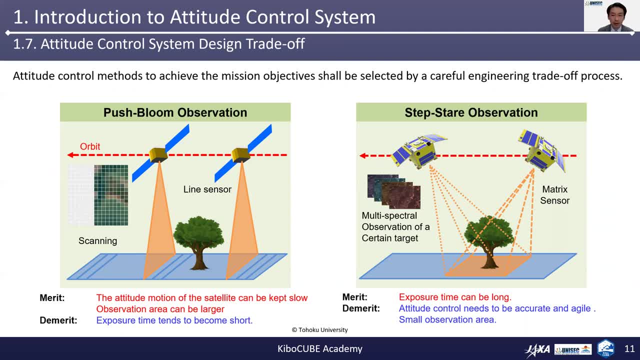 On the contrary, the exposure time tends to be short because of the fast orbital motion relative to the surface of the ground. Its objective advantage. The right-hand side figure illustrates the step stair observation method with target pointing attitude control. The你們 ываем time to get the better signal-to-noise ratio. 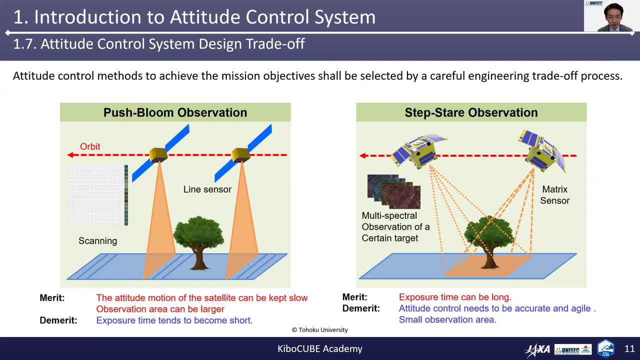 This means we can obtain a better ground sampling distance. However, the challenge in this observation method is that the attitude control needs to be more accurate and agile. Also, the observation area tends to become smaller. The point of the comparison of these two methods is that for the attitude 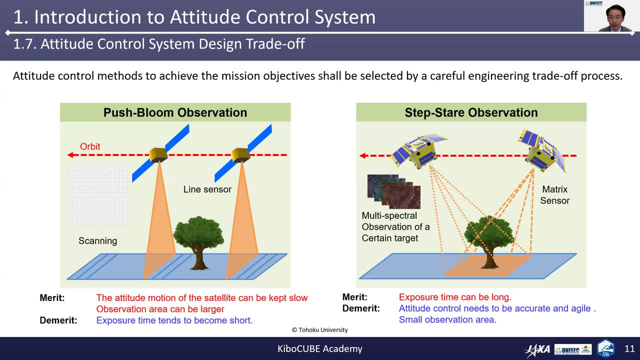 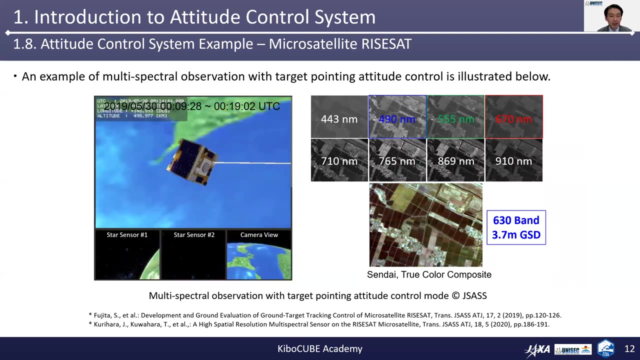 control system design engineers need to conduct careful trade-offs between the attitude control system functionalities, observation capabilities and the project budget, such as the schedule and development cost, et cetera. As an example of a satellite attitude control method, this figure illustrates: 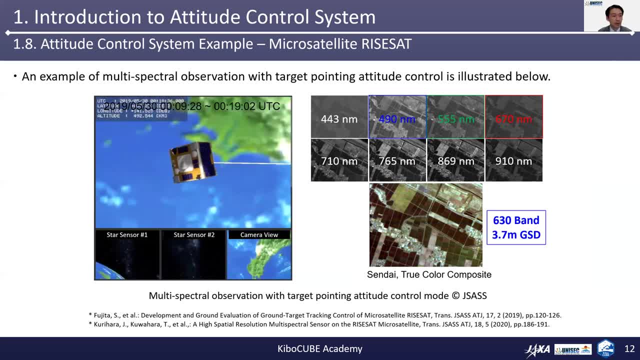 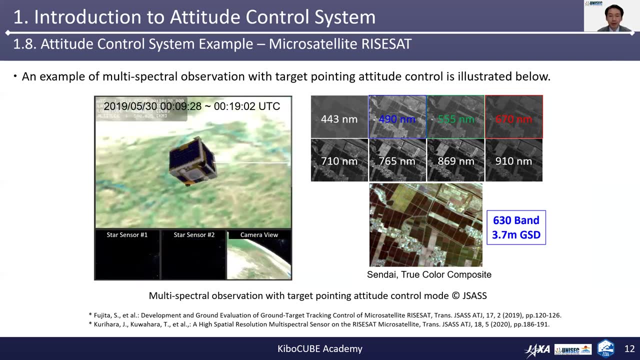 a multispectral observation with target-pointing attitude control, Which was demonstrated by the microsatellite RISE-SAT developed by Tohoku University. This video is showing the satellite attitude conducting target-pointing observation while it flies over the observation targets around Sendai City, Japan. 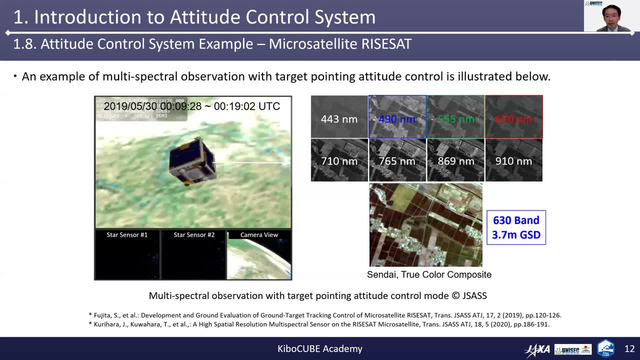 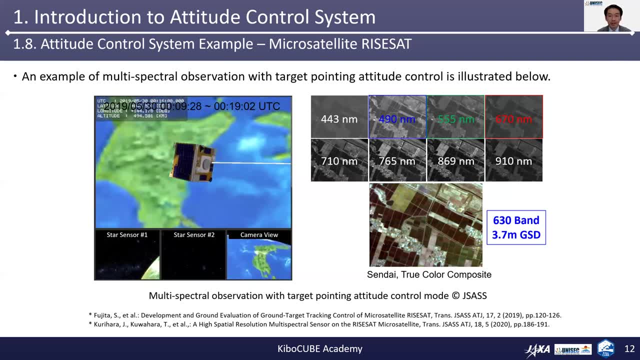 in order to achieve a long exposure time for the target observation with different wavelengths. Doing so allows the combination of some of the wavelengths to generate meaningful scientific data after the observation. This is illustrated on the right-hand side figure. I hope that you could get an idea of how the attitude control of satellites takes place. 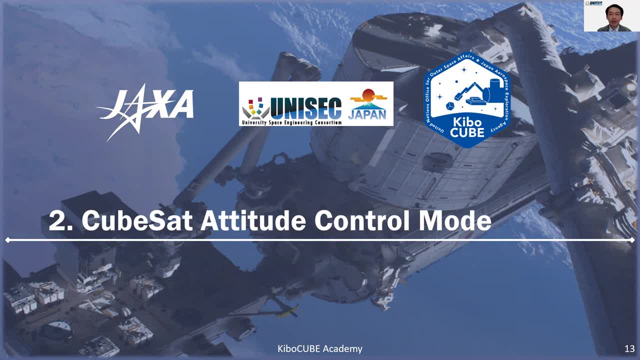 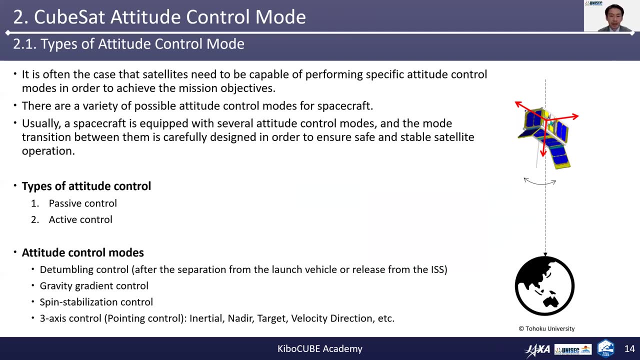 In this next chapter, Let me explain how the attitude control of satellites takes place. Let me now introduce the CubeSat attitude control modes. It is often the case that satellites need to be capable of performing specific attitude control modes in order to achieve mission objectives. 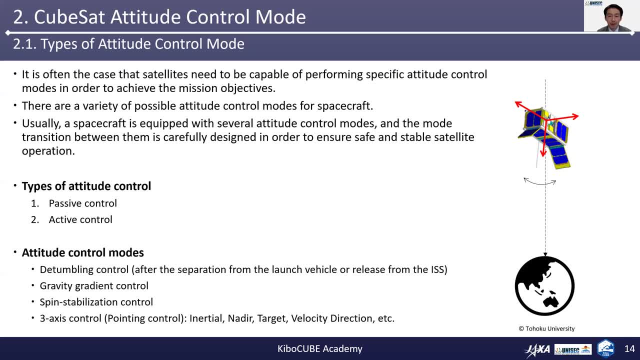 There are a variety of possible attitude control modes for satellites. Usually, a satellite is equipped with several attitude control modes, And the mode transitions between them are carefully designed in order to ensure safety and stable satellite operation in space. From time to time, these need to be autonomous. 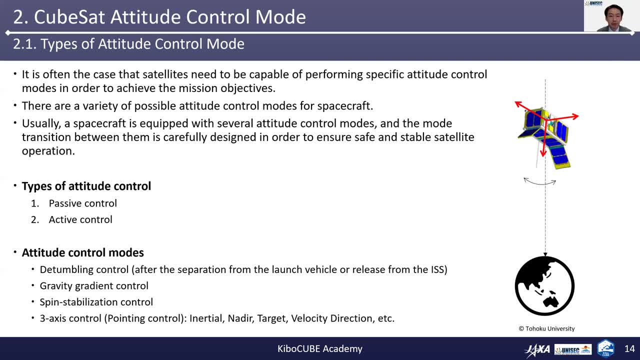 For the attitude control. attitude determination is also necessary beforehand. Therefore, attitude determination sensors and attitude control actuators are required. in general, There are two types of attitude control: passive and active controls. There are many different kinds of attitude control modes. They are the tumbling control. 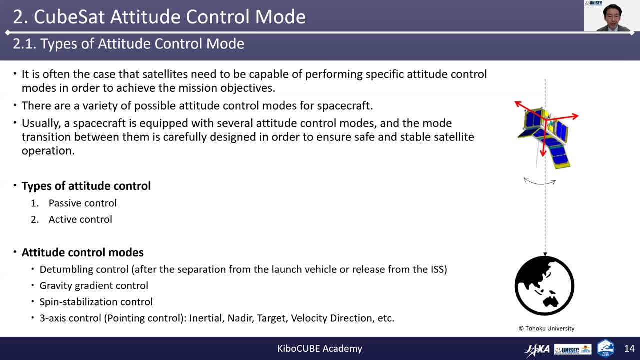 which retumbles the satellite rotational velocity after the separation from the launch vehicle or release from the ISS. Gravity gradient control using passive gravitational torque acting on the satellite rotation velocity on the satellite spin stabilization control and three-axis control, including pointing control, such as inertial nadir, target, velocity, direction pointing and so on. 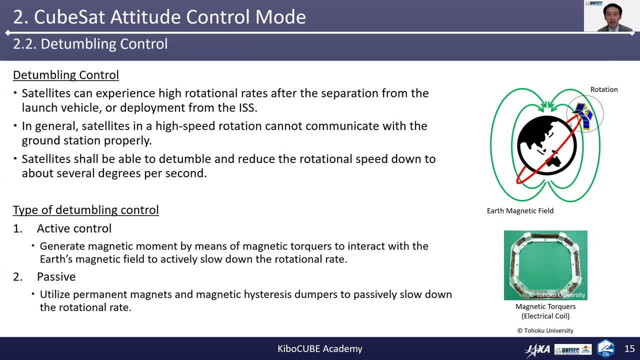 In the following slides I'd like to elaborate about the actual control modes. One of the most important actual control modes is seat determining. control Satellites can experience a high rotational rate after the separation from the launch vehicle or release from the ISS. In general, satellites in high-speed rotation cannot communicate with 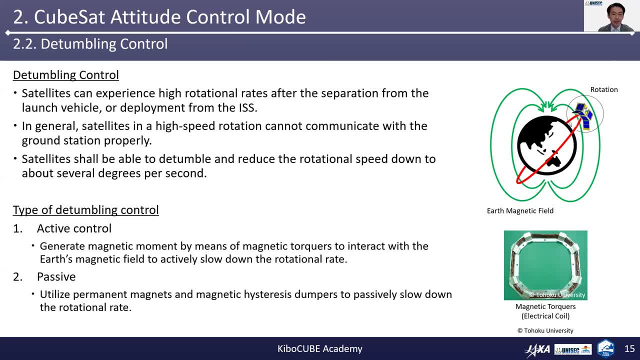 the ground station properly, Satellites shall be able to detumble and reduce the rotational speed down to about several degrees per second at the maximum. There are two types of detumbling controls: active control and passive control. For the active control, in general you generate 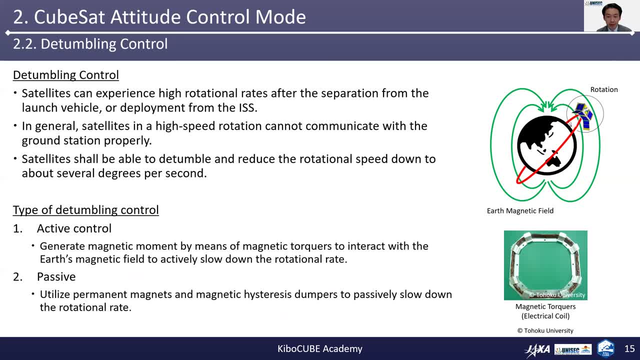 a magnetic moment by means of magnetic torquers to interact with the Earth's magnetic field, actively slowing down the rotational rate. This is illustrated in the figure For the passive control. you utilize permanent magnets and the magnetic hysteresis to generate magnetic torquers to interact with the Earth's magnetic field. 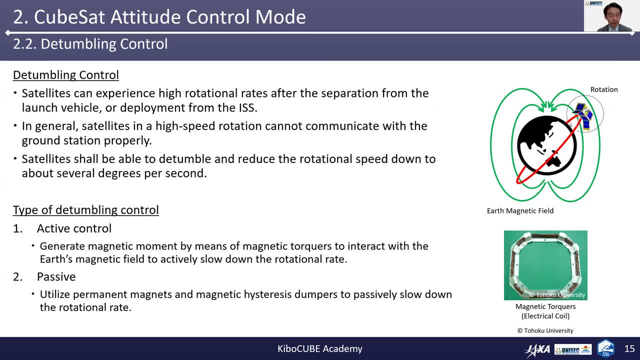 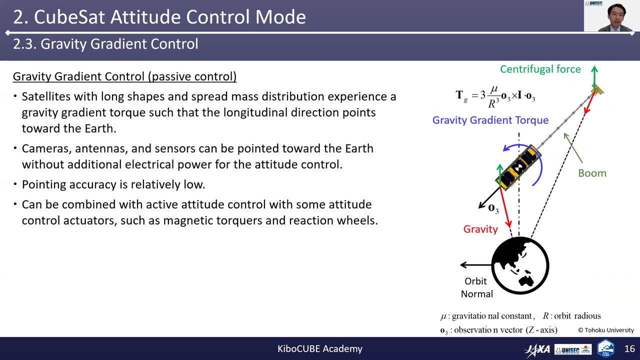 For the active control you utilize permanent magnets and the magnetic hysteresis dampers to passively slow down the rotational rate. This picture is an example of a magnetic torquers. Another interesting actual control method is the gravity gradient control. The gravity gradient control belongs to the passive control category: Satellites with long 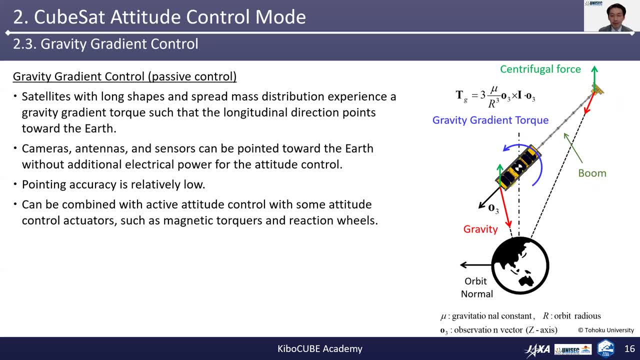 shapes and a spread mass of a certain size are called passive control. The spread mass distribution experiences a gravity gradient torque such that the longitudinal direction points toward the earth. The cameras, antennas and sensors can be pointed toward the Earth without additional electrical power or actual control. 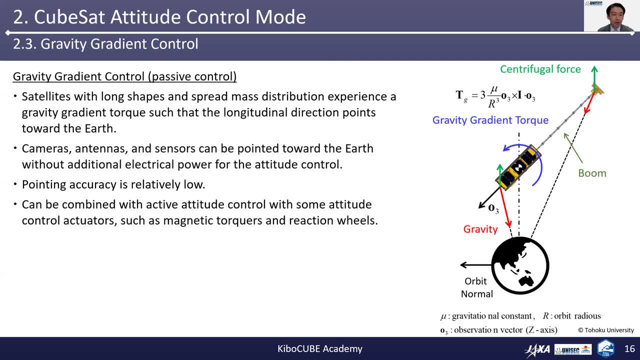 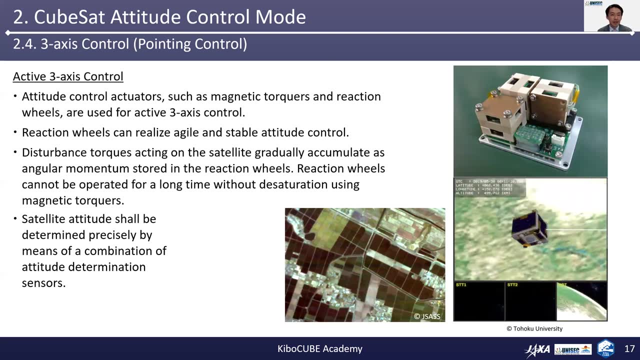 But the pointing accuracy is low. This can also be combined with active actual control with some actual control actuators such as magnetic torquers and reaction wheels. The last example of actual control is the active three-axis actual control. Actual control actuators such as magnetic torquers and reaction wheels are used for 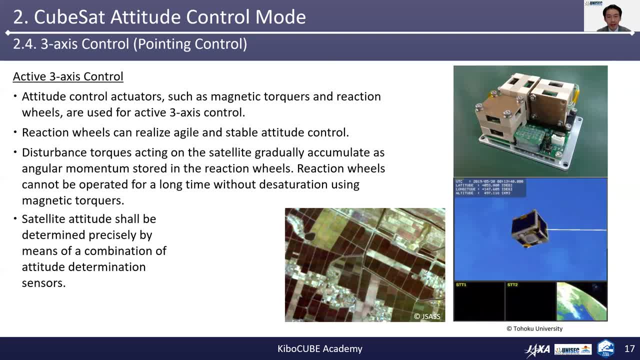 active three-axis control, And specifically reaction wheels, can realize agile and stable actual control. This is shown in the animation. Through three-axis actual control you can point your camera instruments toward the observation target. You can then obtain this kind of image by: 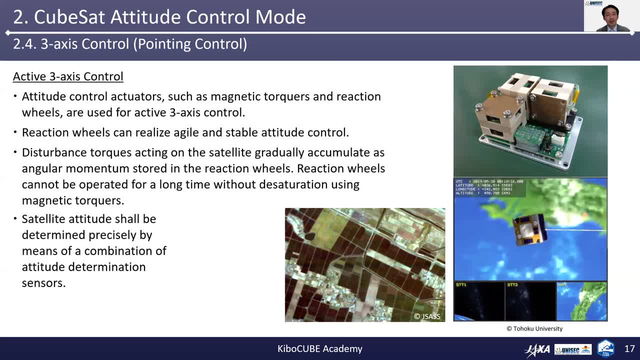 your satellite. Disturbance torques acting on the satellite gradually accumulate as angular momentum stored in the reaction wheels, And therefore reaction wheels cannot be operated for a long time without desaturation using magnetic torquers. Also, I need to mention 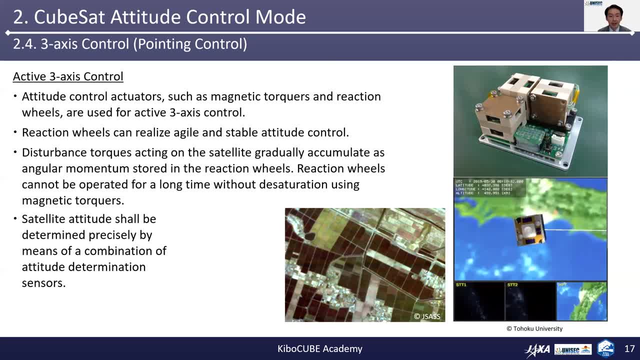 that for this method of actual control, the satellite actual shall be determined precisely by the reaction wheels. This is shown in the animation. Through three-axis actual control, we can estimate theısall aquilozientras Catherine by means of a combination of actual determination sensors. 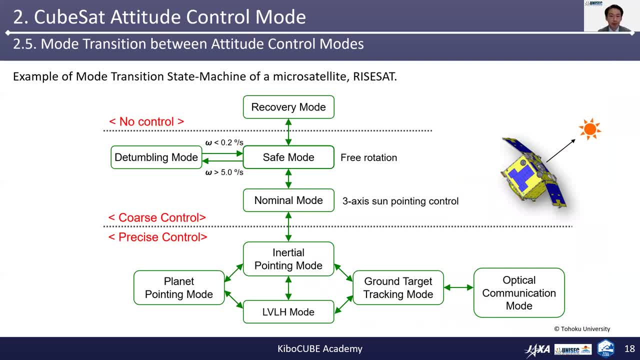 This slide illustrates the implemented actual controller modes over the spacecraft and their state-transition diagram. This is an example of the microsat right right side developed by the Tohoku University. Usually this gigs for the, the actual control system, Definitely components or instrument you are already familiar with, can offer quite aremo of post-diagnostics. moving to stack, controlar data spend in the different directions possible In the tools which, Dziękuję repeat, have shown deep effects. results现在 about the. whichever node you plug in, you should get the people who are peeking. is that of the marquee that way? Or these nodes are directly connected to, such as the: 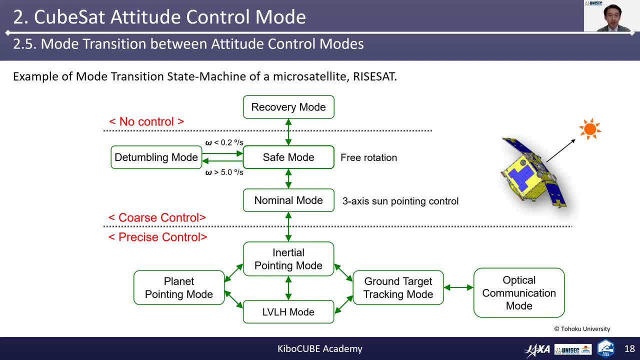 active three-axis factors. Therefore, the weak point of usable interaction means that the to identify what kind of actual control modes are required to achieve the mission objectives of the satellite, Those actual control modes need to be combined in a state machine diagram, as illustrated in this slide, together with the mode transition conditions between them. 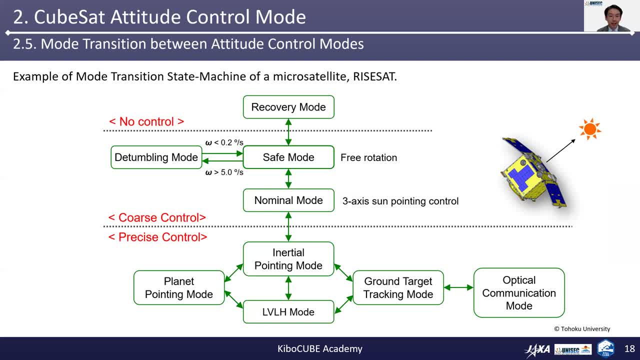 Mode transition can be triggered either by the telecommand sent from the ground station or autonomously based on the internal parameters by the onboard computers, such as satellite angular velocity. So in this example the automatic mode transitions are implemented between safe mode and the tumbling mode. 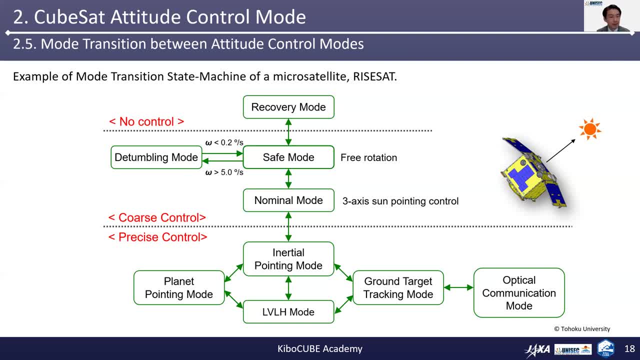 In this example, if the angular velocity becomes bigger than five degrees per second, the satellite autonomously and automatically starts the tumbling mode to detumble the rotational velocity in order to achieve stable satellite operation, And if the angular velocity becomes lower than 0.2 degrees per second, it comes back to the safe mode. 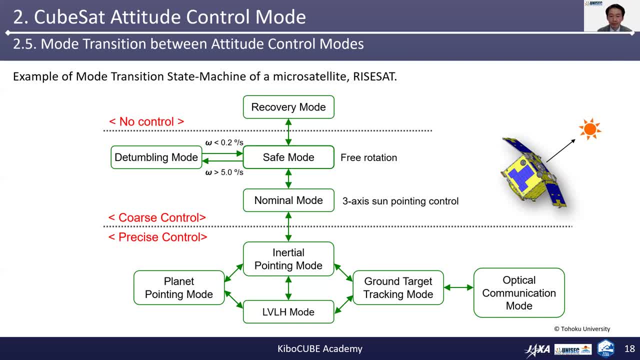 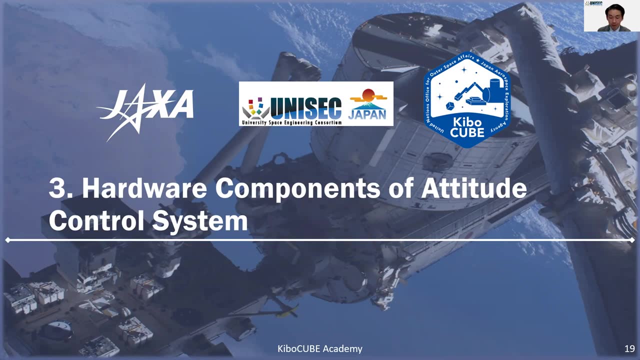 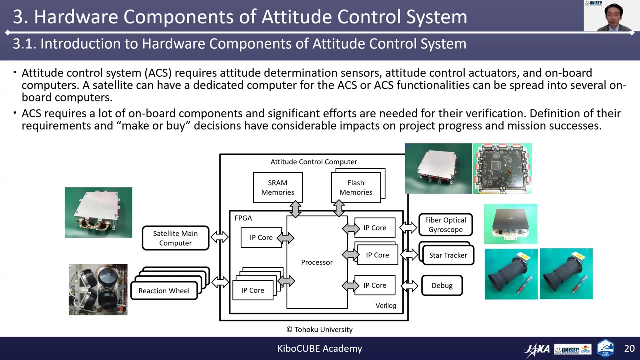 The attitude control system is a complex system which requires attitude detection sensors, behaves manually and automatically and onboard computers In general. a satellite can have a dedicated computer for the ACS or ACS functionalities can be spread into several onboard computers. ACS requires a lot of onboard components and significant efforts are needed for the verification. 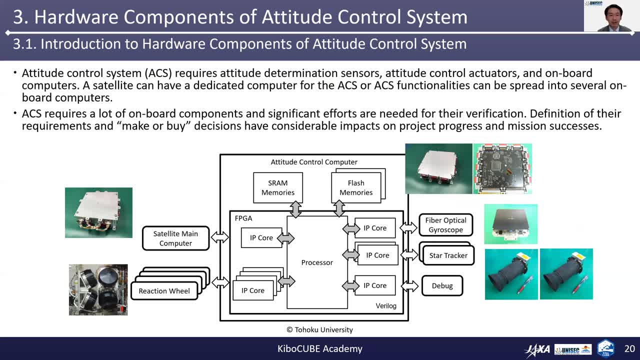 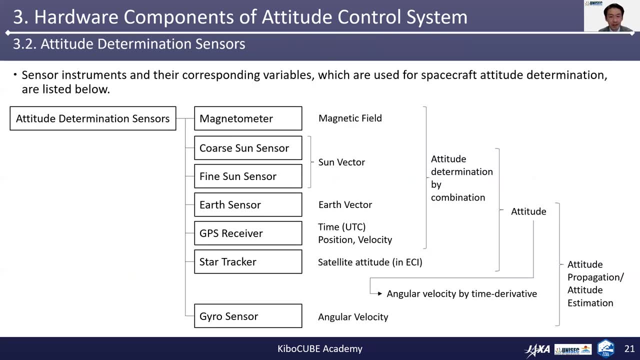 You need to pay attention to the fact that the definition of their requirements and make or buy decisions have considerable impacts on the project progress and mission success. In this slide I have summarized the actual determination sensors. These are the sensors commonly used for satellite actual determination. 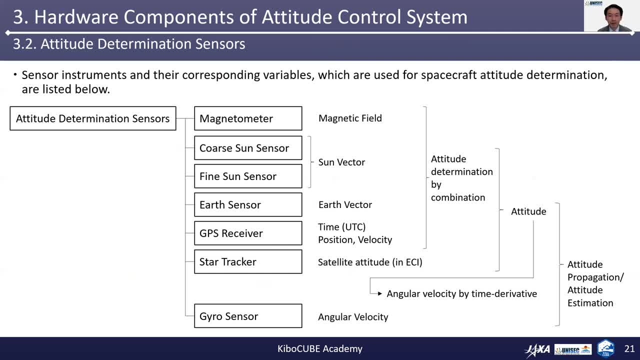 The first one is the magnetometer, which measures the magnetic field. The second one covers a family of sun sensors, including the coarse sun sensor and fine sun sensor. These sun sensors measure the sun vector. The next sensor is an earth sensor, which measures the earth vector or the direction of the earth center. A GPS receiver is used to obtain time information. 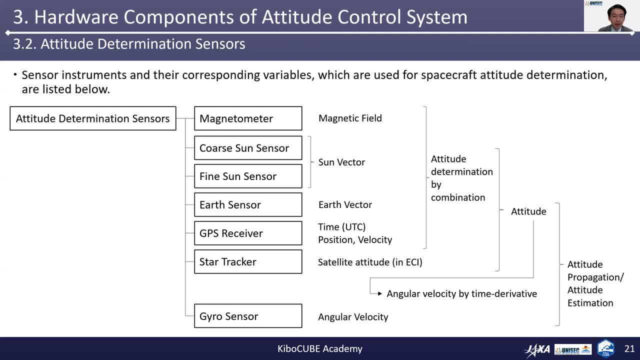 such as UTC and time. The GPS receiver is used to obtain time information such as UTC and time. This lookcat sensor is used to track shooting speed information and satellite position and velocity. The next sensor is a Star tracker which directly determine the satellite attitude in the internal inertial coordinate. 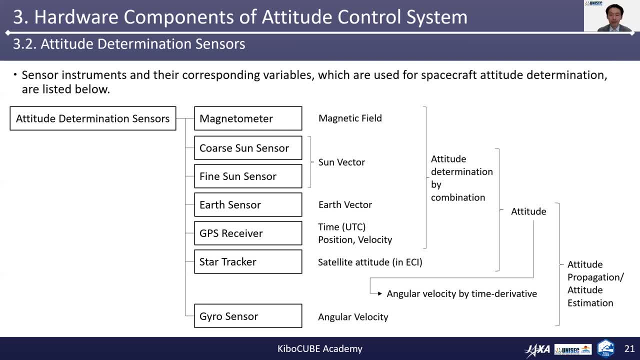 Last one is the gyro sensor, which measures the angular velocity or angular rate of the satellite, As indicated in this slide. также一 любов体 zero believe the今天的地球是一. Oscilla diagram. the first set of these sensors are used to determine the satellite attitude by 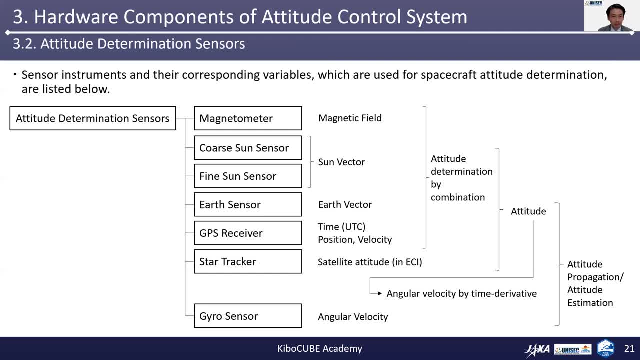 combining their obtained data, The star tracker can determine the satellite attitude alone and therefore out of these sets of sensors we can obtain the satellite attitude information For the attitude propagation or attitude estimation indicated at the right. we need not only the 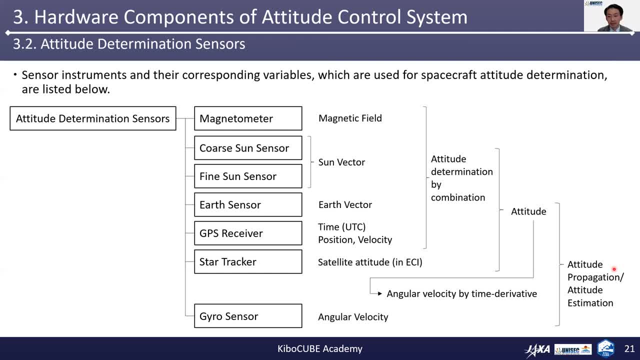 attitude information of the satellite, but also the angular velocity, which can be measured directly by gyro sensors or derived from the attitude information by taking its time derivative. We need to combine these parameters in order to determine the satellite attitude in the onboard computer. 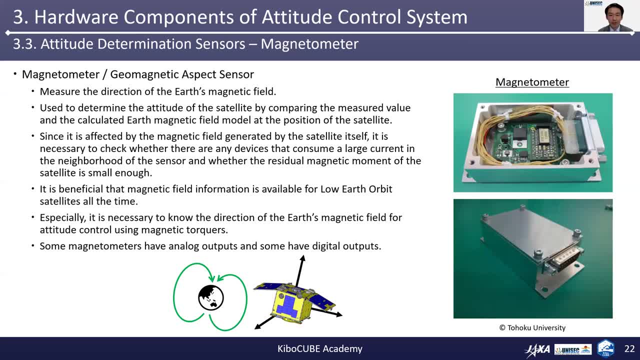 In the following slides I'd like to introduce the attitude determination sensors one by one. The first one is the magnetometer, also known as a geomagnetic aspect sensor. Magnetometers measure the direction of the Earth's magnetic field. It is used to determine the attitude of the satellite by comparing the measured value and the calculated. 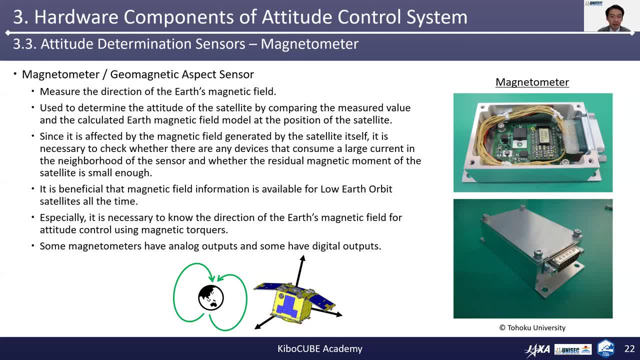 Earth's magnetic field model at the position of the satellite. Since it is affected by the magnetic field generated by the satellite itself, it is necessary to check whether there are any devices that consume a large current in the neighborhood of the sensor And whether the residual magnetic moment of the satellite is small enough. 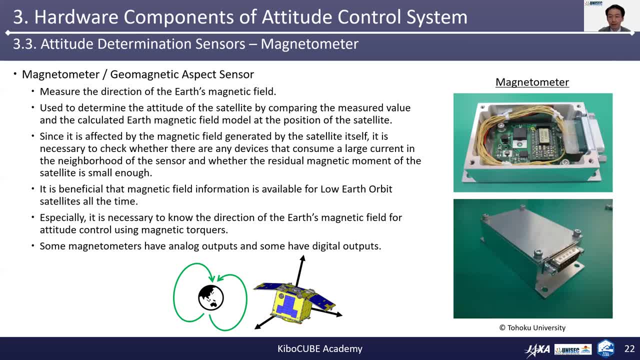 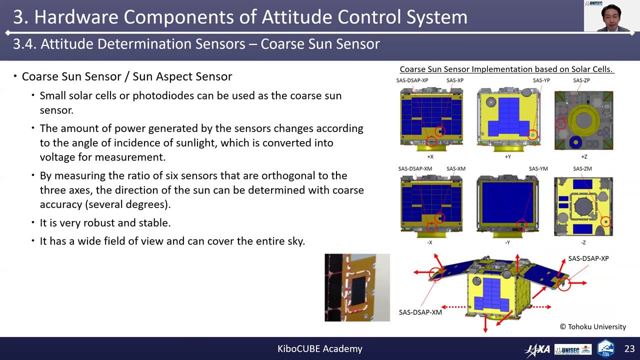 It is beneficial that magnetic field information is available for low Earth orbit satellites all the time, So it is especially necessary to know the direction of the Earth's magnetic field for actual control using magnetic torquers. Okay, Any other questions? Then I'd like to introduce the sensor. 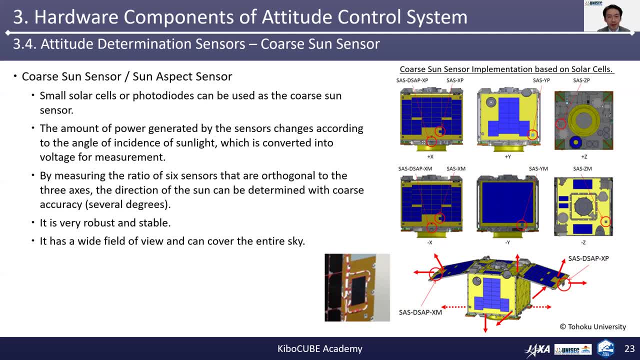 Once again, the sensor is placed inside the centre of the subject, not in the center of the image. In the same way, it is a very reliable sensor because it has a large dynamic force and the same function as a magnetic field sensor. It is a very reliable sensor. 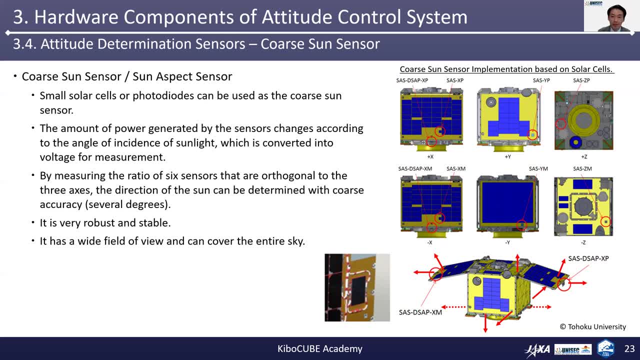 It is a very reliable sensor because it has a large dynamic force and the magnetic force from the center of the subject can be used to measure the magnetic field of incidence of sunlight, which is converted into voltage for the measurements By measuring the ratio of six sensors. 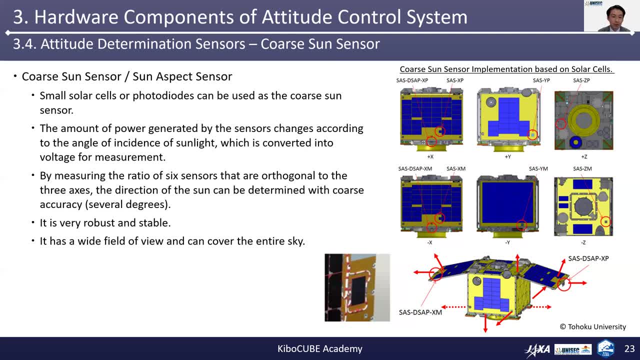 on each surface of the satellite that are all to the three axis. the direction of the sun can be determined with close accuracy, with several degrees. It is very robust and stable And it has a wide field of view and can cover the entire sky. 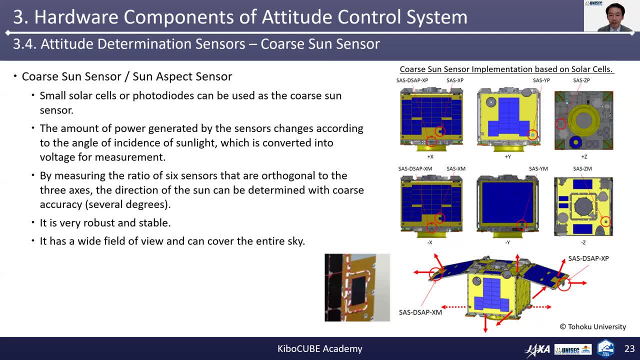 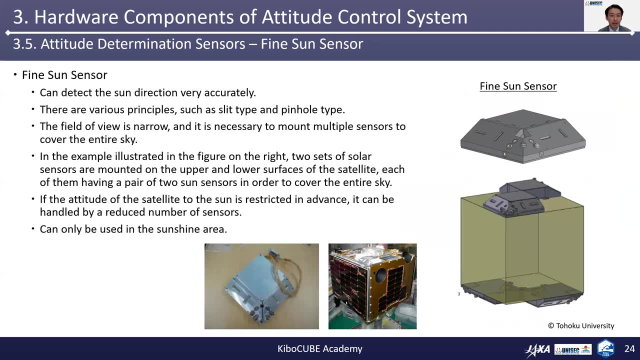 In the right-hand side of this slide, an implementation example in the case of microsat- ISAT- is illustrated. The next one is the fine sun sensor. Fine sun sensors can detect the sun's direction very accurately. There are various principles, such as slit type. 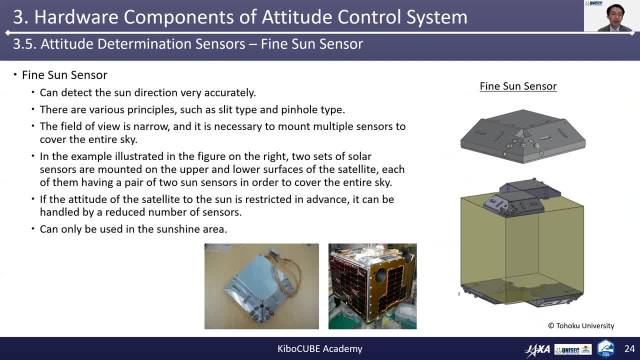 and pinhole type. The field of view is narrow and it is necessary to mount multiple sensors to cover the entire sky. In the example illustrated in the figure on the right, two sets of solar sensors are mounted on the upper and lower surfaces of the satellite. 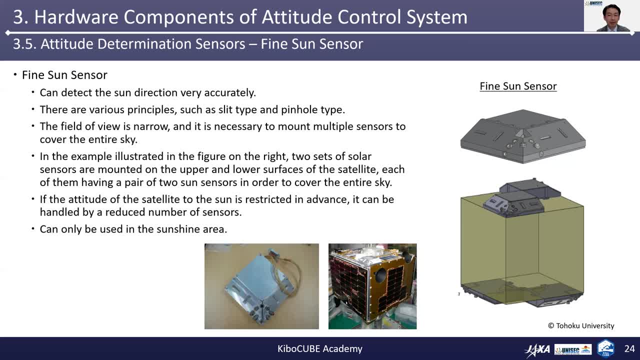 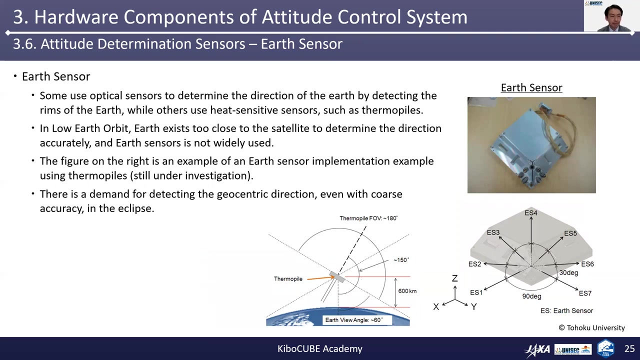 These are not perfect or reasonable banana tree organisms. they have no impasse activity. the earth sensor: Some earth sensors use optical instruments to determine the direction of the earth's center by detecting the rims of the earth, while others use heat sensitive sensors. 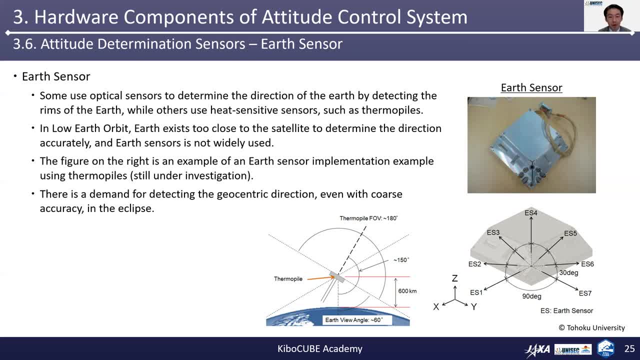 such as sound piles In low earth orbit. earth exists too close to the satellite to determine the direction accurately, and hence earth sensor is not widely used. The figure on the right is an example of an earth sensor implementation using sound piles, which is still under investigation at Tohoku University. 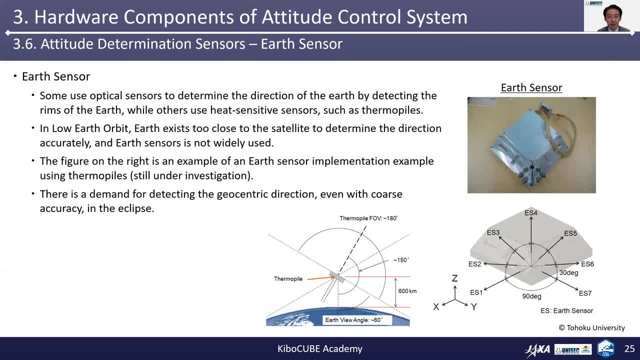 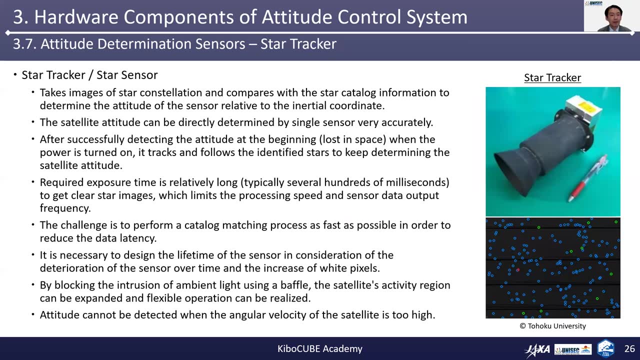 There is a demand for detecting the geocentric direction, even with course accuracy, especially in the eclipse side of the earth. as you cannot have information about the sound vector, The next sensor is the star tracker, also called a star sensor, A star tracker. 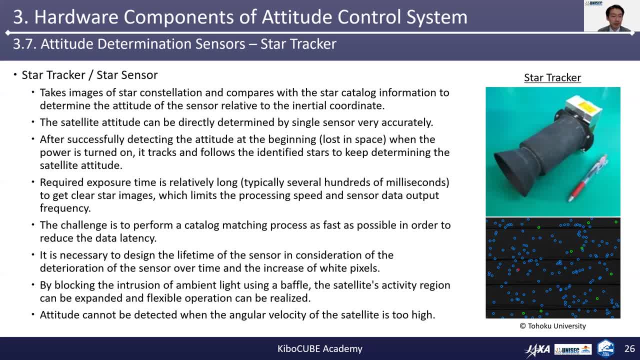 developed by Tohoku University is illustrated in the right hand side picture. Star trackers take images of star constellations and compare them with the internal star catalogue information to determine the attitude of the sensor relative to the inertial coordinate. The satellite attitude can be directly determined. 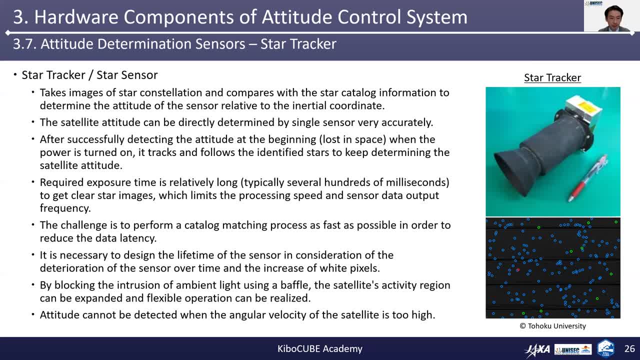 by a single sensor very precisely After successfully detecting the attitude at the beginning when the power is turned on, which is called a lost in space situation. the tracker tracks the identifiable stars and the initial detection date can be determined by a broadcast means which was developed by the satellite. The star tracker tracks and follows. 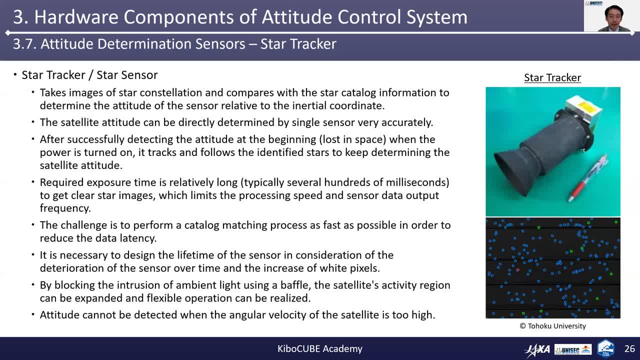 the identified stars to keep determining the satellite attitude. The required exposure time is relatively long, which is typically several hundreds of milliseconds, to get clear star images, which limits the processing speed and sensor date output frequency. to perform a catalog matching process as fast as possible inside the sensor in order to 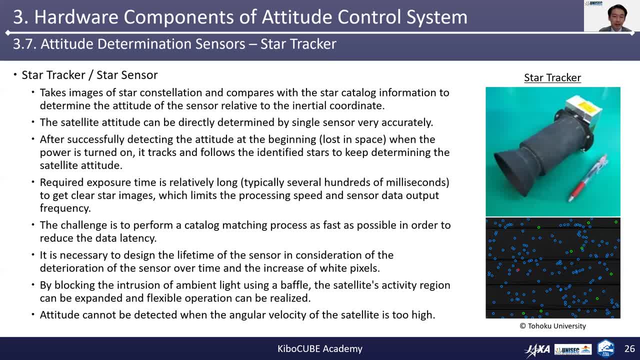 reduce the data latency. It is necessary to design the lifetime of the sensor in consideration of the deterioration of the sensor over time and the increase of white pixels. By blocking the intrusion of ambient light using a baffle, the satellite's activity region can be expanded and flexible operation can be realized. 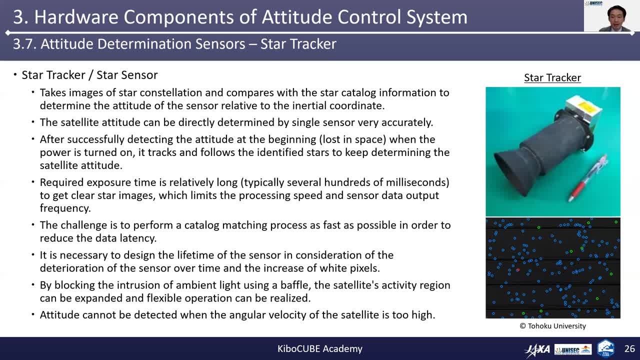 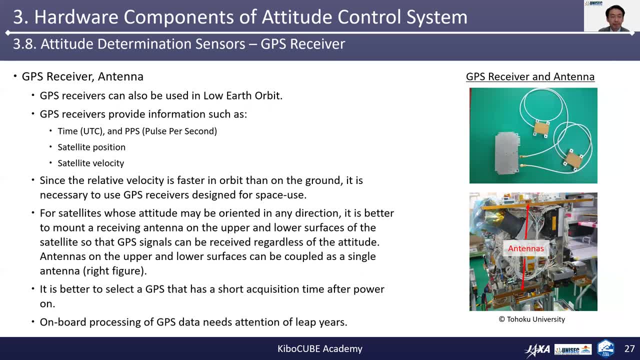 Note that attitude cannot be detected by star trackers when the angular velocity of the satellite is too high. The next sensor is the GPS receiver and antenna. GPS receivers can also be used in low-Earth orbit. in space, A GPS receiver provides information such as time in UTC and PPS and satellite. 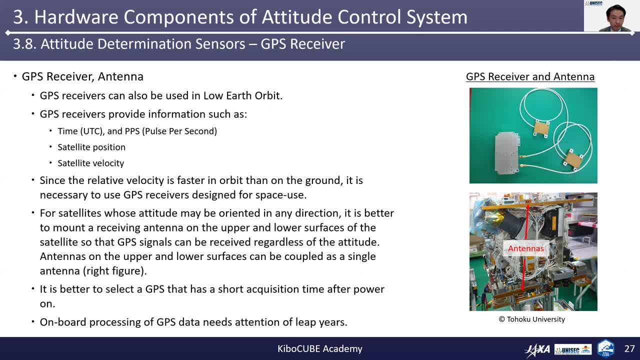 position, satellite velocity, etc. Since the relative velocity is faster in orbit than on the ground, necessary to use a GPS receiver designed for space use For satellites whose attitude may be oriented in any direction. it is better to mount a receiving antenna on the upper and lower. 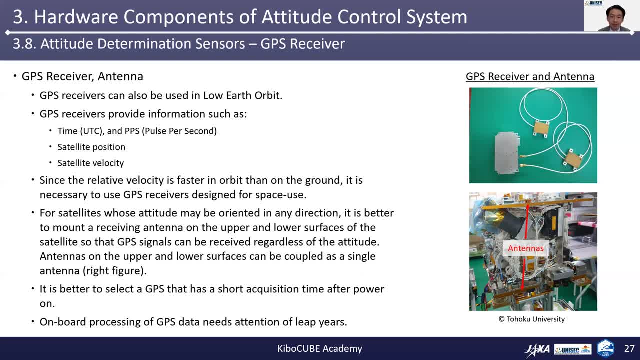 surfaces of the satellite so that GPS signals can be received regardless of the attitude. Antennas on the upper and lower surfaces can be coupled as a single antenna, as illustrated in the right figure. It is better to select a GPS that has a short acquisition time after the power on. 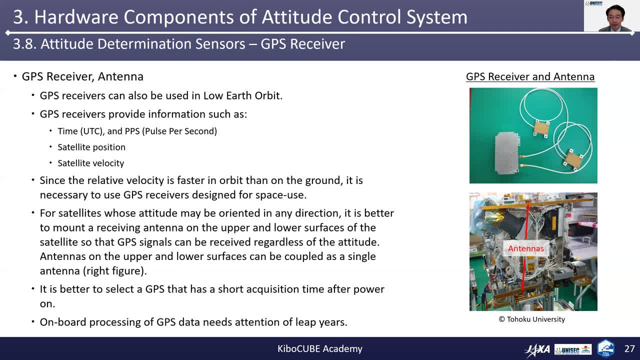 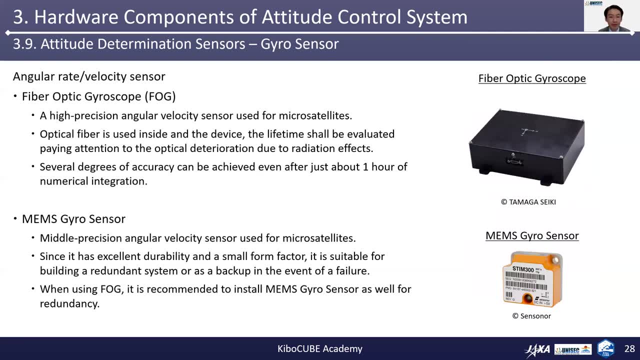 On-board processing of GPS data needs to pay attention to leap years as well. The last sensor is the angular rate Angular velocity sensor. The first one I will introduce is the fiber optic gyroscope, or just FOG. FOG is a high precision angular velocity sensor. 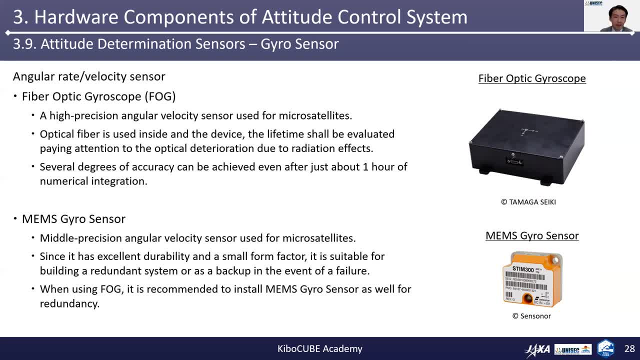 used for microsatellites. Optical fiber is used inside and the device lifetime shall be evaluated by paying attention to the optical deterioration due to the radiation effect. Several degrees of accuracy can be achieved even after about one hour of numerical integration. The second one I will introduce is the MEMS gyro sensor. 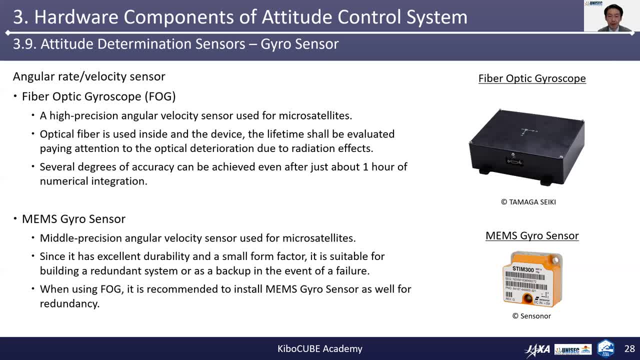 It is a middle precision angular velocity sensor used for microsatellites. Since it has excellent durability and a small form factor, it is suitable for building a redundant system Or for use as a backup in the event of failure. When using FOG, it is recommended to install MEMS gyro sensor as well for redundancy. 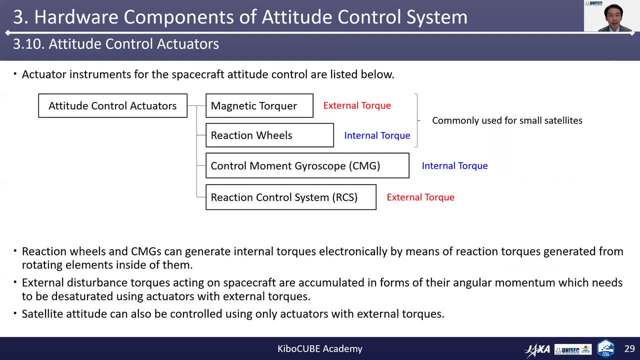 The next group is the actual control actuators. This slide illustrates the families of the actual control actuators. These are magnetic torquers, Reaction motors, Reaction wheels, Control moment gyroscope or just CMG, And reaction control system or just RCS based on thrusters. 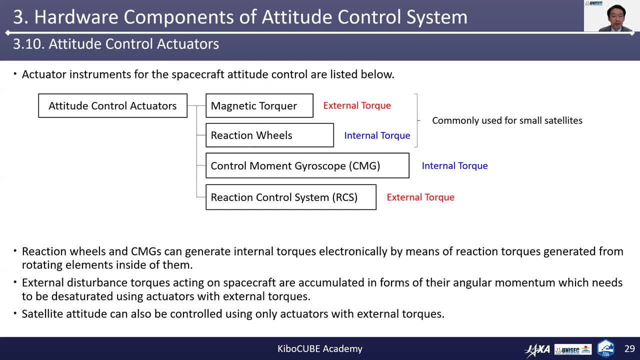 The magnetic torquers and reaction control system generates external torques, while reaction wheels and control momentum gyroscopes generate internal torques For CubeSats. the first two actuators, which are magnetic torquers and reaction wheels, are commonly used for actual control. 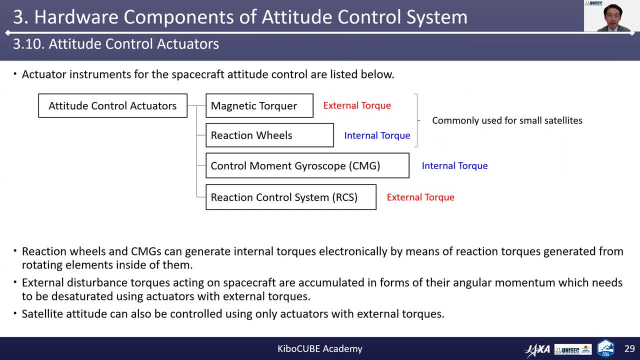 Reaction wheels and CMG can utilize internal torques generated from rotating elements inside of them. The external disturbance torques acting on satellites are accumulated in the form of the angular momentum inside. This load needs to be desaturated using actuators which can generate external torques for long. 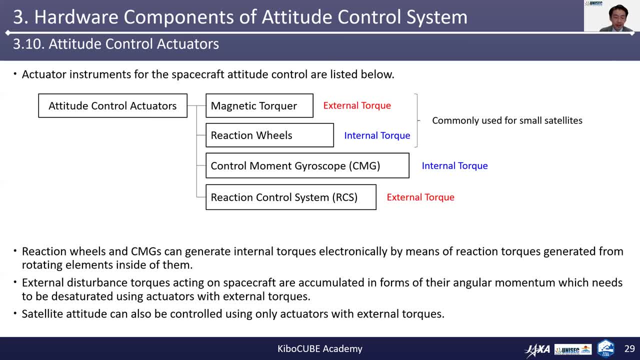 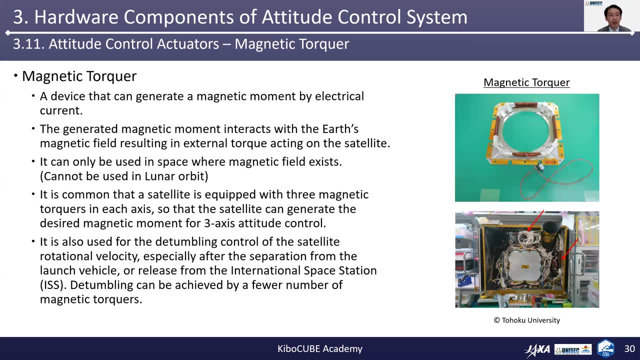 operation time Satellite attitude can also be controlled using only actuators with external torques as well, such as magnetic torquers. In the following slides I'd like to introduce the actual control actuators one by one. The first actuator is the magnetic torquer. 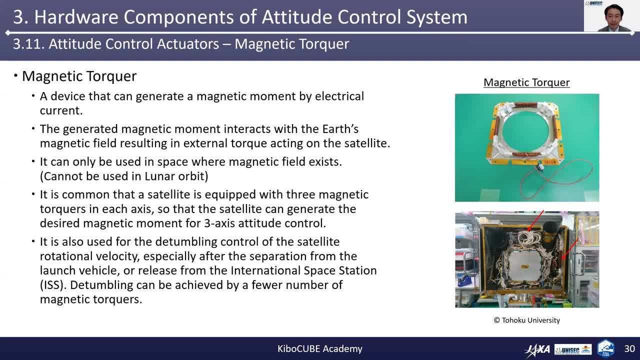 A magnetic torquer is a device that can generate a magnetic moment by electrical current. The generated magnetic moment interacts with the earth's magnetic field, resulting in external torques. It can only be used in space where a magnetic field exists. therefore, it cannot be used. 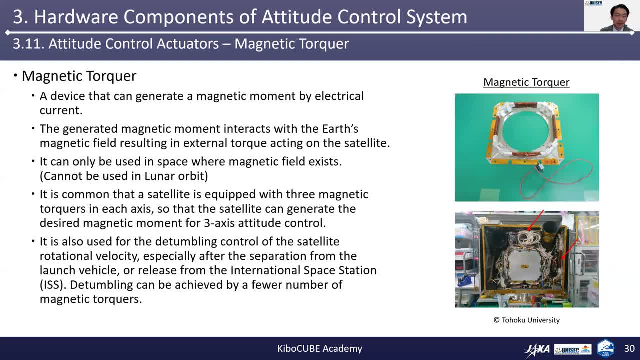 in lunar orbit, for example, as there is no magnetic field, It is common that a spacecraft is equipped with three magnetic torquers in each axis, so that the satellite can generate the desired magnetic moment for three axes. The second actuator is the magnetic torquer. 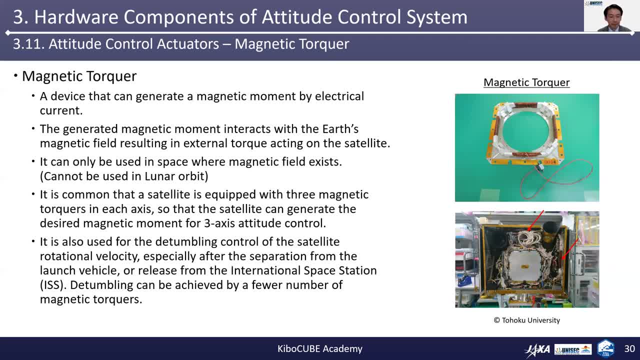 It can only be used in space where a magnetic field exists, so that the satellite can generate the desired magnetic moment for three axes. This is the actual control of the v-axis. It is also utilized for the tampering control, for instance after the separation from a launch. 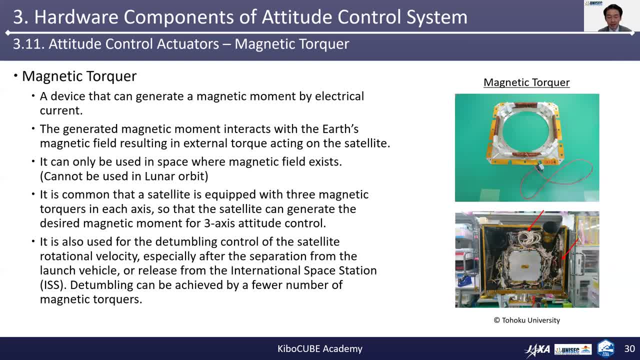 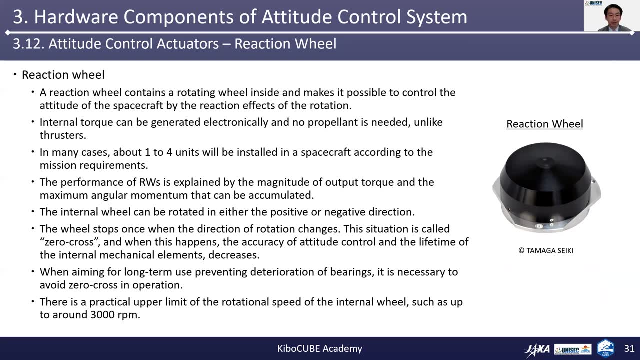 vehicle or after the apprenticeship, from a space spacecraft. The tampering control can be achieved by the use of a stronger magnetic torquer. The谢谢 actuator is a different action. It is strongly heating the natural energy of the aerobatics. 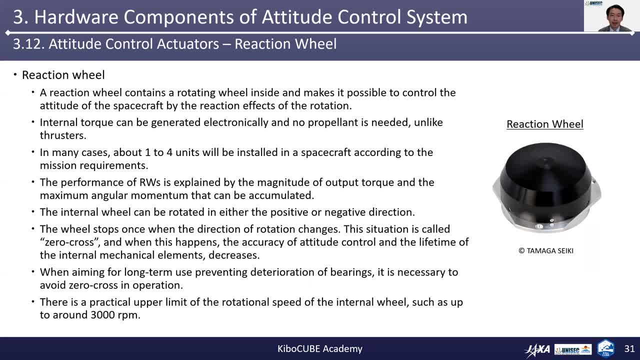 This activity forces the light and gravity to fuse, For example, if, for example, fishtank can be pulled, Sesha and China while switching from one side to another. it will therefore turn andそれでə causes the light-and- delighted. A reaction wheel contains a rotating wheel inside and makes it possible to control the. 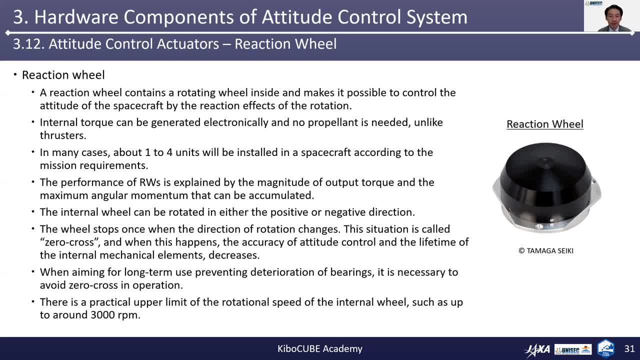 action of the satellite by the reaction effects of the rotation. Internal torque can be generated electronically and no propellant is needed, unlike thrusters. In many cases, about 1 to 4 units will be installed in a satellite, according to the mission requirements. 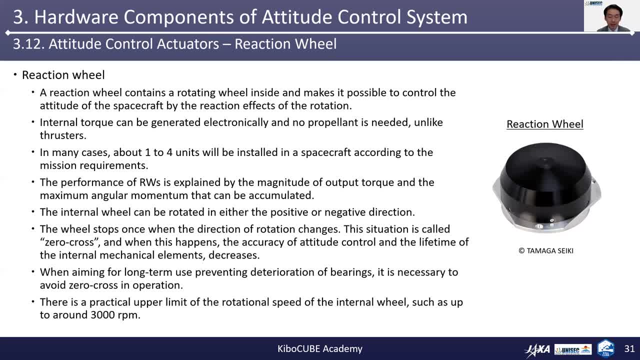 The performance of reaction wheels is explained by the magnitude of output torque and the maximum angular momentum that can be accumulated. The internal wheel can be rotated in either the positive or negative direction. The wheel stops at the maximum angular momentum. The wheel stops once when the direction of rotation changes. 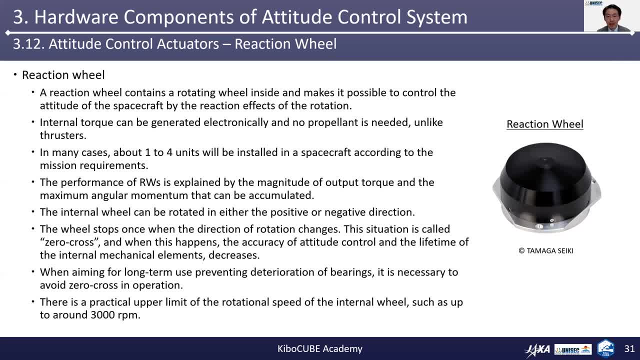 This situation is called zero-cross and when this happens, both the accuracy of the actual control and the lifetime of the internal mechanical elements decreases. When aiming for long-term use by preventing deterioration of bearings, it is necessary to avoid zero-cross in operation. 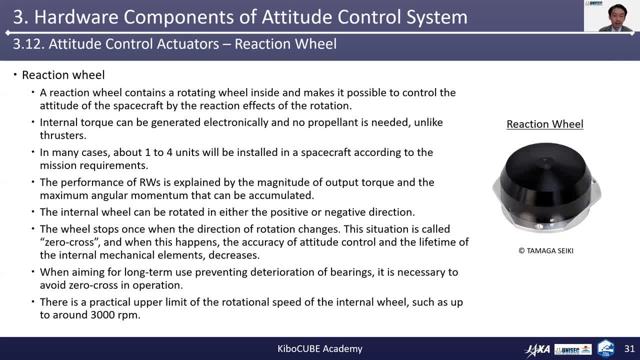 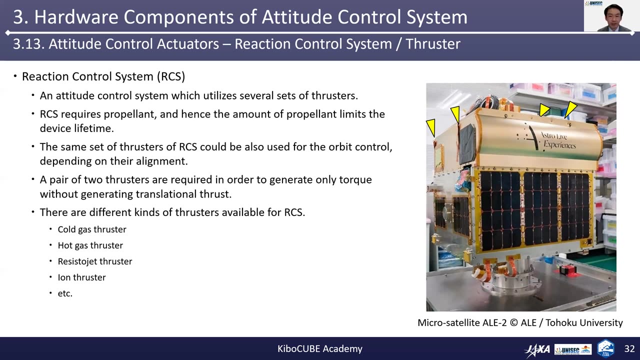 There is a practical upper limit of the rotational speed of the internal wheel, such as up to around 3,000 rpm, and so on. The next one I introduce is the reaction control system, or RCS. RCS is an actual control system with UTI design. 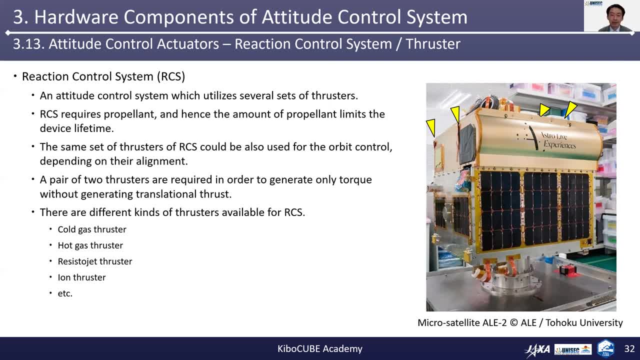 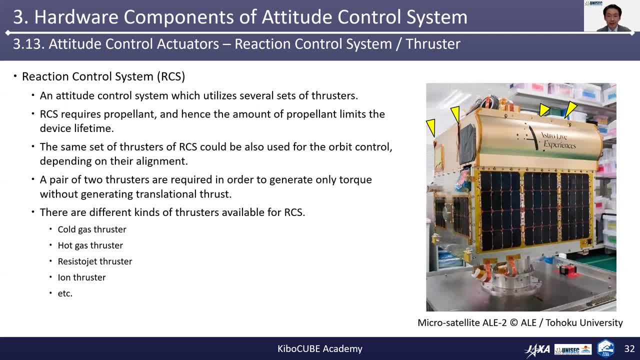 The same set of thrusters of RCS could also be used for controlling orbit. depending on their alignment. A pair of two thrusters are required in order to generate only torque without generating translational thrust. This picture is an example of microsatellite AL2,, which was implemented. 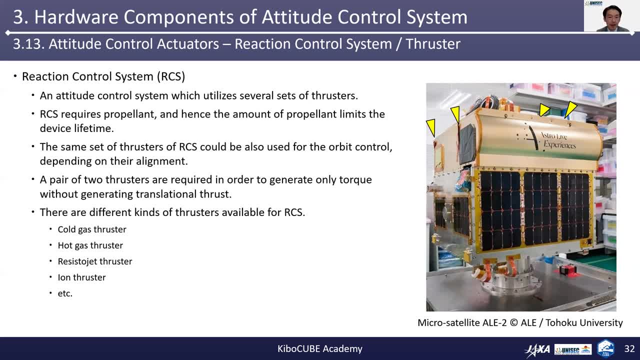 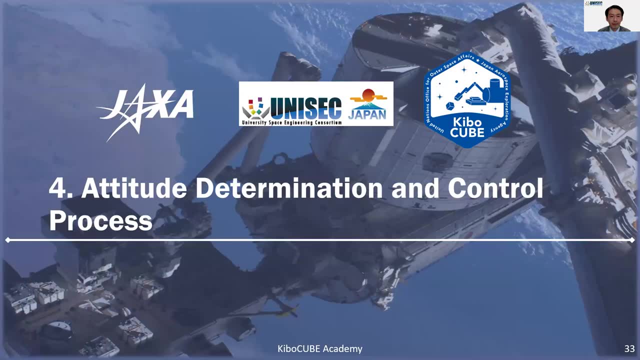 with four RCS thrusters. There are different kinds of thrusters available for RCS, such as cold gas thruster, hot gas thruster, resistojet thruster, ion thruster, etc. We will now move on to the next chapter, where I will explain the actual determination and 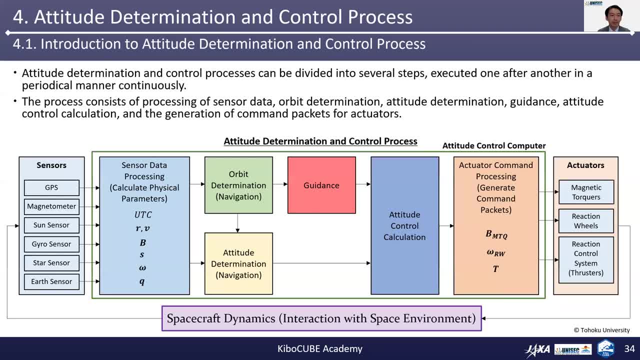 control process. The actual determination and control process can be divided into several steps which are executed one after another in a periodical manner, continuously. The process consists of processing sensor data, Orbit determination, actual determination guidance, actual control calculation and. 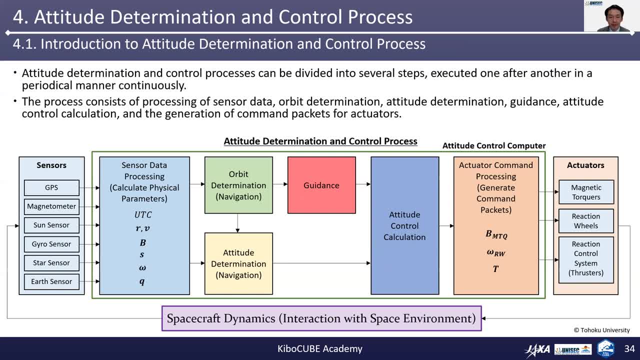 generation of actual control command packets sent to the actuator hardware. as illustrated in this figure, The outputs from the actuators change the satellite attitude by interacting with the space environment through satellite-actual dynamics. The sensors again measure the physical parameters of the updated situation in the 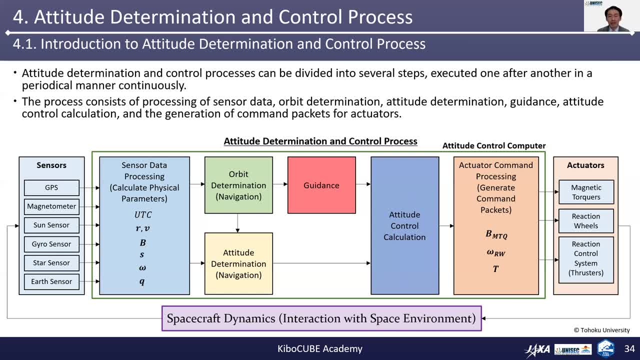 next time step. The orbit and attitude determination belong to the navigation process as discussed before, And for the calculation inside on-board computer. the environmental parameters need to be processed digitally. Processing of sensor data is required to convert the sensor output information to the digital variables. 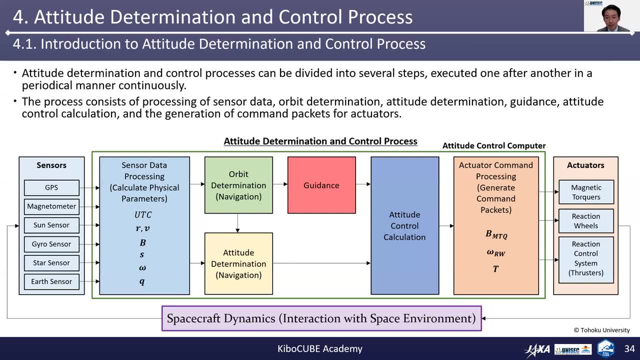 We can use products from our client's database in this body, such as PC4 or devsight, for example. The commands for the actuators need to be calculated out of the result of attitude control calculations inside onboard computer, So actuators have limitations in performance, such as maximum torque or the direction of. 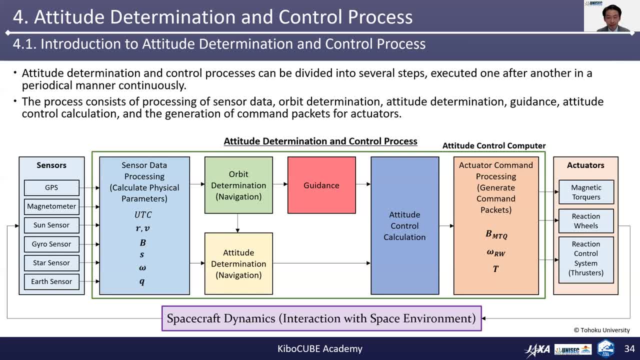 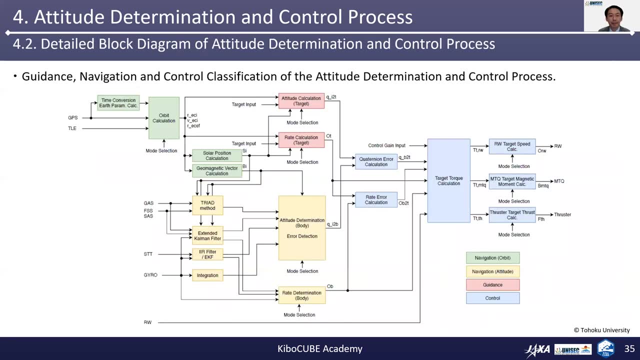 the torque, which can be generated. Terms a-i, wackia, comment, comment, comment, comment, comment and comments need to be generated in a meaningful manner in order to increase the efficiency of the driving electrical power or thruster propellant. 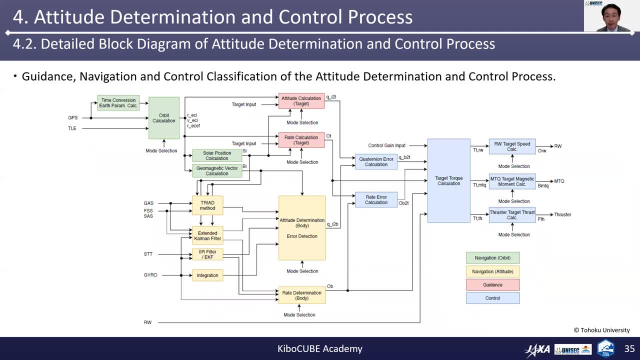 This diagram illustrates an example of a detailed attitude determination and control process over satellite. You can see that orbit calculation and attitude calculation are related to each other and they are classified into a navigation part, followed by a guidance part and control part, connected in this order. 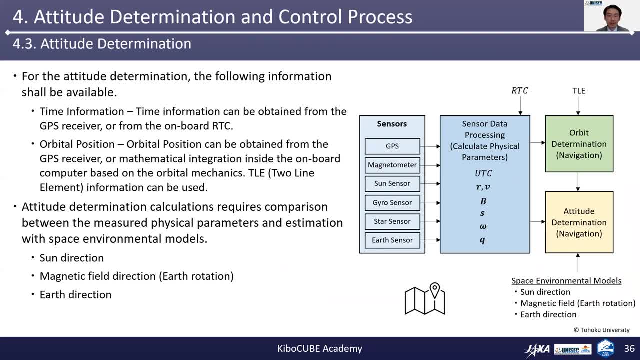 In the following slides I'd like to discuss each of the processing steps of the attitude determination and control. Our first topic is attitude determination. The following information shall be available for attitude determination: So Time information. Time information can be obtained from the GPS receiver or from the onboard real-time. 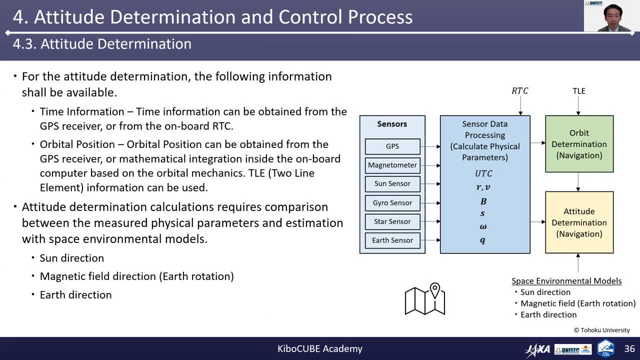 clock or RTC Orbital position. Orbital position can be obtained from the GPS receiver or mathematical integration inside onboard computer based on the orbital mechanics, TLE or two-line element information. This information can also be used for this purpose. 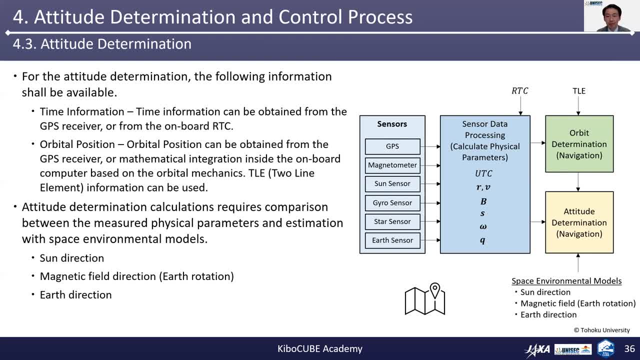 Attitude determination calculation requires comparison between the measured physical parameters and estimation with space environmental models such as sun direction, magnetic field direction, earth direction and so on. For the sensor data processing, the processing timing shall be determined by the measurement parameters or the measurement of the physical parameters and the measurement of the physical 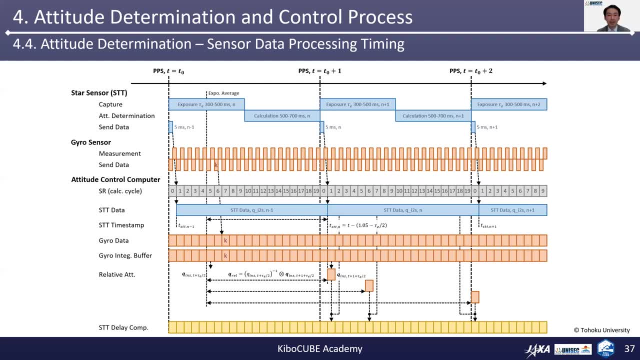 parameters For the sensor data processing. the processing timing shall be determined by the measurement parameters, So Time information timing shall be designed very carefully. This diagram is indicating an example of implementation of the processing timing of the actual determination, Usually sensor data output. 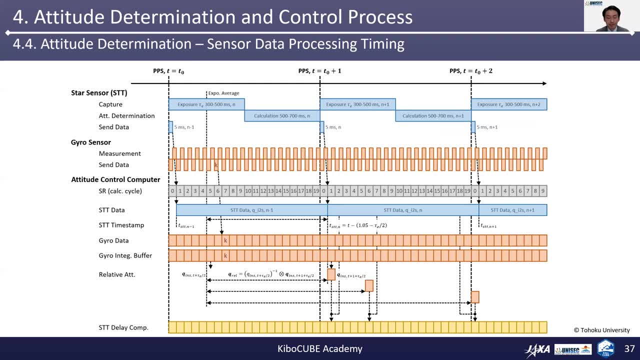 periods are depending on the devices. For example, a star tracker has lower output frequency than gyro sensors. Also, some outputs from sensors often correspond to situations of the past. For example, actual information output from star trackers are based on the time when the star images are acquired in the past. In those cases, we need to calculate a backwards. 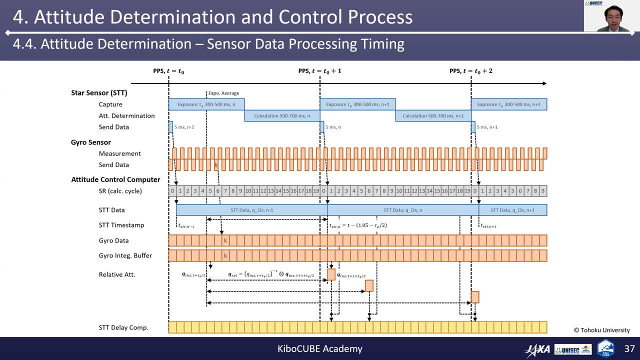 to determine the satellite at shoot at the time in the past and then we need to numerically integrate to get the current, updated actual information using the rotational velocity information stored in memory. this kind of back and forward calculation is necessary when you want to achieve a very high actual determination accuracy also it is very important. 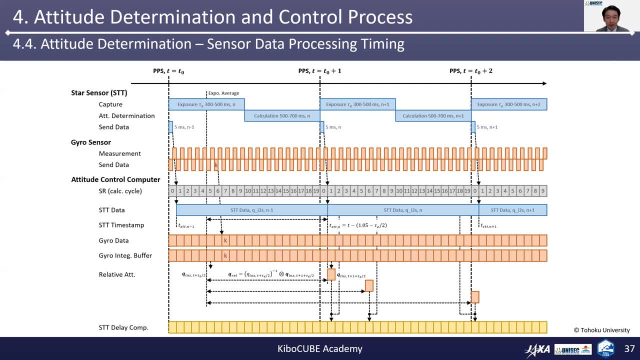 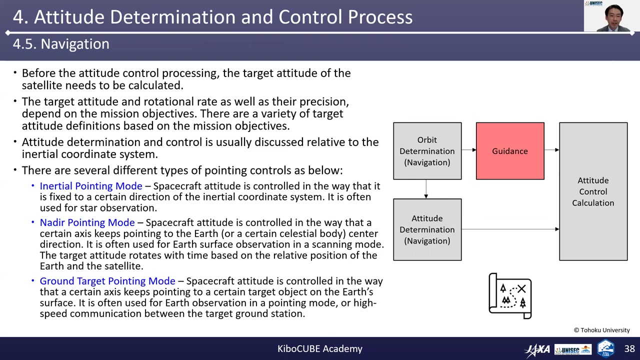 that the timing of these sensors outputs are carefully managed by the onboard computers. for this purpose, it is often the case that the pulse per second or pps signal output from gps receivers are distributed to the onboard peripheral sensor devices so that they can be synchronized with this signal. the next step is the guidance before the actual control processing the target. 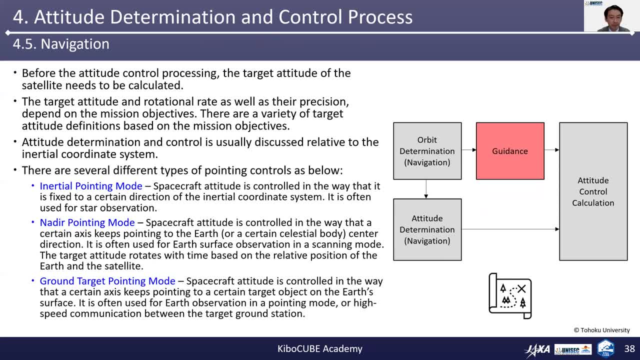 attitude of the satellite needs to be calculated. the target attitude and rotation rate and their precision depends on the mission objectives. there are a variety of target actual definitions based on the mission objectives, so actual determination and control is usually discussed. relative to the inertial coordinate system, there are several different types of pointing control as 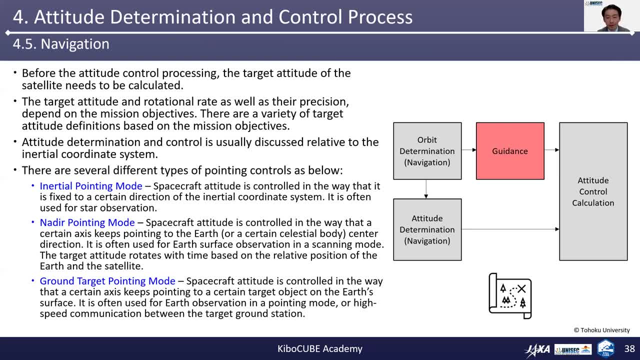 you can see in the video. so, inertial pointing mode: the spacecraft attitude is controlled in the way that it is fixed to a certain direction of the inertial coordinate system. it is often used for star observation. the nadia pointing mode: the spacecraft attitude is controlled in the way that a certain axis keeps. 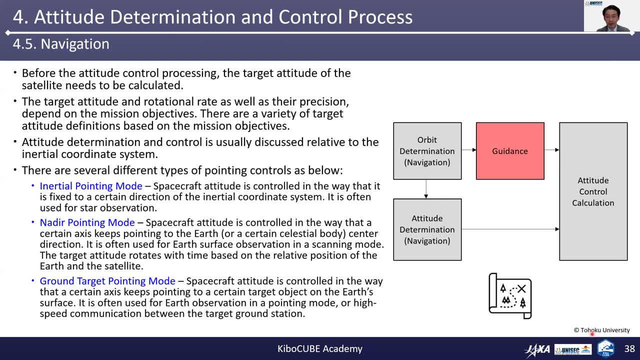 pointing to the earth or a certain celestial body's central direction. it is often used for earth surface observations. in a scanning mode, the target attitude rotate with time, based on the relative motion of the earth and the satellite. the ground target pointing mode. the spacecraft attitude is controlled in the way that a certain 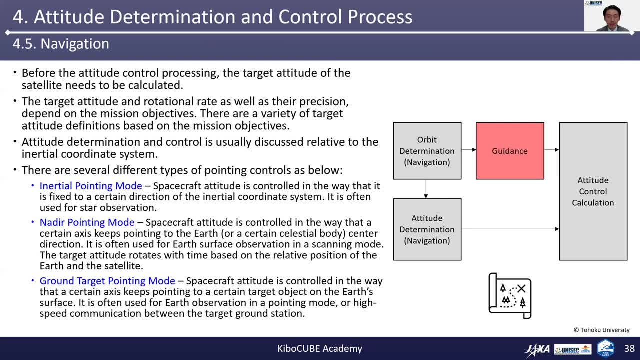 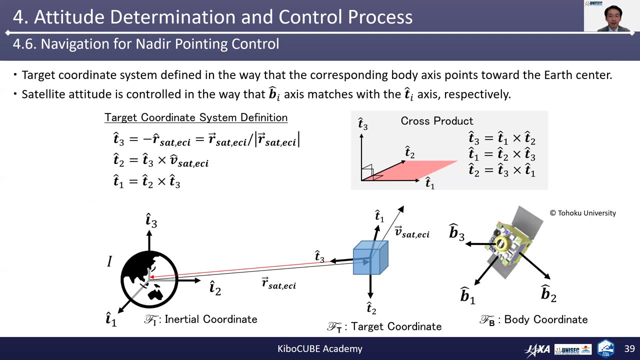 axis is touched keeps pointing to a certain target object on the Earth's surface. It is often used for Earth observation in a pointing mode or for high-speed communication between the satellite and target ground station. In the following two slides I'd like to show you two examples of navigation. 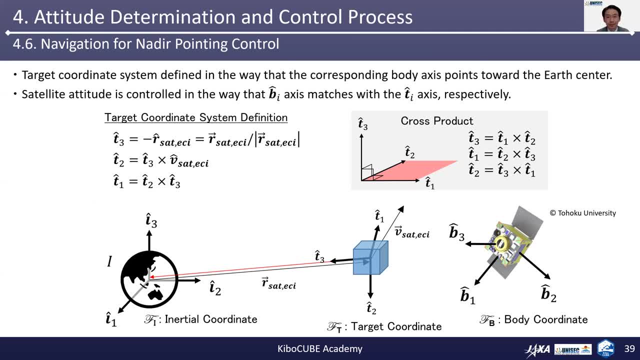 for different kinds of satellite attitude control. Our first example is the navigation for the Nadia Pointing Control. In this example, the target coordinate system is defined in the way that the corresponding body axis points toward the Earth's center. This is illustrated in this figure below. 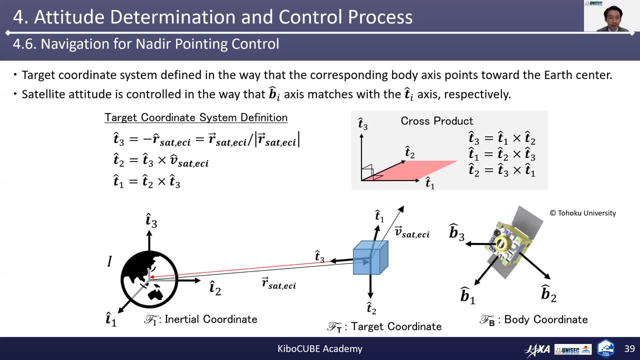 For this definition, the position vectors of the satellite are the SAT. and the position vectors of the satellite are the SAT. Relative to the Earth's center is used to determine the third axis of the target coordinate system first, which is indicated as T3.. 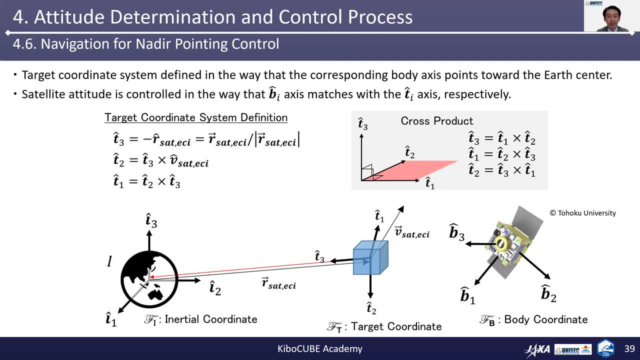 Then, in this example, the second vector, T2, is defined in the way that it's perpendicular to the orbital plane, And then the T1, is determined in the way that it is orthogonal to both of these two vectors. The body coordinate system is controlled in the way that: 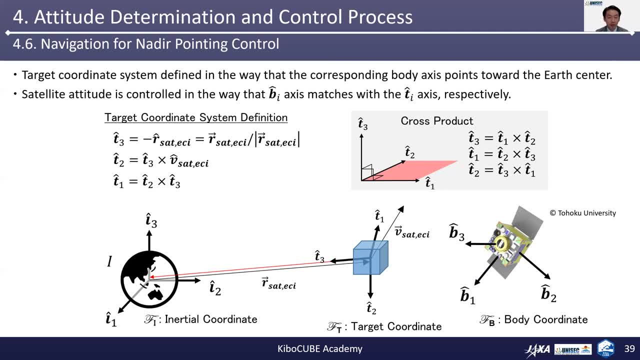 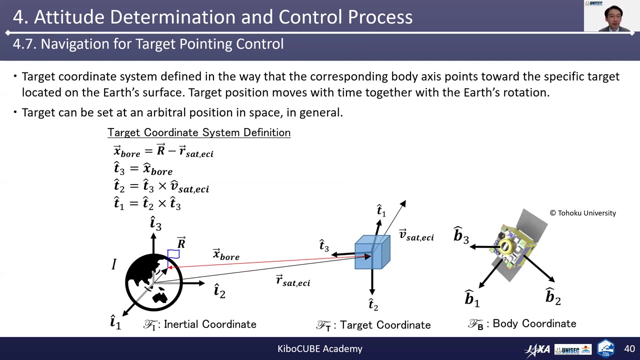 it overlaps with the defined target coordinate to achieve the pointing of these sensor instruments toward the Earth's center, As illustrated in this figure. for this calculation we often use cross products of vectors. The second example is the navigation for the target pointing control. 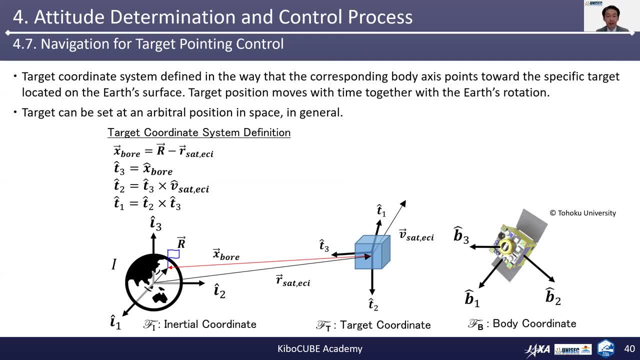 The target coordinate system is defined in the way that the corresponding body axis points toward the specific target located on the Earth's surface. In this example, the target position moves with the time, together with the Earth's rotation. As indicated in this example, the target can be set at an arbitrary position in space. in general, 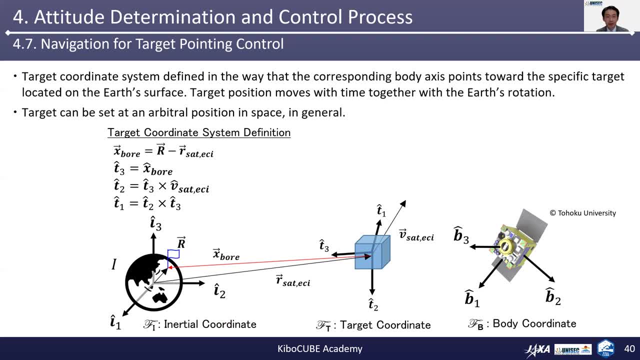 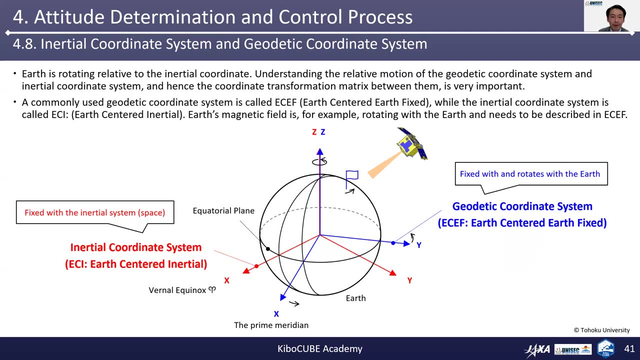 This kind of reference coordinate system can be designed using available vector information, such as the position vector of the spacecraft, velocity vector, position vector of the target position and so on. For the actual determination and control purpose, we need to understand the relationship between the inertial coordinate system. 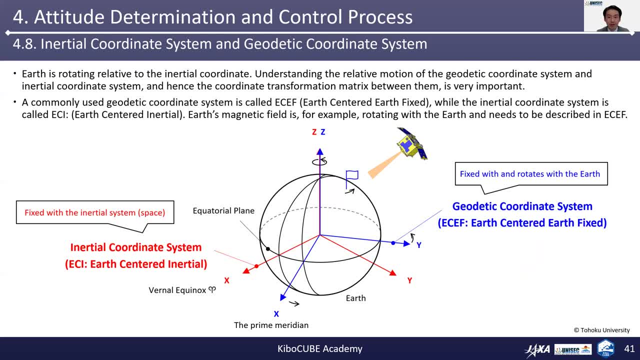 and the geodetic coordinate system. as the Earth is rotating relative to the inertial frame, as illustrated in the figure below. The inertial coordinate system, or often called the Earth-centered inertial coordinate system, is indicated in red, which is fixed with space. 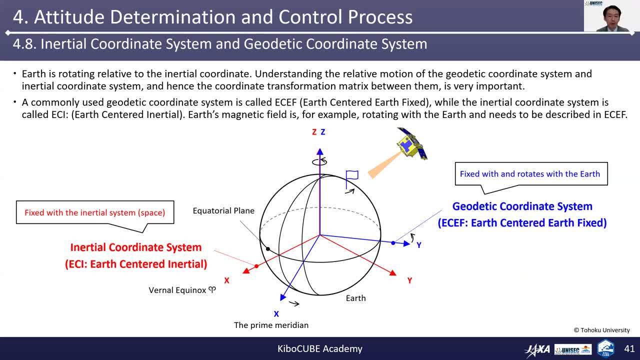 The geodetic coordinate system, which is often called ECEF- Earth-centered, Earth-fixed system- is indicated in blue, which is fixed with the Earth and rotates together with the Earth. For example, longitude and latitude information is defined relative to the ECEF coordinate system. 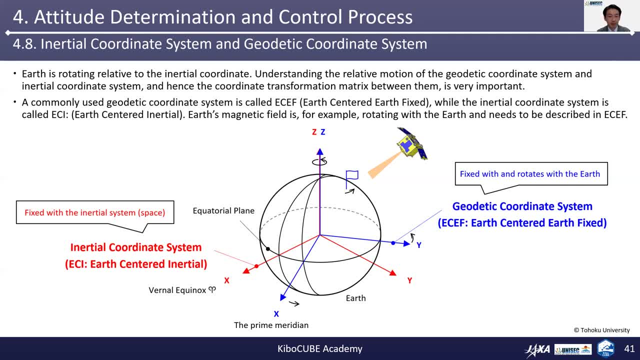 The Earth's magnetic field is rotating with the Earth and needs to be described in ECEF as well. On the contrary, the direction of the Sun, Moon and so on are described against the ECI system. generally speaking, Understanding the relative motion of the geodetic coordinate system, 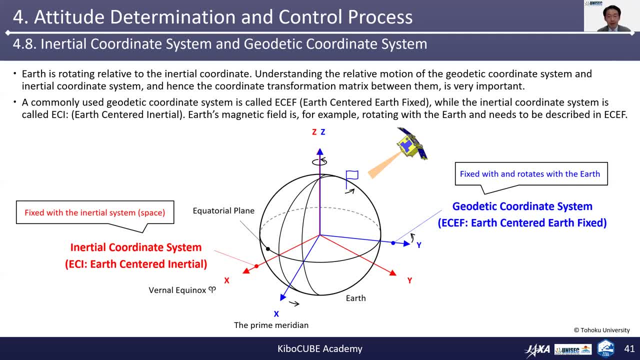 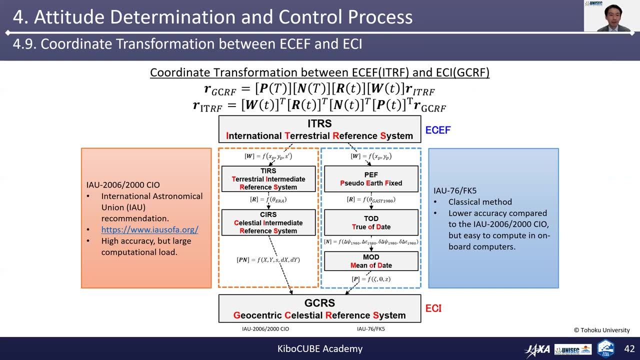 and the inertial coordinate system, and hence the coordinate transformation matrix between them is very important. This slide illustrates the coordination transformation between the ECEF and the ECI. Earth's rotation actually consists of several different motions, such as rotation mutation. 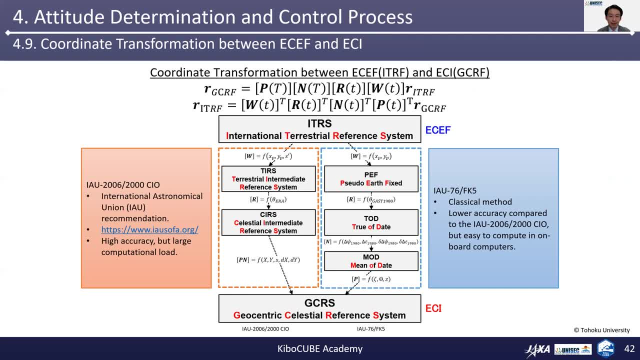 and precision. All of these effects need to be taken into account for a precise coordinate transformation between the ECEF and the ECI. For example, a GPS receiver usually delivers position in an ECEF coordinate and then you need to transform that information back to the ECI coordinate. 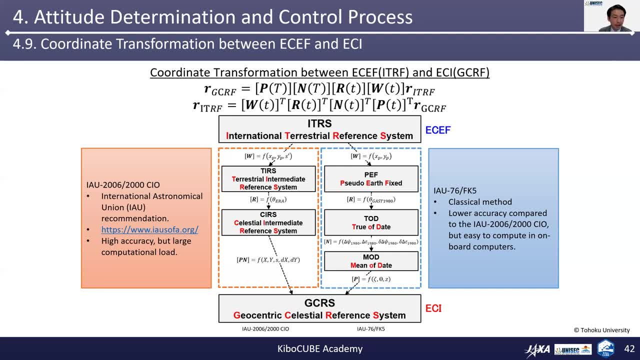 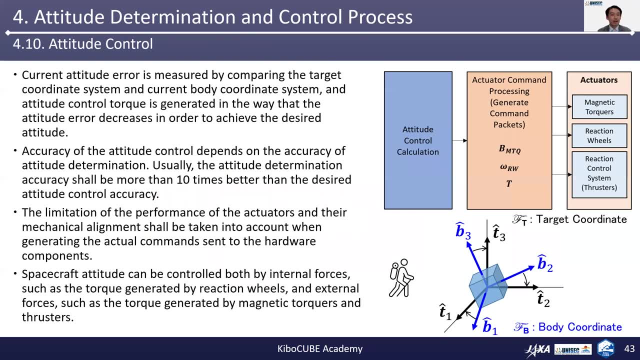 in order to determine the position of the ECEF. This is the last slide of this chapter. The last step is the attitude control. The current attitude error is measured by comparing the target coordinate system and the current body coordinate system. An attitude control torque is generated. 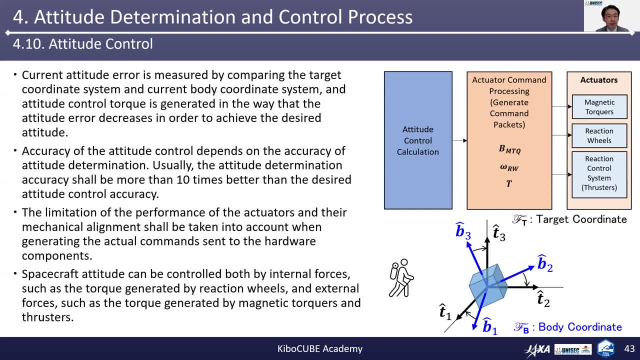 in the way that the actual error decreases in order to achieve the desired attitude. Accuracy of the attitude control depends on the accuracy of the attitude determination. Usually, the attitude determination accuracy shall be more than 10 times better than the desired attitude control accuracy. 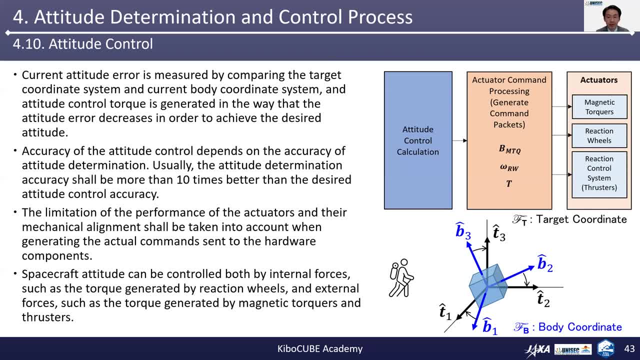 The limitation of the performance of the actuators and their mechanical alignment and orientation shall be taken into account when generating the actual commands sent to the hardware components. Spacecraft attitude can be controlled both by internal forces, such as torque, generated by reaction wheels, and external forces such as torque. 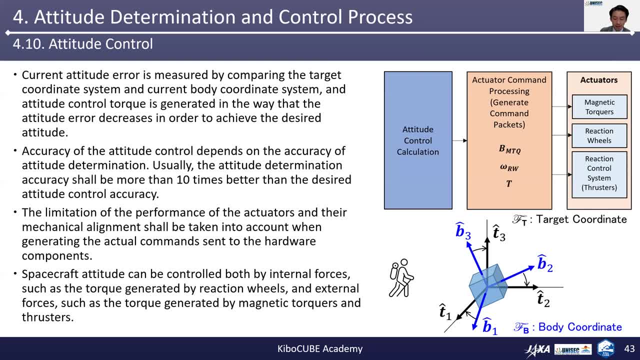 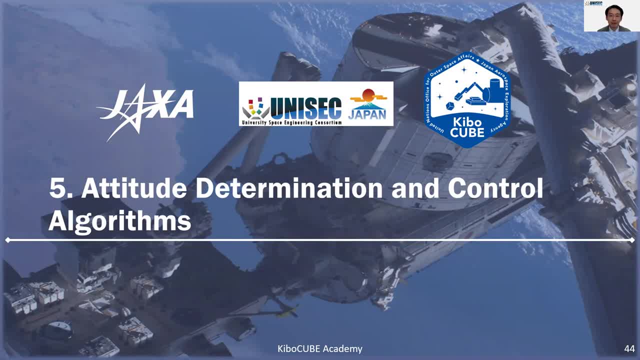 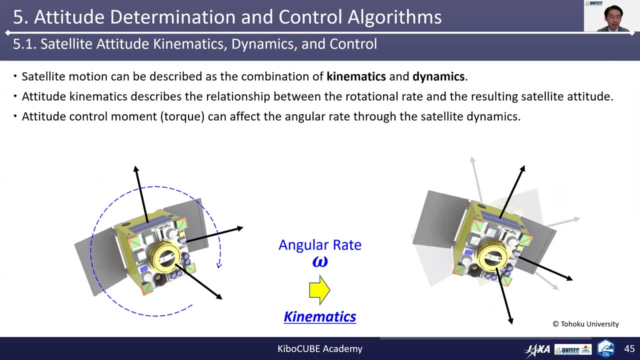 generated by magnetic torquers and thrusters. Now let's take a close look at the attitude determination and control algorithms from the mathematical point of view in this next chapter. Satellite motion can be described as the combination of kinematics and dynamics. Attitude kinematics describes the relationship. 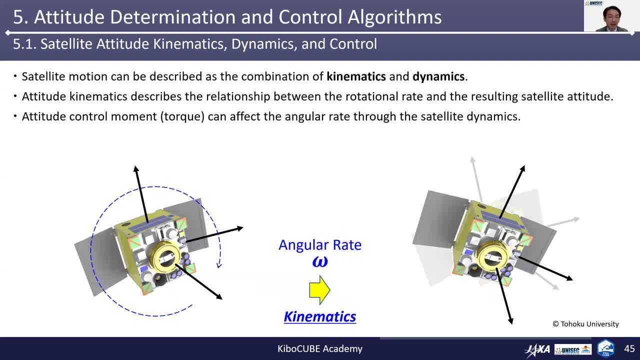 between the rotational rate and the resulting satellite attitude. Therefore, measuring the attitude angular velocity is necessary in order to numerically propagate the satellite attitude. This is illustrated in this figure. In addition to this, an actual control moment or torque acting on the satellite. 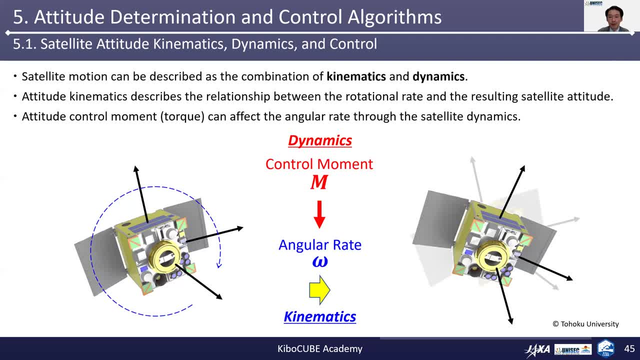 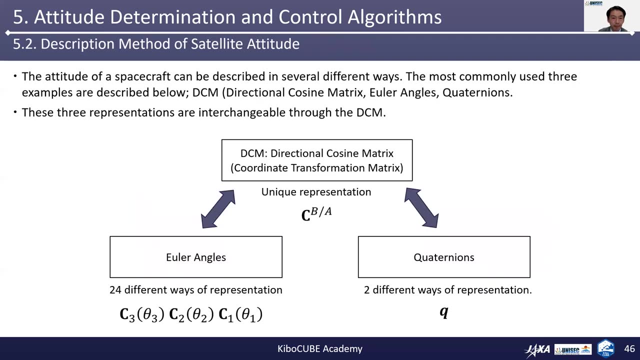 can affect the angular rate through the satellite dynamics. As a result, the satellite attitude can be integrated with the updated angular velocity information for the next time step. The attitude of spacecraft can be described in several different ways. The most commonly used three examples are described below. 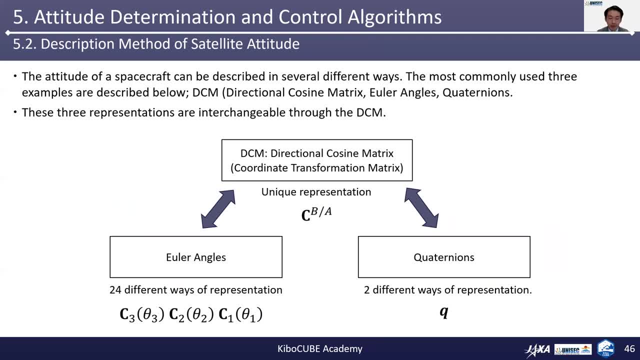 BCN, the directional cosine matrix, Euler angles and quaternions. As illustrated in this diagram, these mathematical descriptions represent the actual description method respectively. While there is only one way of representing the DCM, there are multiple ways of description. 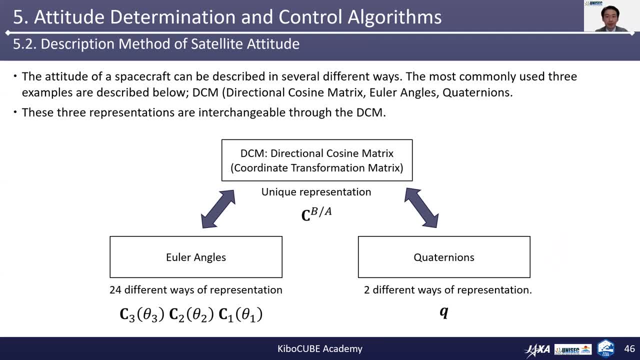 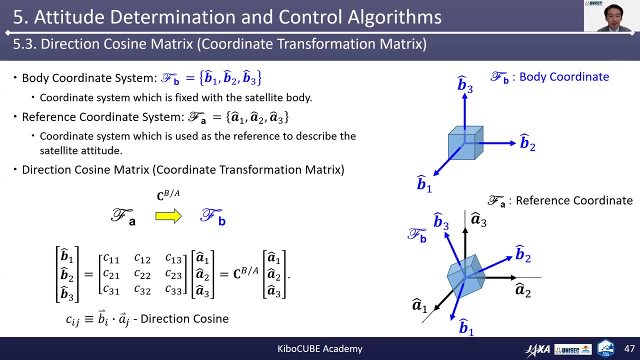 variations available for the other types of description methods. These three representations are interchangeable. In the following slides, I'd like to explain each of these description methods briefly. Let's start from the direction cosine matrix or DCM, which is also called a coordinate transformation matrix. 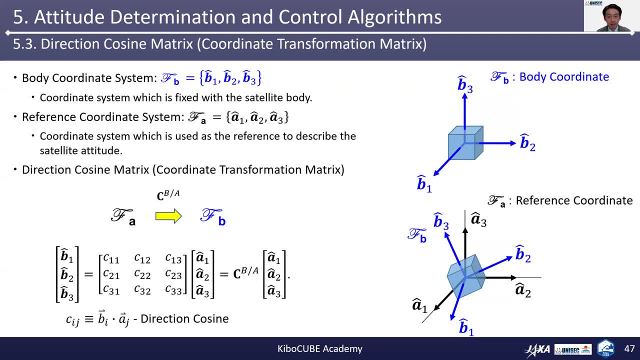 We start from the definition of a body coordinate system, which is indicated by FB, system B, and also the reference coordinate system indicated by FA, here, system A, as illustrated on the right. So here the body coordinate system is a system. 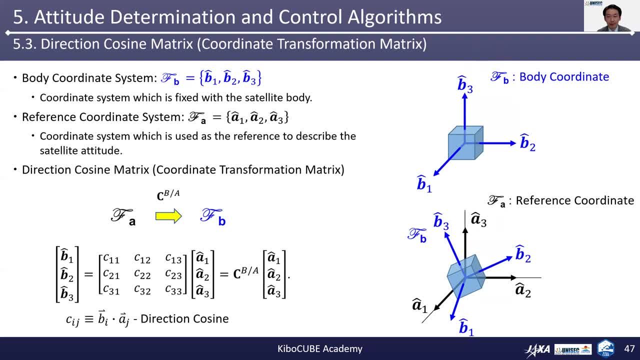 which is fixed with the satellite body. The direction cosine matrix can be described in the form of a 3x3 matrix as described below. In this equation, each element of this matrix is called a direction cosine between the components of each coordinate system's. 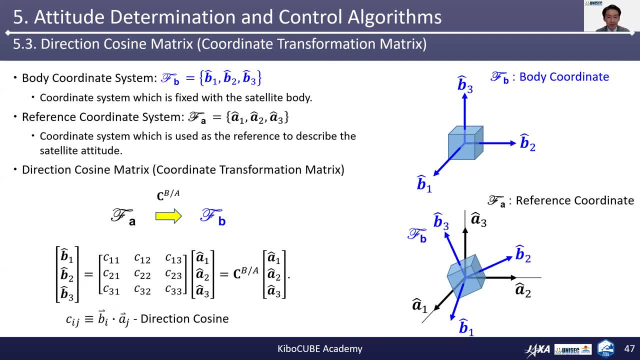 basis vectors, And therefore this matrix is called a direction cosine matrix. This is also known as a coordinate transformation matrix. Information in the reference coordinate system can be transformed to the body coordinate system, or vice versa, using this coordinate transformation matrix. This is indicated here. 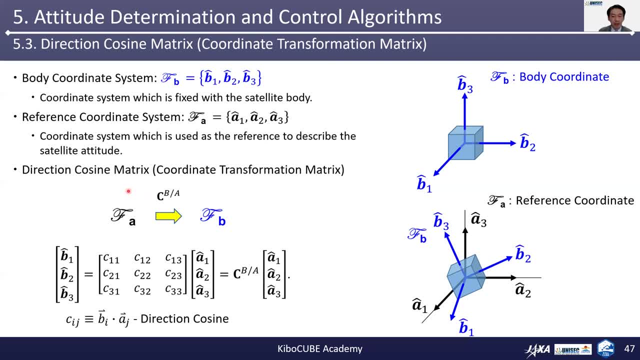 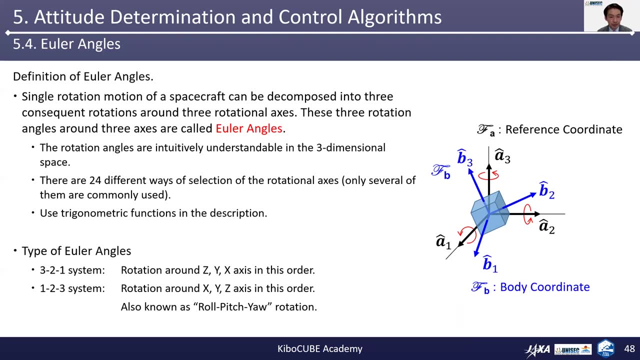 in the form of C, B over A, indicating that this is a coordinate transformation matrix from the system A to system B. The next one is the Euler angles. Single rotation motion of a spacecraft can be decomposed into three consequent rotations around three rotational axes. 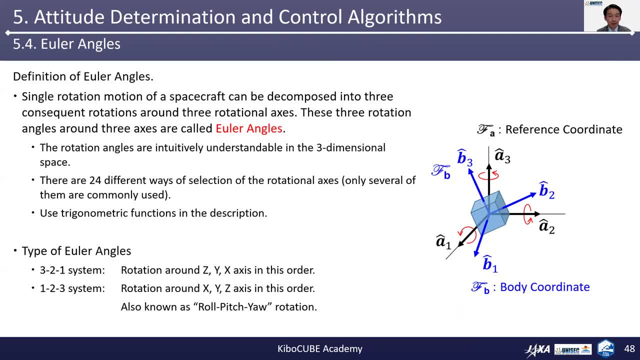 These three rotational angles around three axes are called Euler angles. The rotation angles are intuitively understandable in three-dimensional space. There are 24 different ways of selecting the rotational axes and there are several commonly used ones, among them An Euler angles calculation uses trigonometric functions. 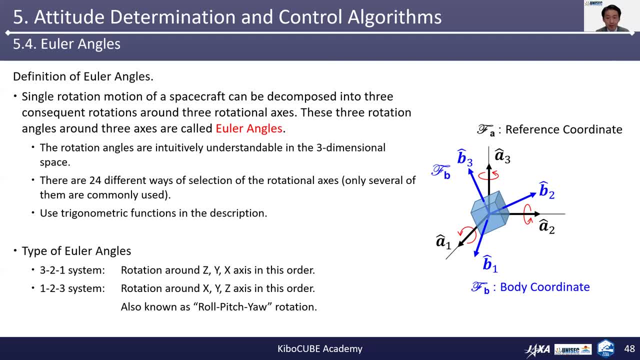 Some of the commonly used sets of Euler angles are listed below. The 3-2-1 system is a rotation around the Z, Y and X axes in this order, and the 1-2-3 system is a rotation around the X, Y and Z axes. 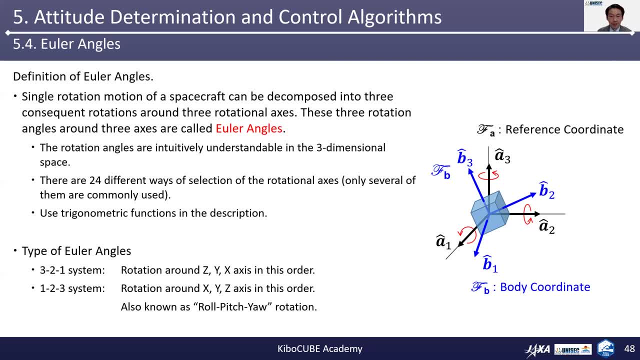 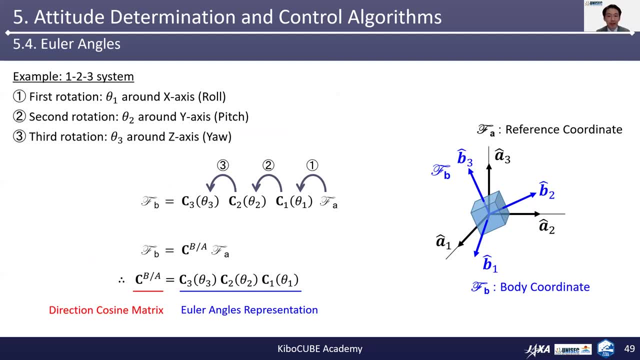 in this order, which is also known as roll pitch yaw rotation. Let's take a look at the example of Euler angles in the 1-2-3 system. So in this definition, the first rotation is around the first axis. 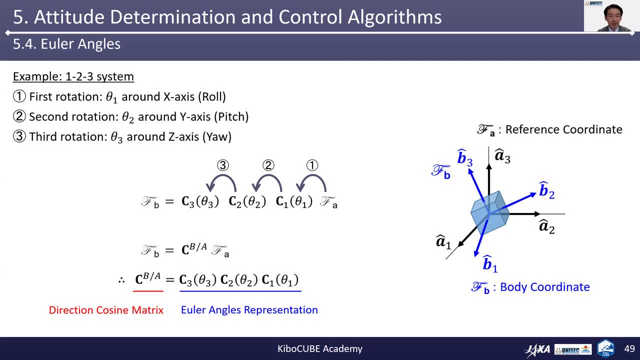 which is the X axis for the angle of theta1.. This is also called a roll angle. The second rotation is about the Y axis for the angle of theta2, which is called a pitch angle, And then the third rotation is around the Z axis. 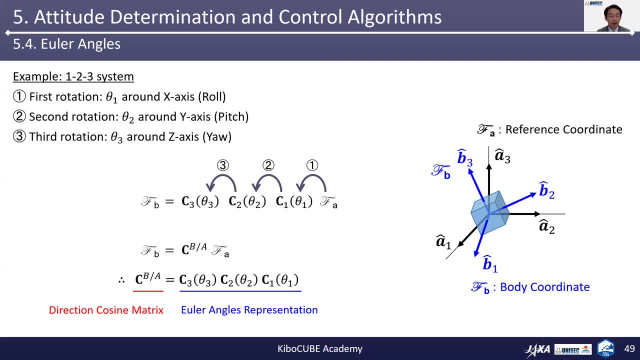 for the angle of theta3, which is called a yaw angle, The rotational order is around the X, Y, Z axes, or 1,, 2,, 3 axes. The rotational matrix to be multiplied to system A can be described in this way: 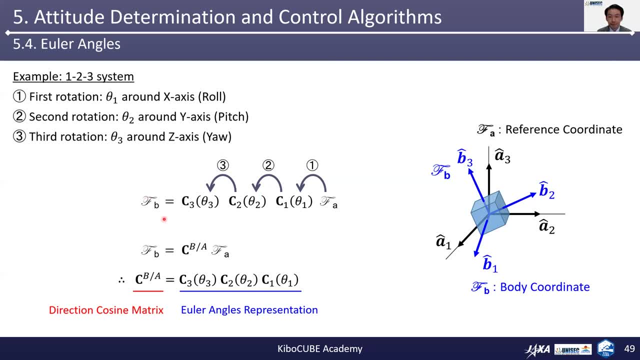 as described in this equation, The first rotation to be multiplied is located in the rightmost position- theta1.. And then the second rotation comes to the next position, which is C2, theta2.. The third rotation is located at the leftmost position. 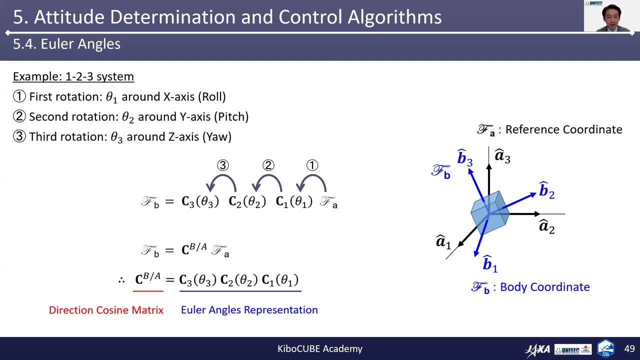 of this multiplication, such as C3, theta3, in this mathematical equation, You can also remember that the coordinate transformation between system A to system B can be indicated by C, B over A, as discussed in the previous slides. So if you compare these two equations, 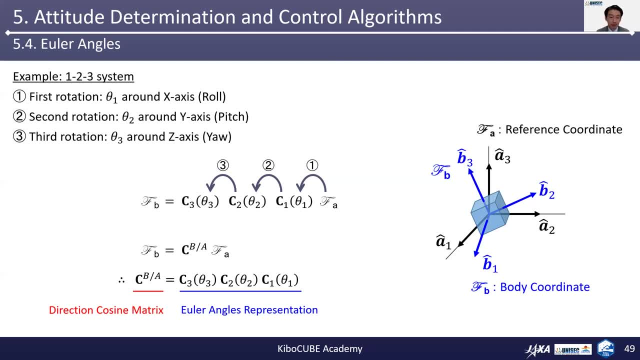 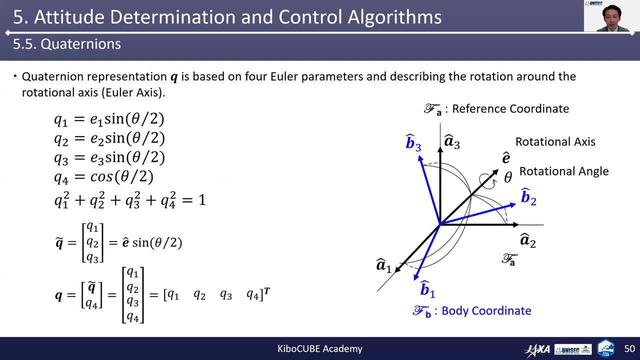 you can also extract the relationship between the direction, cosine matrix and Euler angles representation, which is in this case in the 1,, 2, 3 system, as described here. The third example is the quaternions. The quaternion represented by Q is based on four Euler parameters. 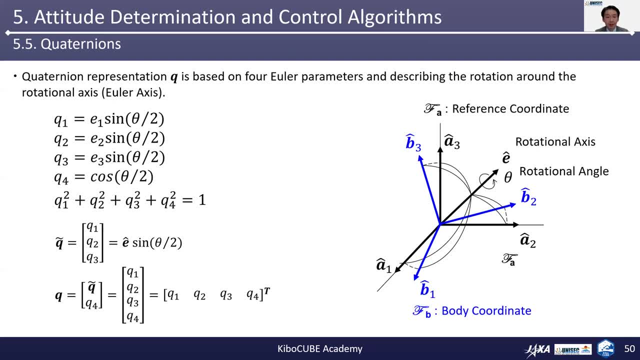 which is indicating the rotation around the rotational axis, also known as Euler axis. In the figure on the right I have illustrated the relationship between the reference coordinate and body coordinate systems: Euler axis of rotation and rotation angle. theta around the Euler axis: Any displacement. 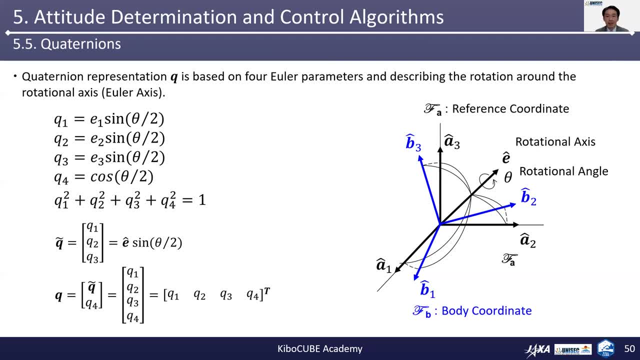 of the satellite attitude can be described as a single rotation around the specific axis or specific angle, as indicated in this figure. These Q1 to Q4 parameters are the so-called Euler parameters. If you take the summation of these terms, it becomes one. 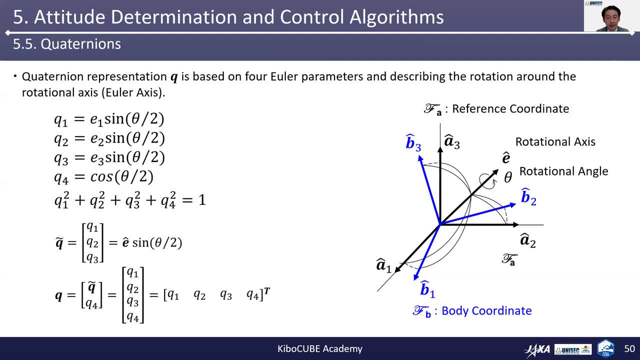 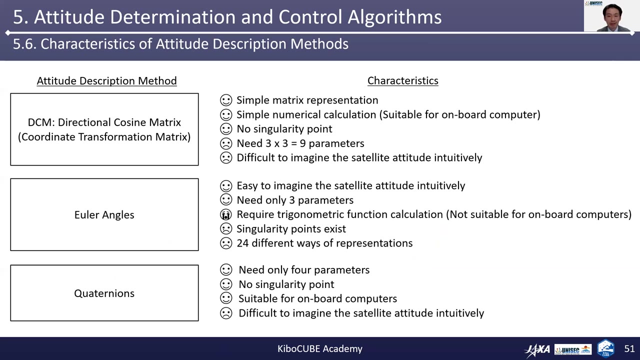 So quaternion Q is then described in the vector form using these four parameters. Quaternion doesn't have a singularity problem and is a very useful description used for satellite attitude representation. In this slide I have summarized the characteristics of each attitude description method. The first one, 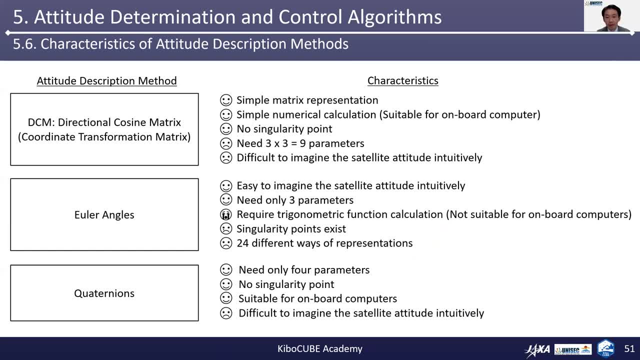 is the direction cosine matrix or DCM, also known as coordinate transformation matrix. As we saw in the previous slides, DCM is a simple representation with a 3x3 matrix. We need only simple numerical calculations, which is suitable for onboard computers. 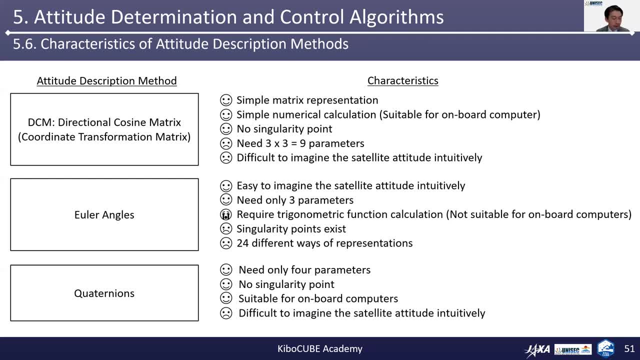 and it has no singularity point. Some drawback using DCM is that it has a 3x3 and in total nine parameters, which makes it difficult to imagine the spacecraft attitude intuitively and instantaneously. Next is the Euler angles. Euler angles. 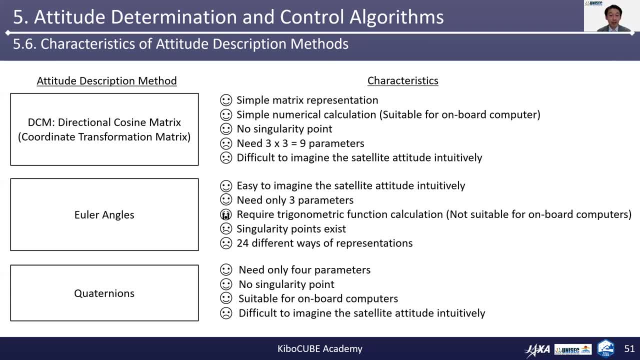 make intuitively understanding the satellite attitude easy, And it also needs only three parameters. These are the merits using Euler angles. However, calculating Euler angles requires trigonometric function calculations, which is not suitable for onboard computers, And also Euler angle definitions. 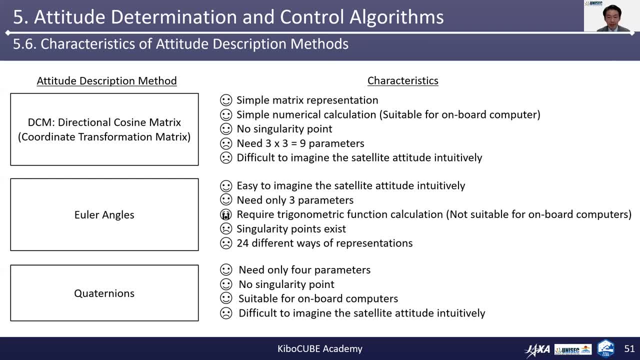 have singularity points. Furthermore, there are 24 different ways of representing Euler angles. The third one is quaternions. So quaternions need only four parameters and it has no singularity points. These features make it suitable for onboard computers, as they are less trigonometric functions. 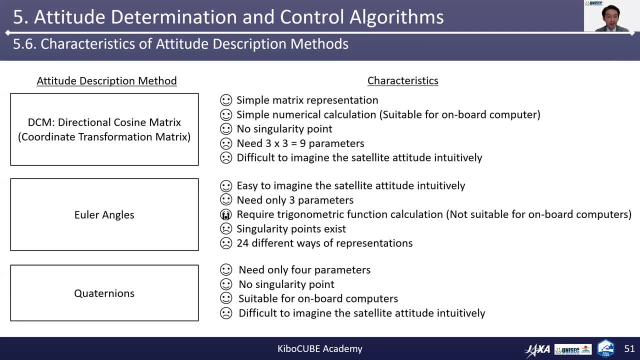 But it is still difficult to imagine the satellite attitude intuitively. According to these characteristics, quaternions are usually widely used for the satellite attitude representation, And then directional cosine matrix and Euler angles are used to reproduce necessary information for the understanding of the satellite operator. 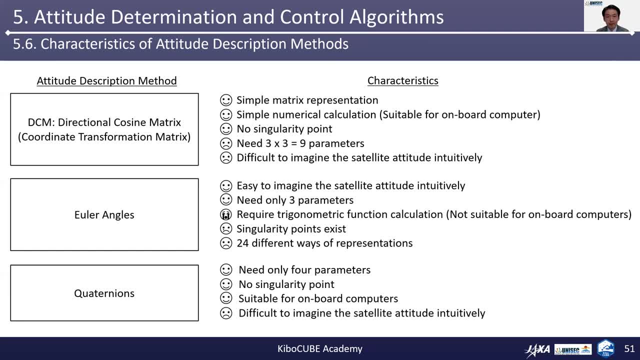 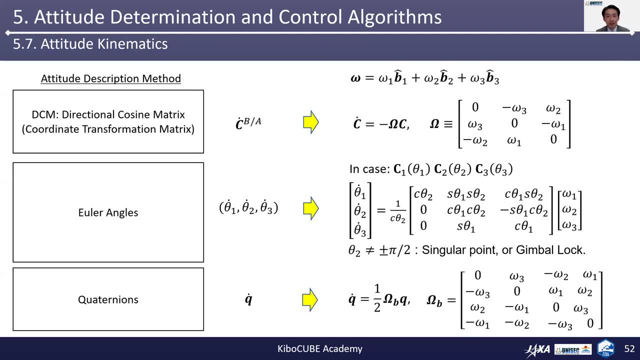 or for specific attitude control purposes. When you have learned about the attitude description method, the next step is to understand the attitude kinematics. Attitude kinematics is the relationship between the angular rotational velocity and the time derivative of the attitude description method In this slide. 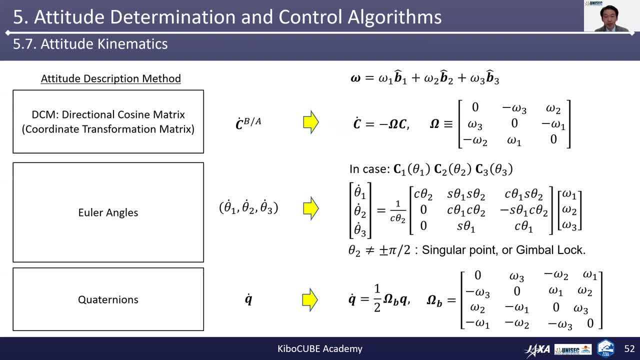 I have listed up three different descriptions of the attitude kinematics corresponding to the previously mentioned three different ways of attitude representation methods. The first one is the directional cosine matrix. If the angular rotational velocity, omega, is provided, the time derivative of the direction cosine matrix. 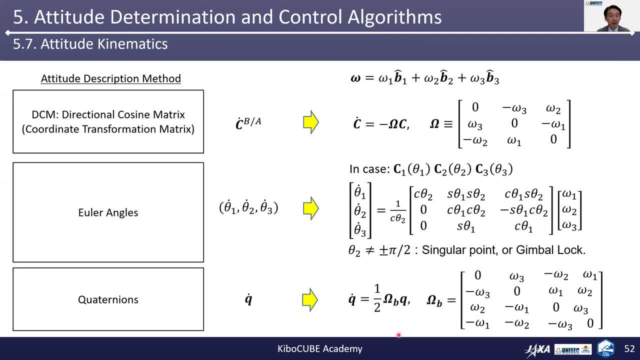 can be obtained using this equation on the right-hand side. In a similar way, the time derivative of Euler angles and quaternions can be obtained using the equations described below, As described here, depending on which description method you are using: the time derivatives. 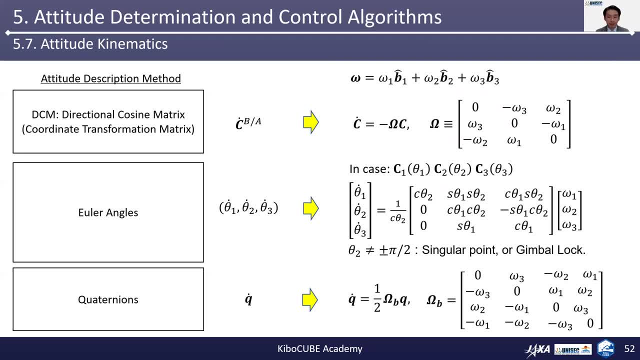 can be obtained from these equations, And by knowing these values, you can numerically integrate and propagate the satellite attitude in each time step. Therefore, it is now clear that measuring accurate satellite angular velocity is very important to determining the satellite attitude. So torque-free. 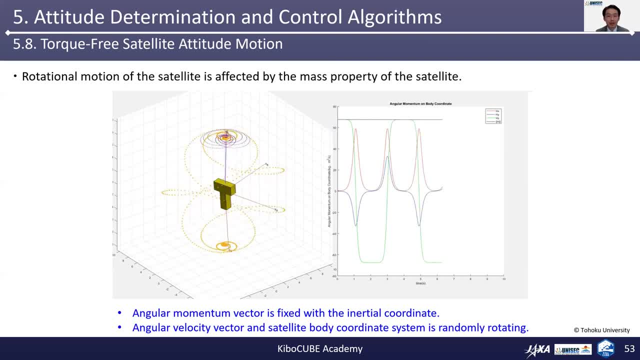 satellite attitude motion can be calculated based on the knowledge about attitude descriptions and satellite attitude kinematics explained in the previous slides. This slide shows a simulated result of actual rotational motion of a satellite as an example. In this example, a T-shaped satellite with such a mass distribution. 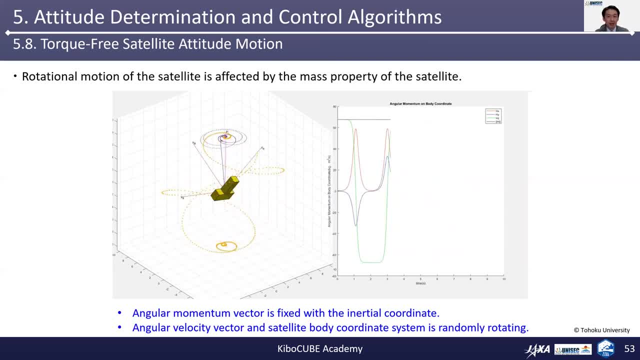 is analyzed, You can see that the satellite attitude can be calculated based on the kinematics equations, assuming that the angular velocity can be measured by a gyro sensor which is attached to the satellite body. It is therefore important to know that the measured value of the angular velocity 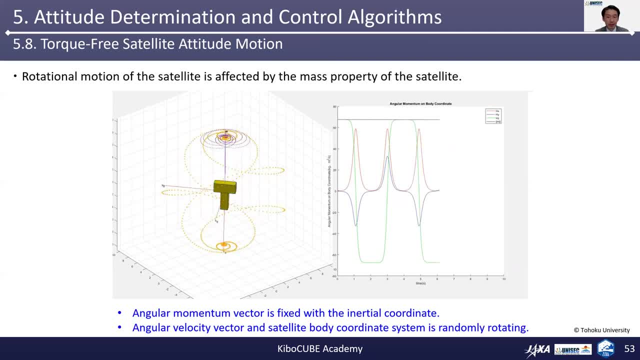 is in respect to the body-fixed coordinate system. In this animation it is shown that the angular momentum vector is fixed with the inertial coordinate system and the angular velocity vector and the satellite body coordinate system appear randomly rotating. So in this next example animation, 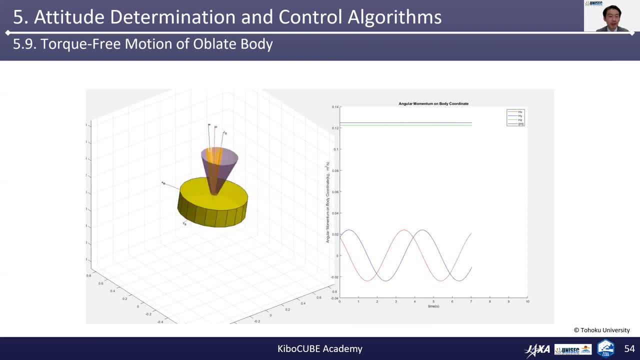 you can see the torque-free rotational motion of a satellite with an oblate shape. Many satellites in the past had a cylindrical shape and then their actual motion was something like this. You can see that the yellow cone, which is called a space cone- 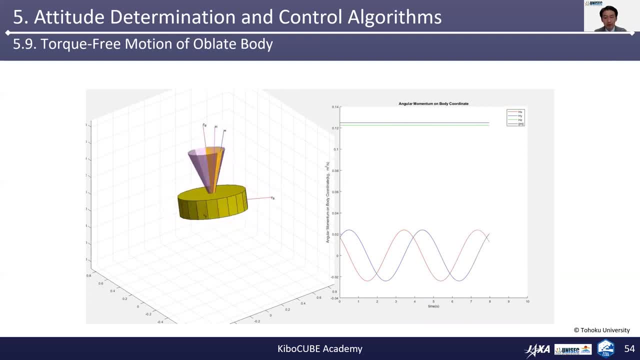 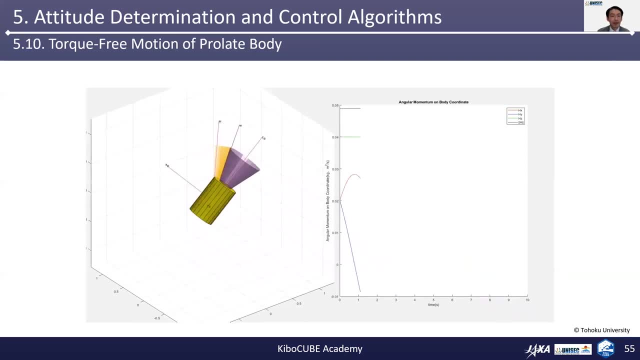 is inside the purple cone, which is called a body cone in this example. In this slide you can see the torque-free motion of a satellite with a fluoride shape. If the satellite body has a long cylindrical shape and mass distribution, the rotational motion. 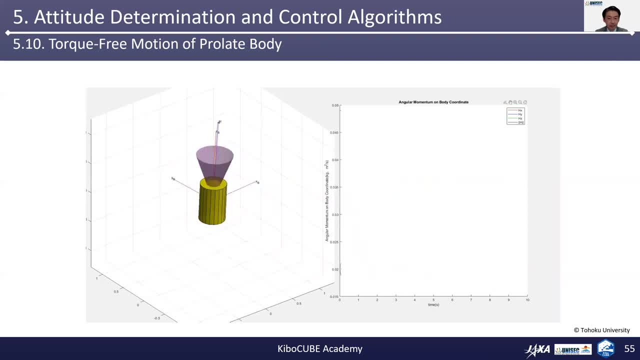 of the spacecraft becomes something like this: So you can see that the yellow and the purple cones are now touching on the outside surface with each other. So you can compare these two motions in terms of the relative relationship between the body coordinate axis. angular velocity vector. 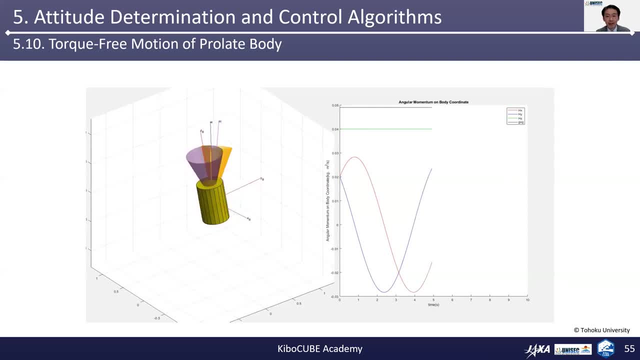 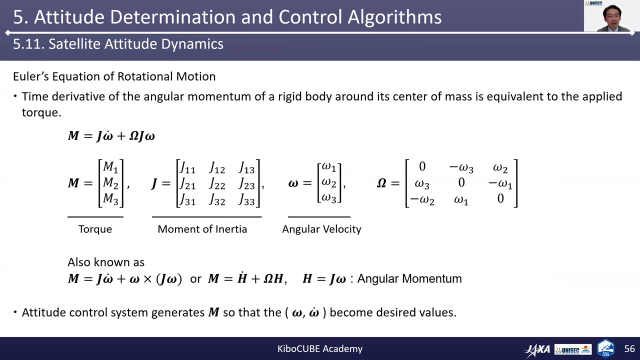 and angular momentum vector. It is indicated that it is important to examine the shape of the satellite and the corresponding mass distribution carefully, because it influences the torque-free satellite attitude. rotational motion characteristics: The next topic we need to understand about the rotational motion of a satellite. 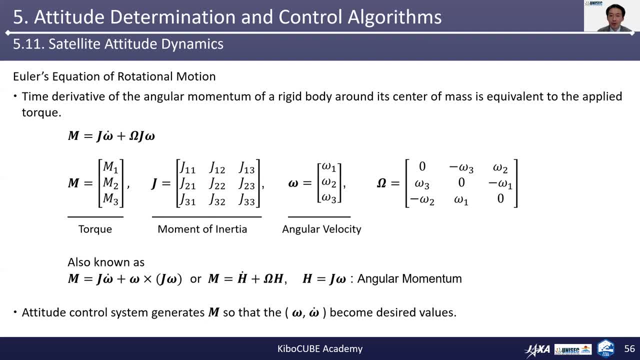 is the satellite attitude dynamics, which means that we need to understand the change in satellite attitude when torque is acting on the satellite, As described in this slide below. the rotational motion of a satellite can be described by the so-called Euler's equation of rotational motion. 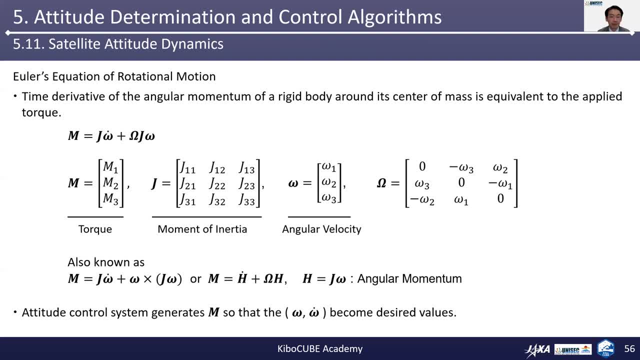 This equation is describing that the time derivative of the angular momentum of a rigid body around its center of mass is equivalent to the applied torque to the system. Here m is the torque acting on the satellite, j is the moment of inertia, which is representing 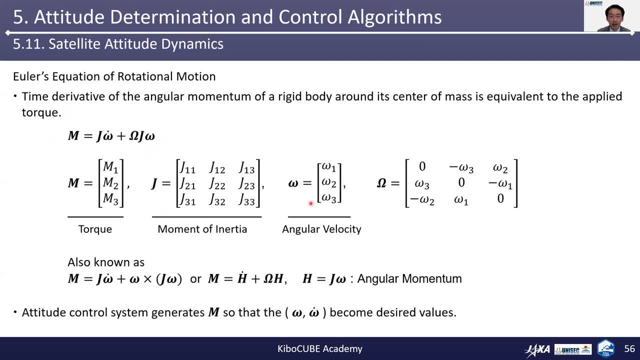 the satellite's mass distribution, and omega is the angular velocity. Also, this large omega is the so-called skew symmetric matrix. Euler's equation of rotational motion can also be described in other forms, as listed below. Here, the h is representing the angular momentum. 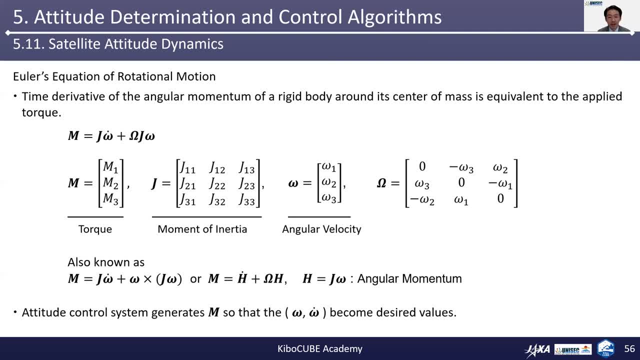 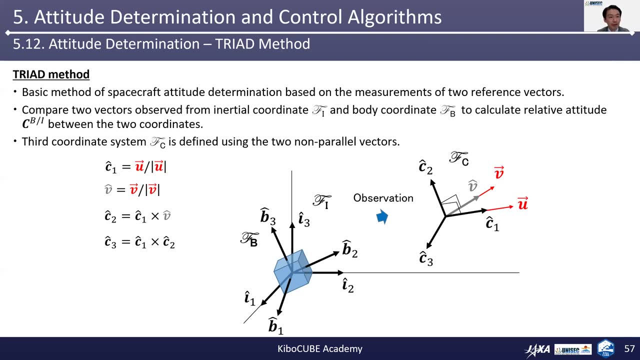 of the satellite. An actual control system shall generate the controlling torque m so that omega and its time derivative can approach the desired values. As we now understand the rotational motion of the satellite, we'd like to discuss actual determination and control in the following slides. 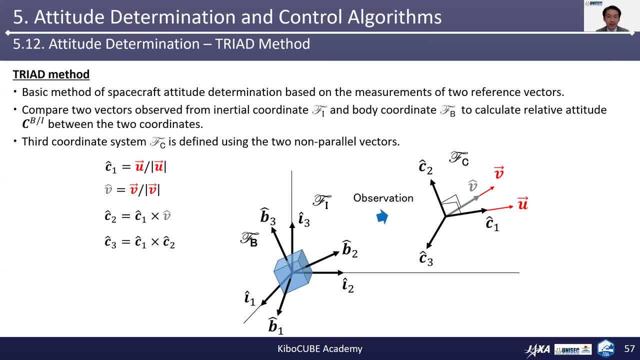 First of all, as an example of satellite actual determination methods, I'd like to introduce the triad method. The triad method is a basic method of actual determination based on the measurements of two non-parallel reference vectors By comparing observations of these vectors. 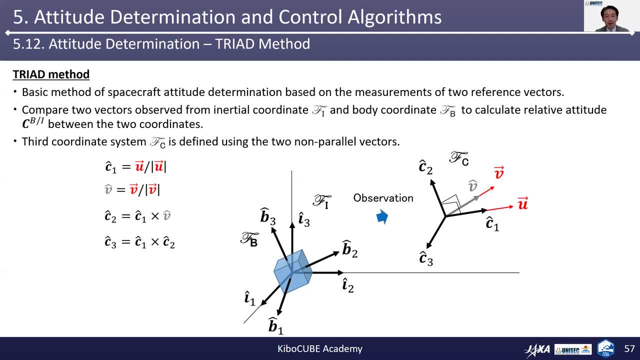 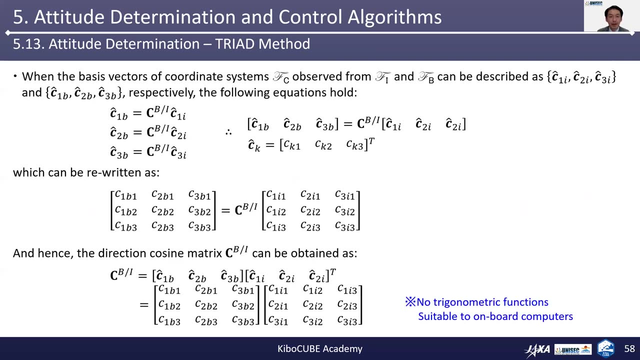 from inertial coordinates and body coordinates. an intermediate coordinate c can be defined, as illustrated in this figure below using these equations: By means of this intermediate coordinate c, the relationship between the observation in the inertial coordinate system and observation in the body coordinate system. 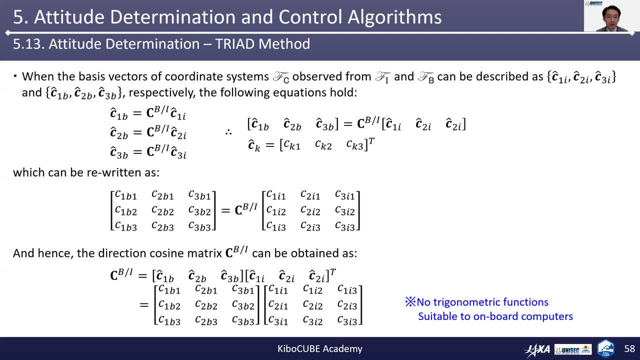 can be related with the coordinate transformation matrix between the two coordinate systems, as described in these equations above. From this equation, the coordinate transformation matrix can be calculated by matrix multiplication, as described in the equation below. Please note that the first matrix is based on the actual observation. 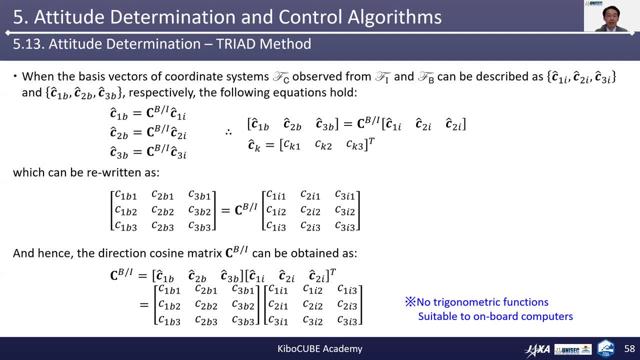 of the reference vectors using onboard sensors, and the second matrix is based on the theoretical values which can be calculated from physical models of the vectors in the onboard computer, such as the magnetic field vector and sound vector models. Also, it is a great advantage. 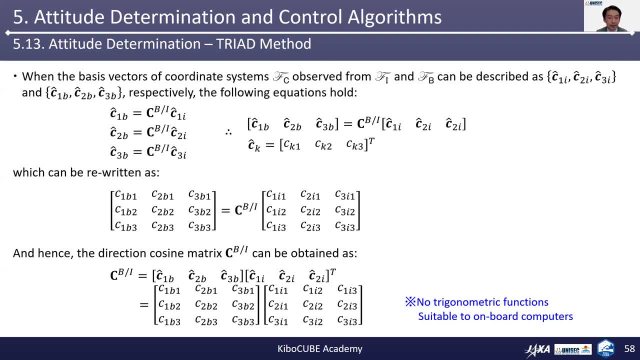 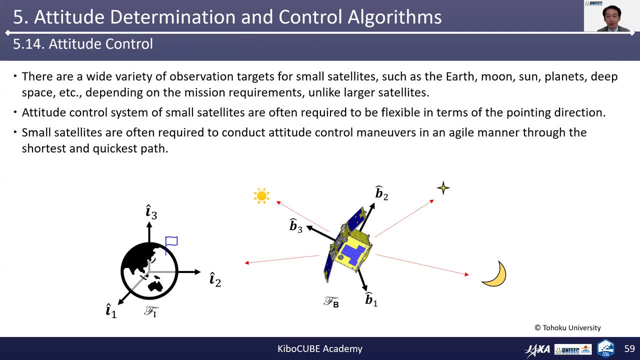 of this method that it doesn't include trigonometric functions, which makes it suitable for implementation in onboard computers. After the determination of the satellite attitude, we can start attitude control of the satellite. There are a wide variety of observation targets for small satellites. 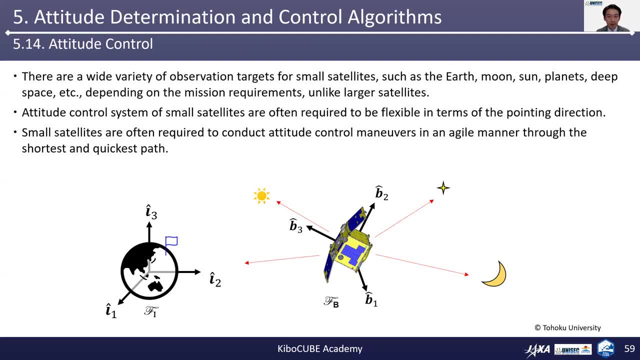 such as the Earth, Moon, Sun planets, deep space, etc. as indicated in the figure below, Depending on the mission requirements. unlike in larger satellites, the attitude control system of small satellites are often required to be flexible in terms of the pointing direction. 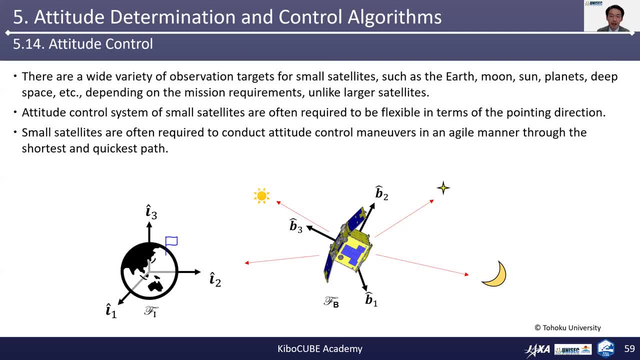 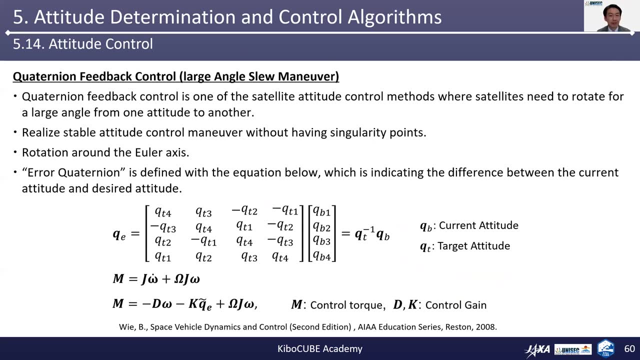 And also small satellites, are often required to conduct attitude control maneuvers in an agile manner through the shortest and or quickest path. Based on this background, in this presentation I introduce you to so-called quaternion feedback control, also known as large-angle slew maneuver. 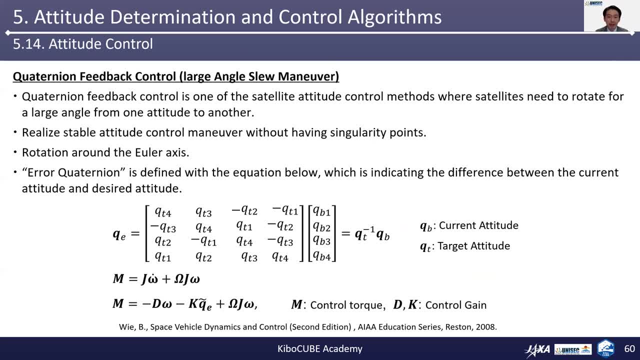 So quaternion feedback control is one of the satellite attitude control methods where satellites need to rotate for a large angle from one attitude to another. This method can realize stable attitude control maneuvers without having singularity points with the rotational rotation around the Euler axis. 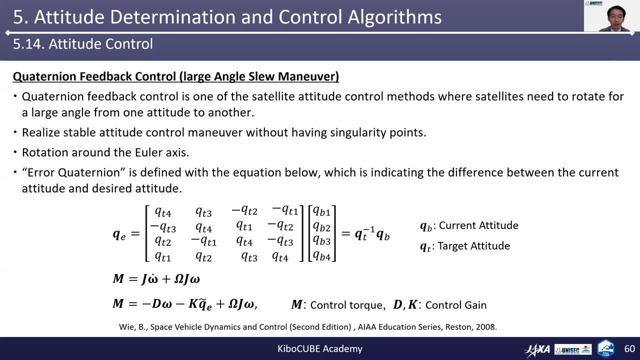 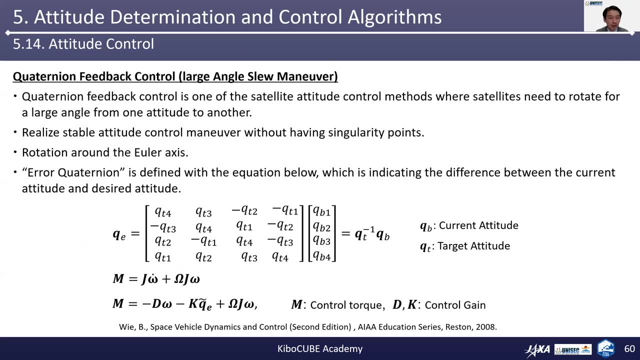 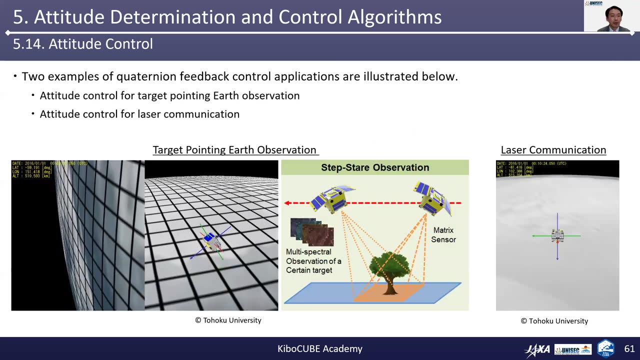 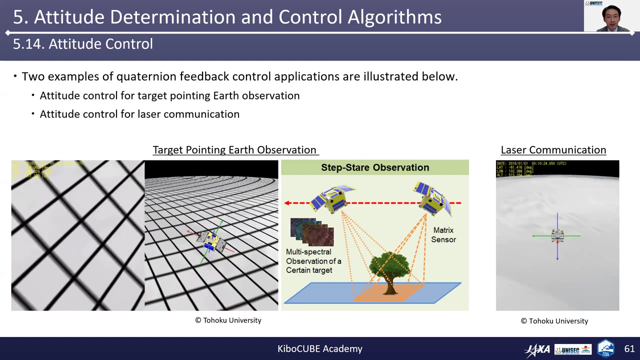 Error. quaternion is defined with the equation below, which is indicating the difference between the current attitude and desired attitude, described in quaternions and used for the feedback gain calculation. So two examples of quaternion feedback control applications are illustrated below The left one. 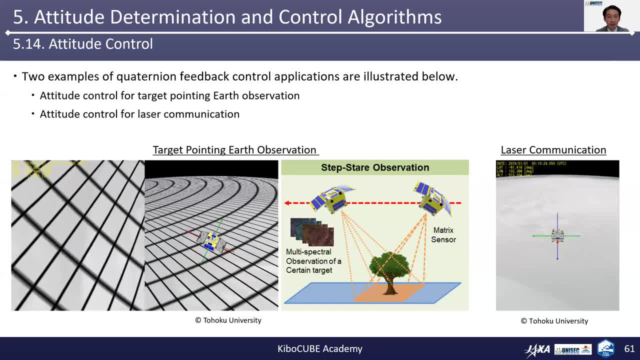 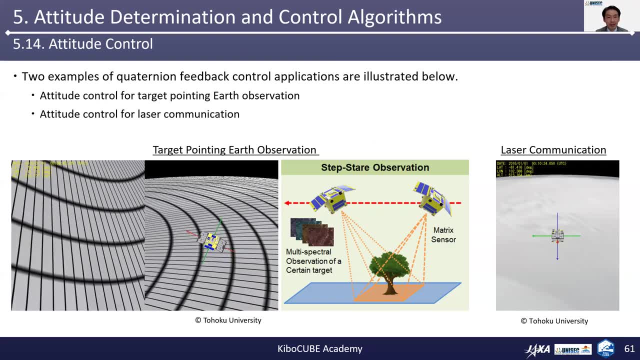 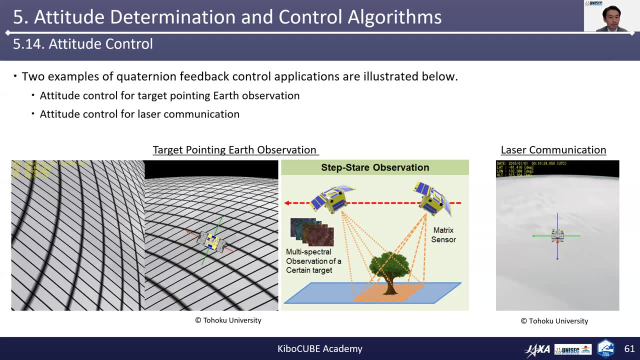 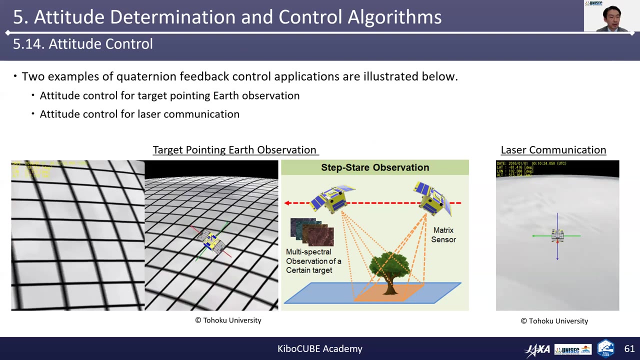 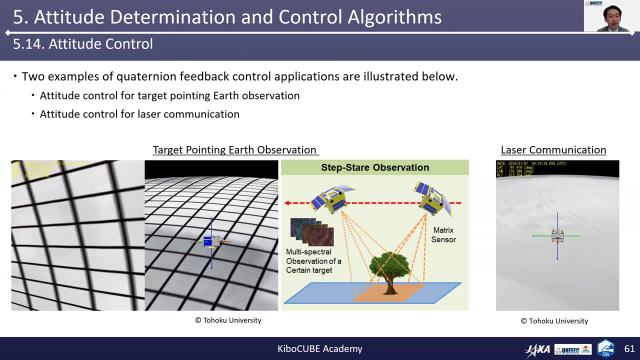 is the attitude control for target-pointing earth observations. Let's take a look at this animation first. You can see that the satellite is observing a target fixed on the earth's surface. It is observing the earth's surface in this way as an example. 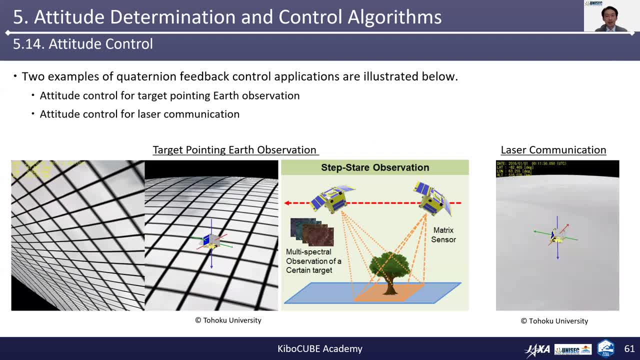 And the right side one is the attitude control for laser communication between the ground station. It is indicated with the red line, So let's take a look at this animation. So for the laser communication, rotational angle around the target direction can be arbitrary. 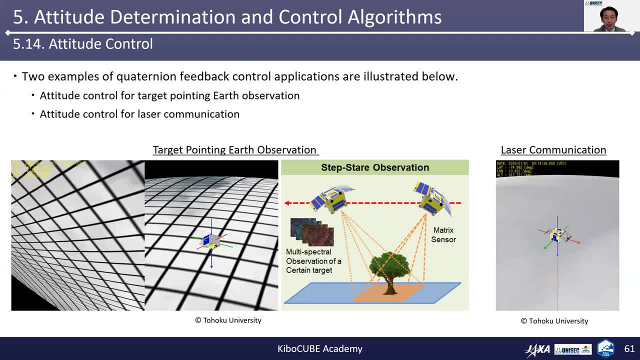 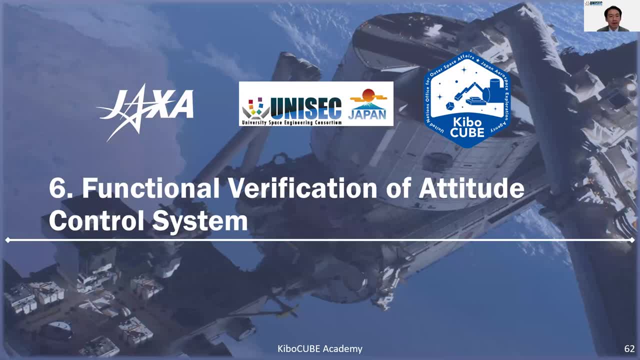 While that angle plays an important role, you can see that the satellite is observing a target fixed on the earth's surface. So the last topic of this lecture is about the functional verification of an attitude control system For the electrical testing of the satellite. 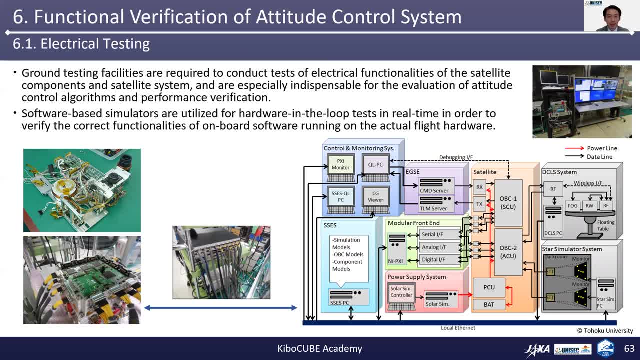 system. ground testing facilities are required to conduct the electrical function tests of the satellite components in an end-to-end test configuration. Software-based simulators are often utilized for hardware-in-the-loop tests in real-time in order to verify the correct functionalities of the on-board software. 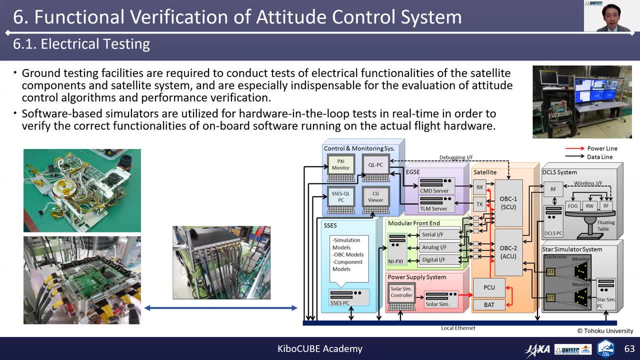 running on the actual flight hardware. These pictures are illustrating the electrical test facility and setup for high-performance satellites in orbit. The diagram in this slide is an example of the electrical testing of satellites in orbit. The diagram in this slide is an illustration of the 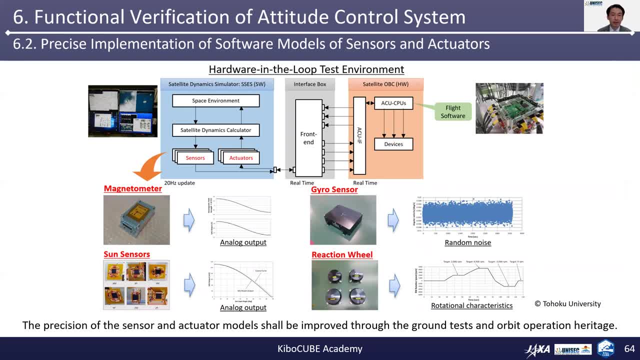 electrical testing of satellites in orbit. The satellite is illustrating the hardware and software components related with the hardware-in-the-loop testing configuration of the simulator, The satellite and dynamics simulator for this kind of ground testing facility, which is located in the center of the satellite. 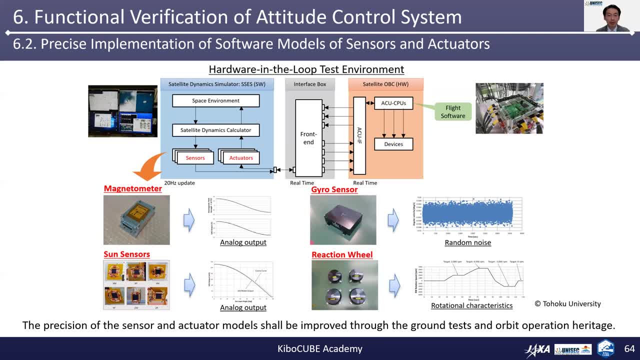 The diagram in this slide is an illustration of the actual control software. The figures below are illustrating the onboard components of the satellite. In this slide you can see that the satellite is located in the center of the satellite. The satellite is located in the. 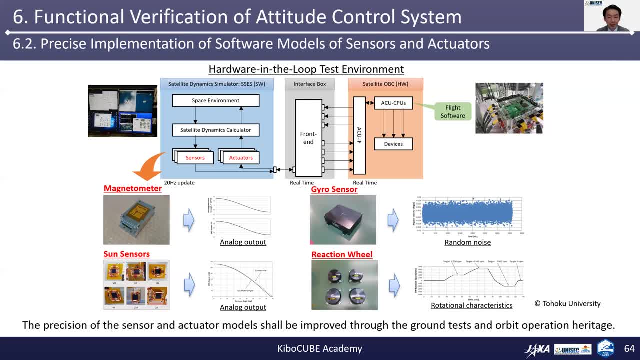 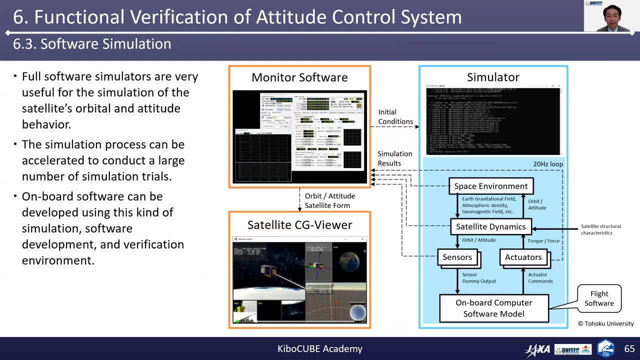 center of the satellite. The satellite is located at the center of the satellite. Look at the graph here. As you see, the satellite has been placed vertically and in the center of the satellite. The can be accelerated to conduct a large number of simulation trials. Onboard software can be. 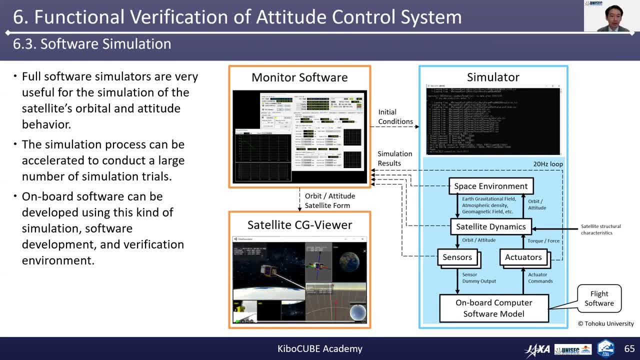 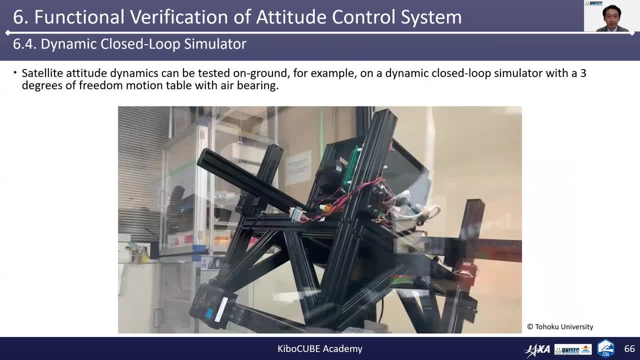 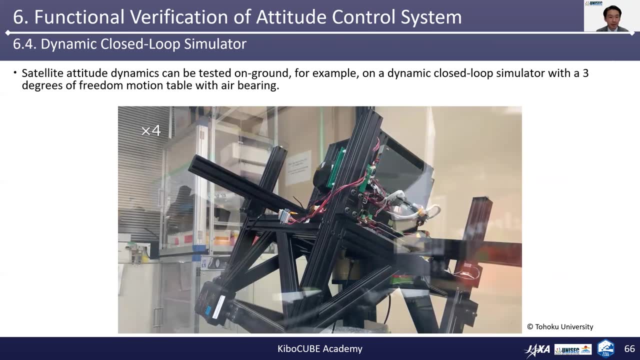 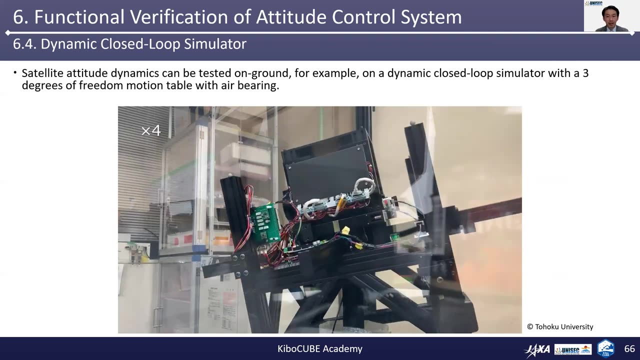 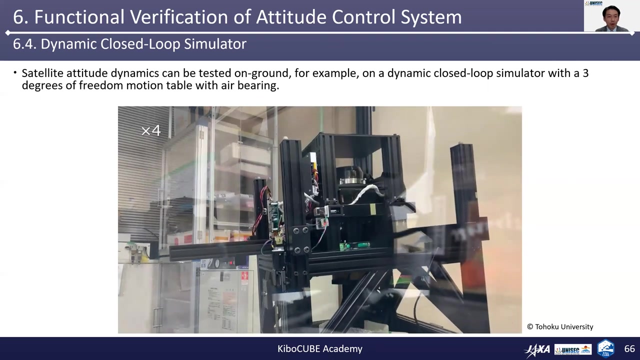 developed using this kind of simulation and software development and verification environment very effectively. The actual satellite dynamics cannot be evaluated by software-based simulators. For this purpose, dynamic simulators are often used to evaluate a microgravity environment. They are often two-dimensional on a floating table or it can be three-dimensional. 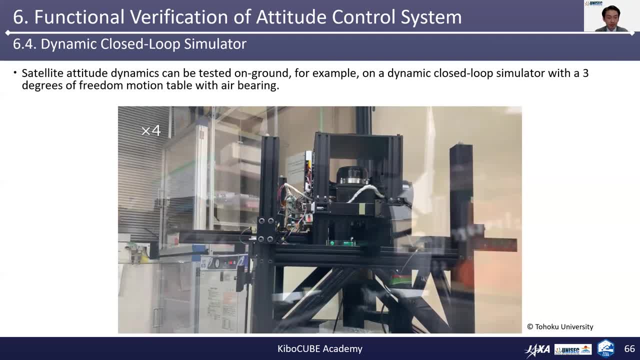 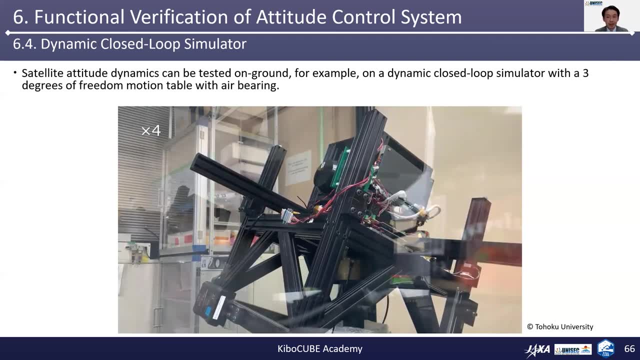 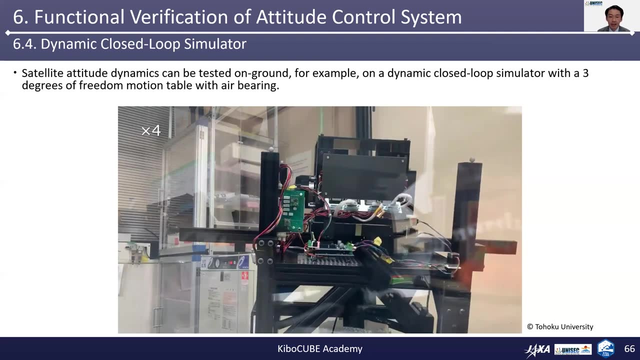 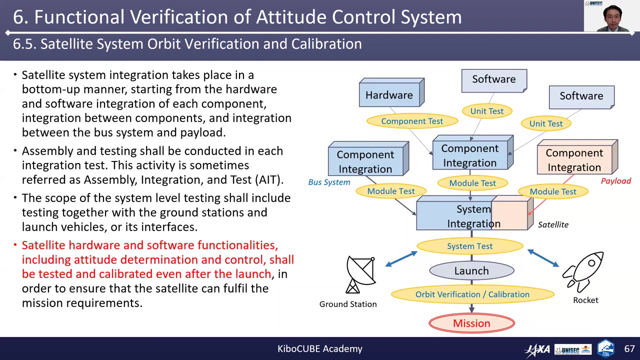 on a floating air bearing, as shown in this video. This testbed is equipped with reaction wheels as actuators and gyroscopic sensors for angular velocity measurements. In this way, satellite attitude dynamics can be tested on ground with three degrees of freedom. Satellite system integration takes place in a bottom-up manner, starting from the hardware and 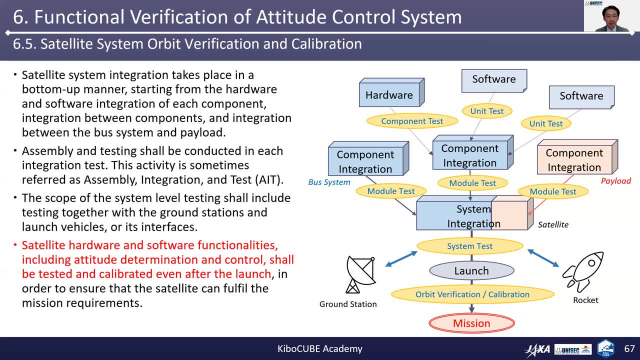 software integration of each component, integration between components and integration between the bus system and the ground and payload. Assembly and testing shall be conducted in each integration step. This activity is sometimes called assembly, integration and test or AIT, The scope of the system-level testing. 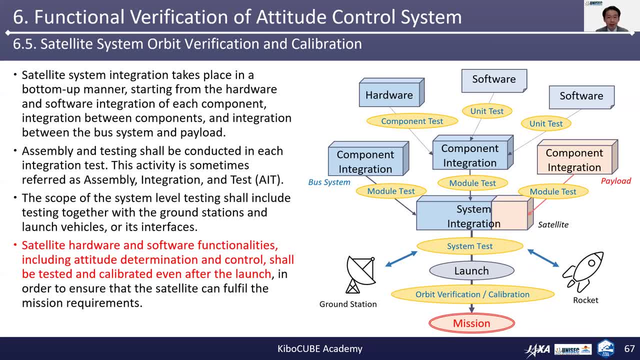 shall include testing together with the ground stations, launch vehicles and any other interfacing systems. Also, it is important to note that the satellite hardware and software functionalities shall be tested and calibrated even after the launch in order to ensure that the satellite can fulfill the mission. 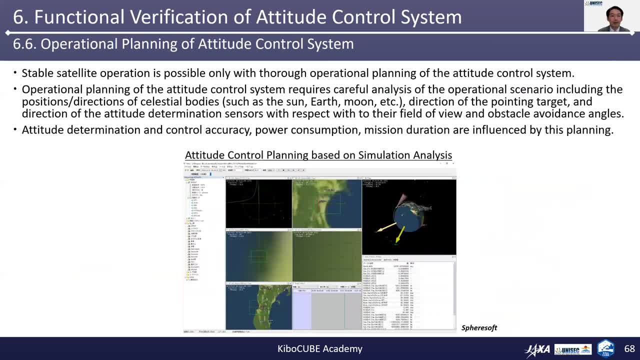 requirements. Stable satellite operation is possible only with thorough operational planning of the actual control system. Operational planning of the actual control system requires careful analysis of the operational scenario, including the positions, directions of celestial bodies such as sun, earth, moon, et cetera. 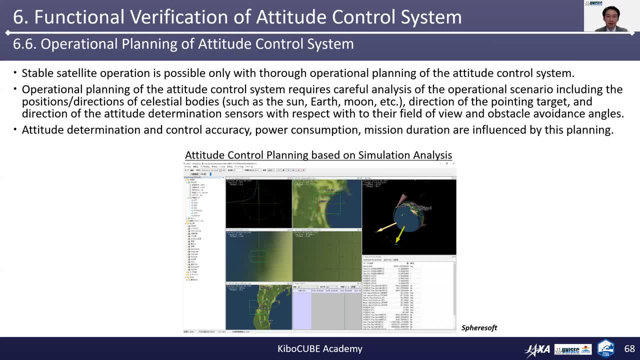 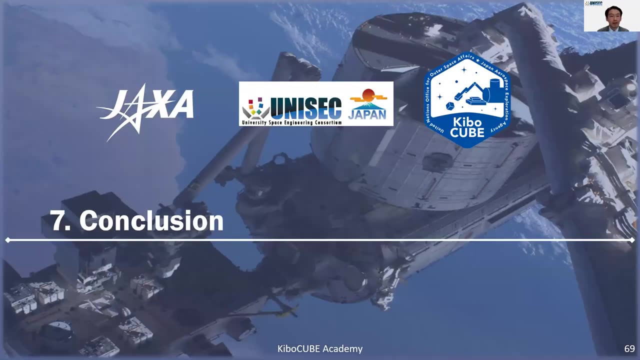 direction of the pointing targets and direction of the actual determination sensors with respect to their field of views and obstacle avoidance angles. Actual determination and control accuracy, power consumption and mission duration are influenced by this planning. Finally, I'd like to conclude this lecture with a summary. 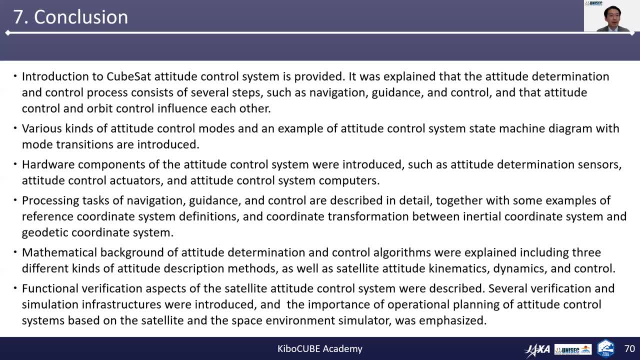 of the content we have covered, So an introduction to CubeSat's actual control system is provided. It was explained that the actual determination and control process consists of several steps, such as navigation, guidance and control, and that actual control and orbit control. 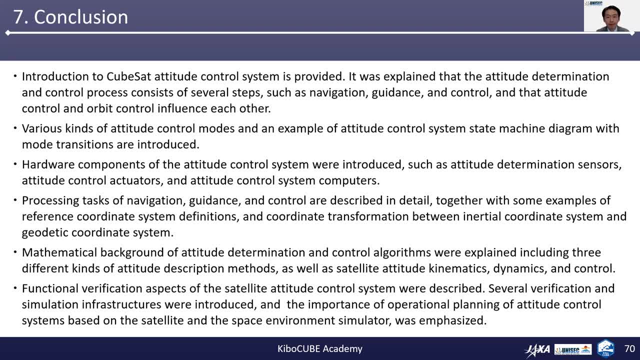 influence each other. Various kinds of actual control modes and an example of actual control system state machine diagrams. with mode transitions are introduced Harder components of the actual control system, such as the actual determination sensors, actual control actuators and actual control system computers. 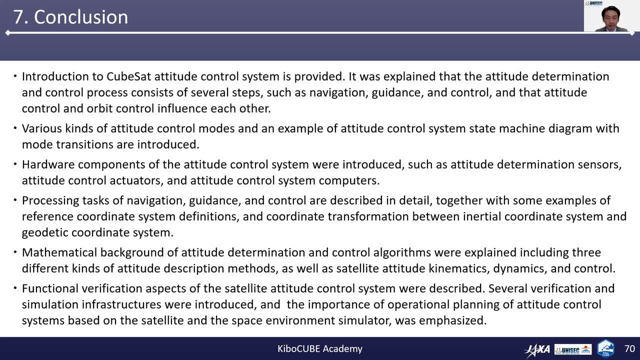 Processing tasks of navigation, guidance and control are described in detail, together with some examples of reference coordinate system definitions and coordinate transformation between inertial coordinate system and geodetic coordinate system. Mathematical background of actual determination and control algorithms were explained, including three different kinds of actual description methods.